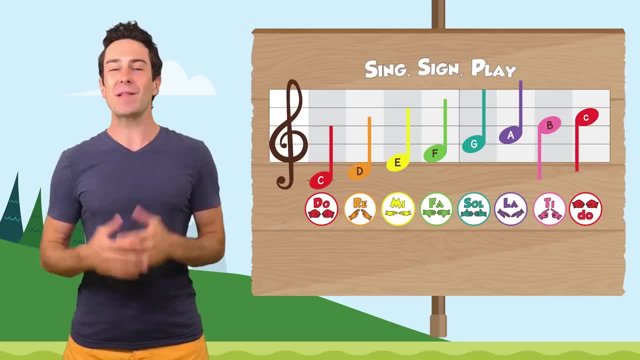 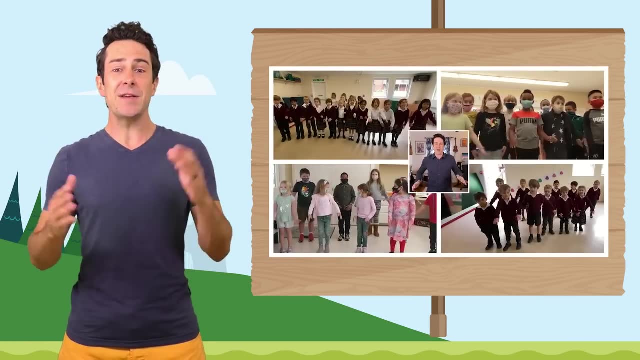 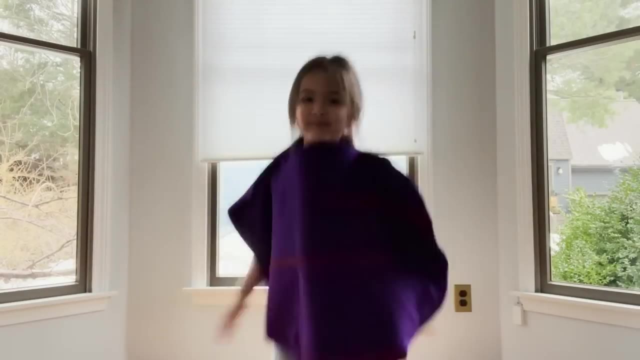 do re mi fa sol, and we'll learn all kinds of things about the awesome world of music. We'll start out with one of my favorite songs, Sweet Beats. Can you tap on your legs just like this? and then we'll sing along together for Sweet Beats. You ready? One, two. 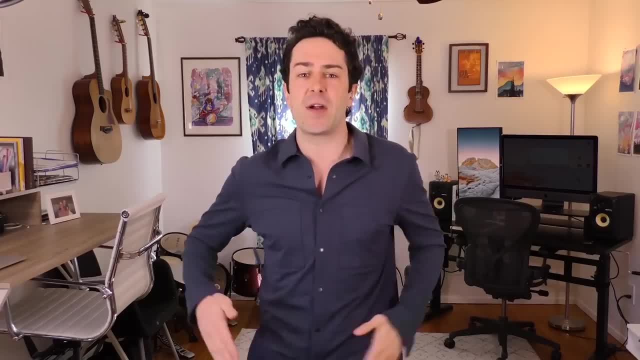 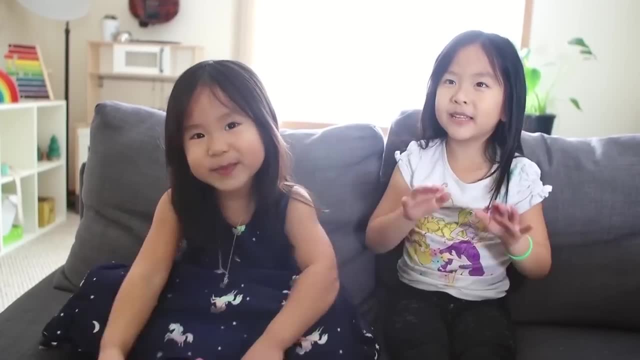 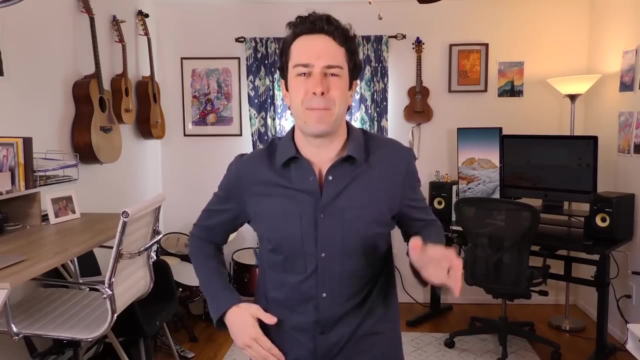 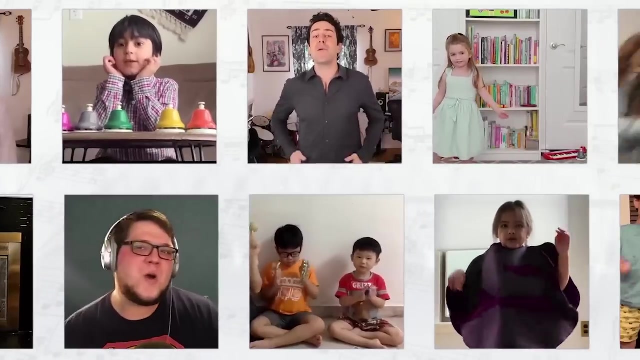 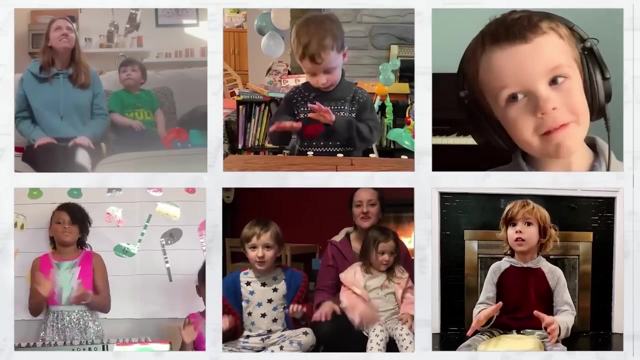 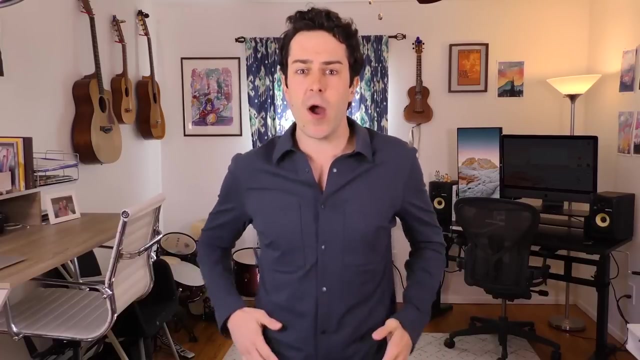 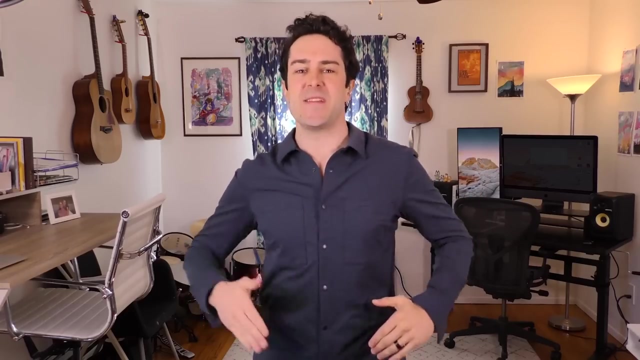 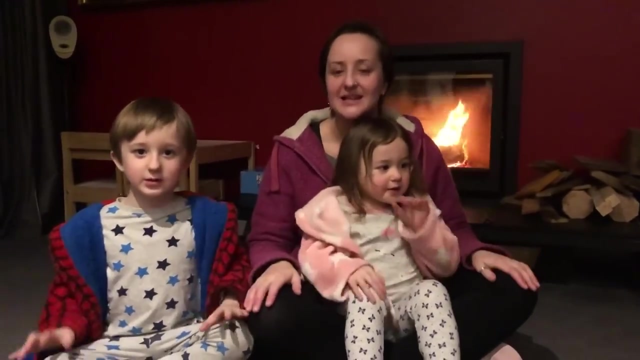 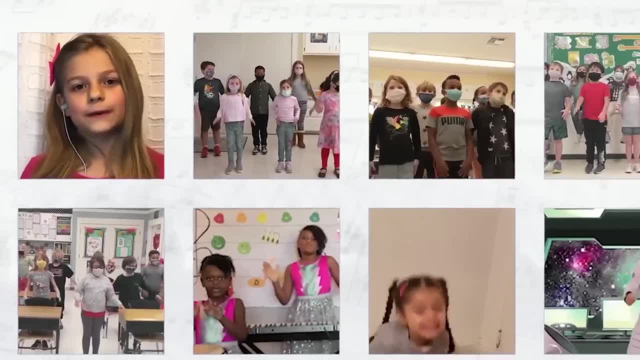 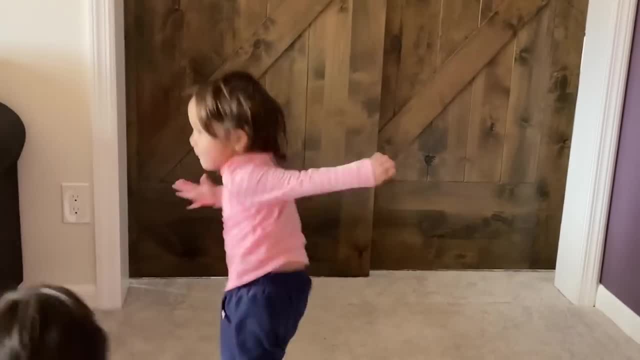 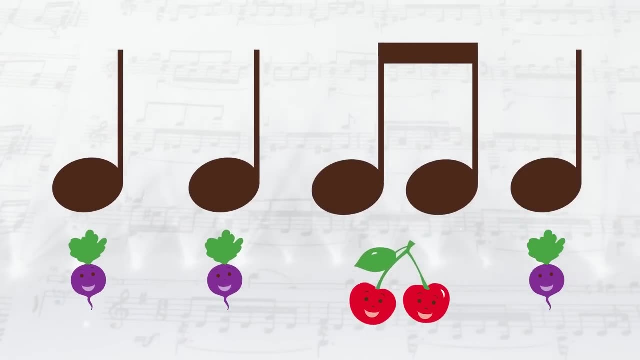 And if you want some sweet beets, we've got them. If you want some sweet beets, we've got them. If you want some sweet beets, we've got them. Let's do it loud this time: Beets, beets, cherry beets. 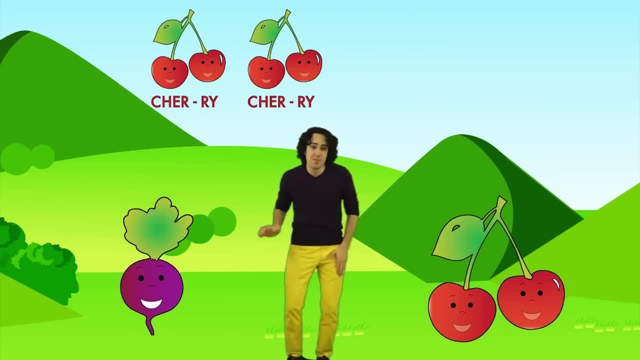 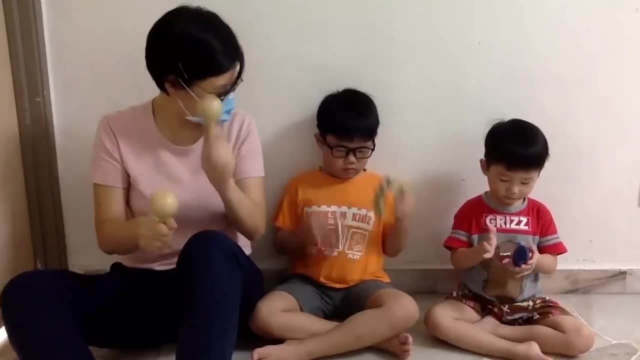 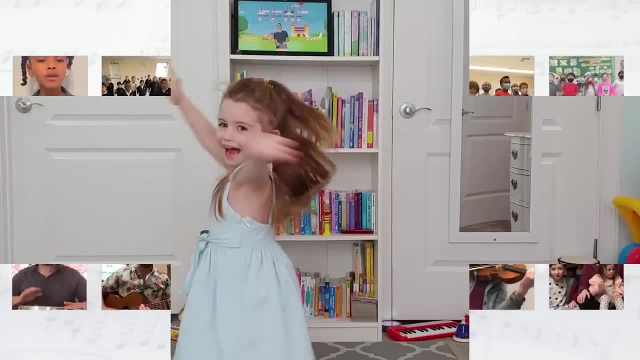 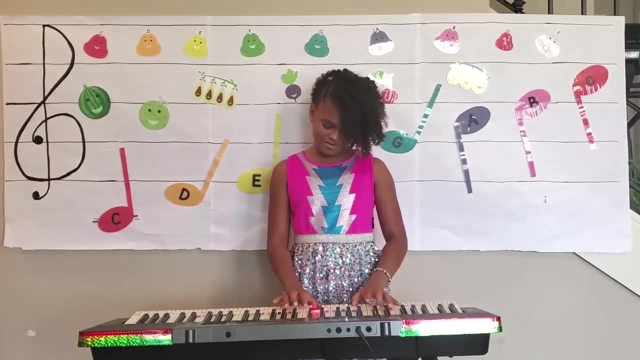 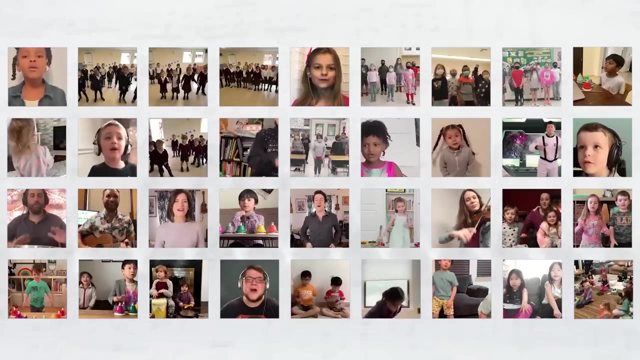 Beets, cherry, cherry beets, Beets, cherry, cherry beets, Sweet beets- we've got them. If you want some sweet beets, we've got them. If you want some sweet beets, we've got them. If you want some sweet beets, we've got them. 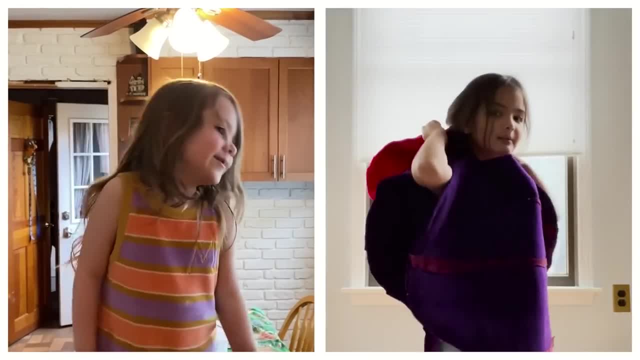 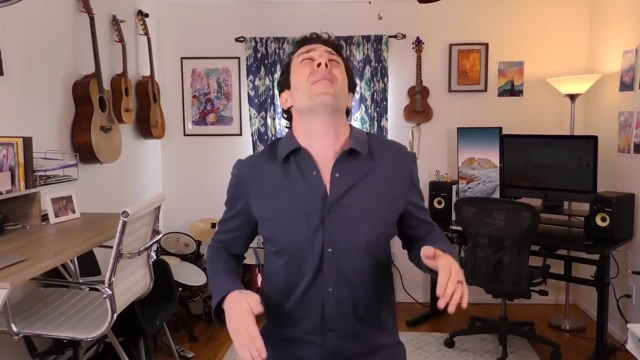 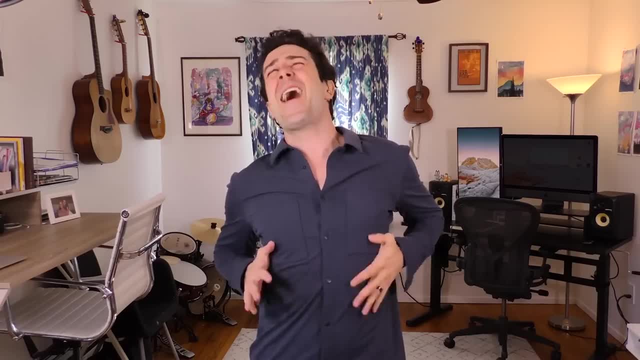 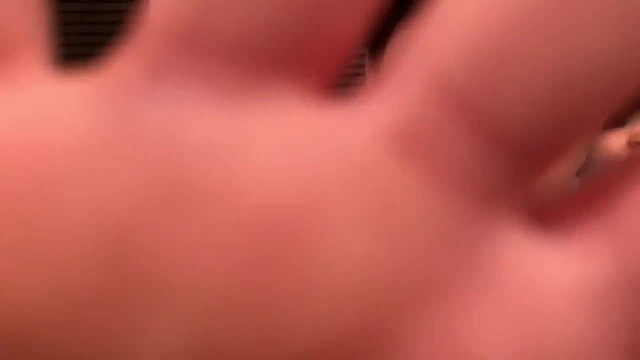 If you want some sweet beets, we've got them. If you want some sweet beets, we've got them. Give yourself a huge round of applause. Excellent job singing Sweet Beets with Beats and Cherry everybody. Nice work with Sweet Beets. 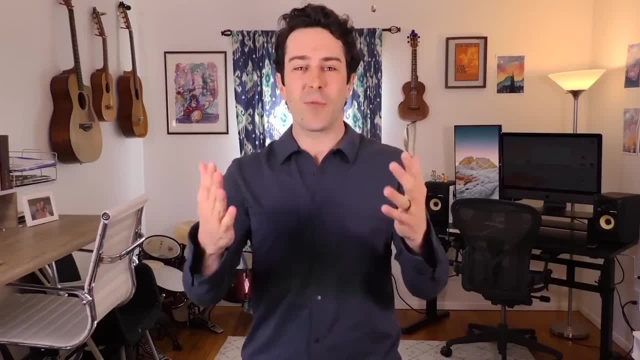 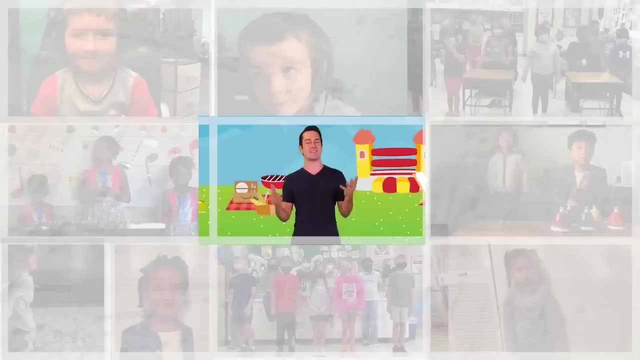 Nice work with Sweet Beets. Nice work with Sweet Beets. Thank you so much for being a part of our first ever virtual choir. Thank you so much for being a part of our first ever virtual choir. Happy Musicking And until next time. 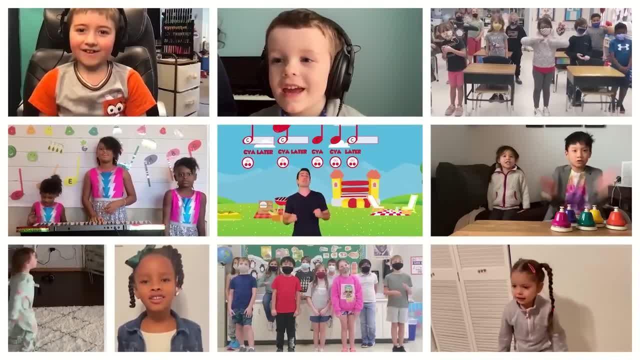 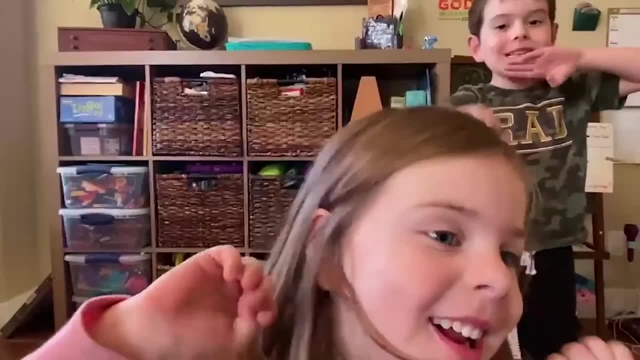 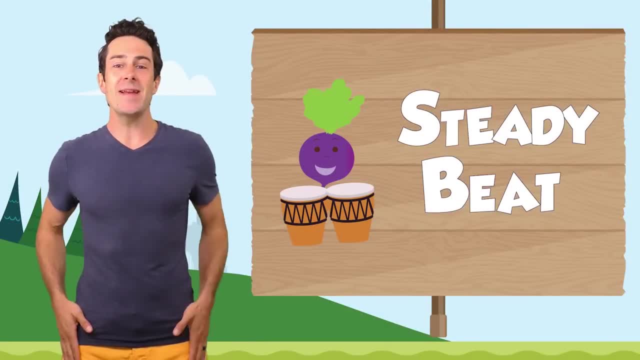 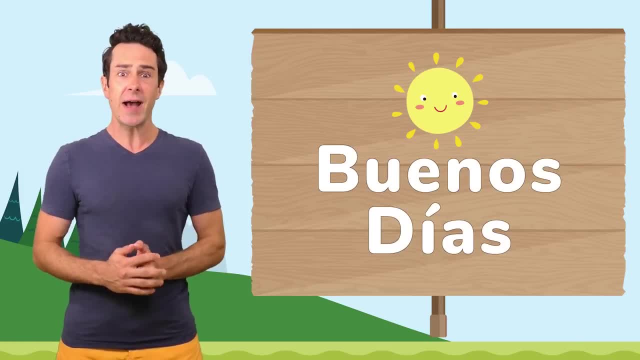 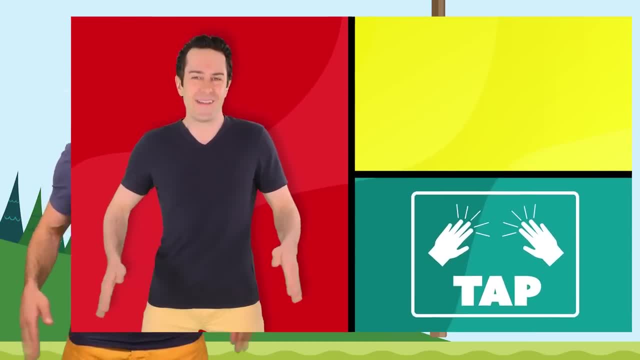 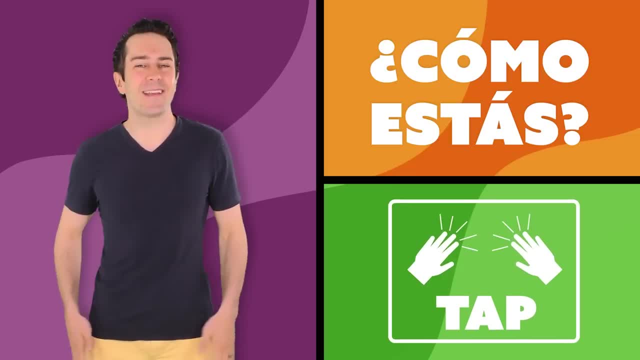 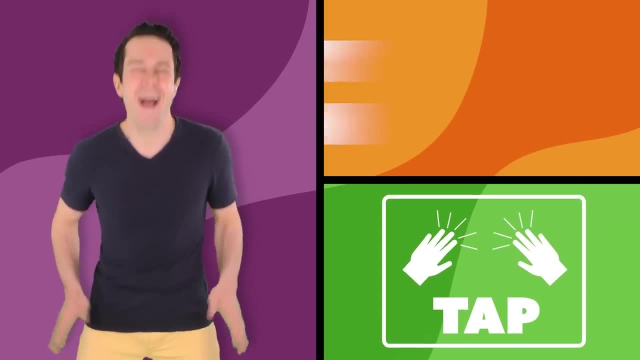 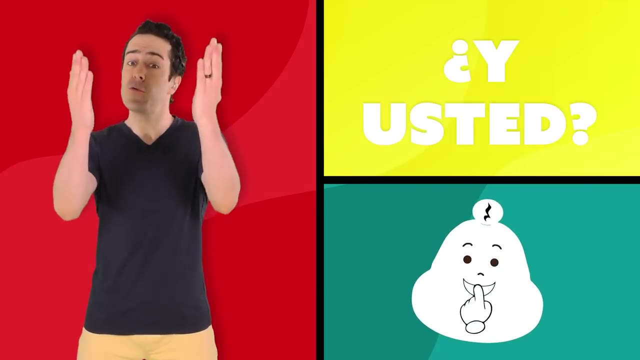 And until next time I will see you later. And until next time I will see you later. And until next time I will see you later. Buenos dias, Como estas Muy bien, Gracias Y usted Nice. 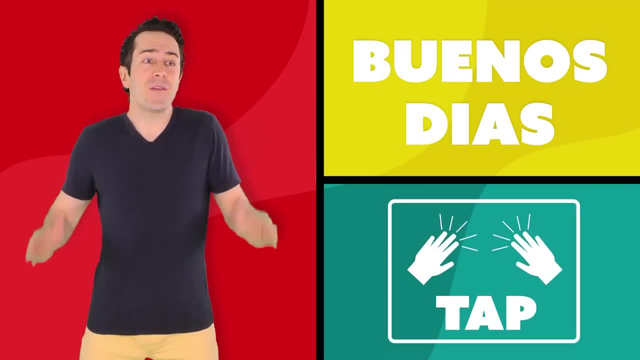 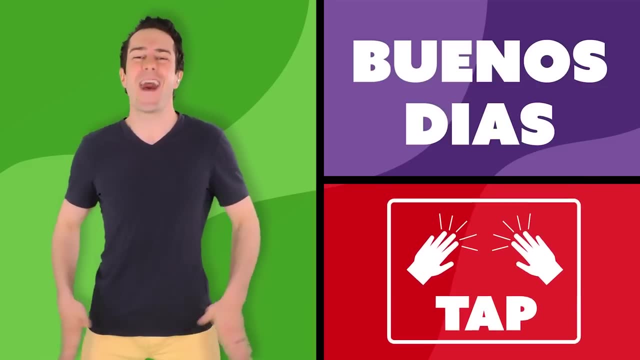 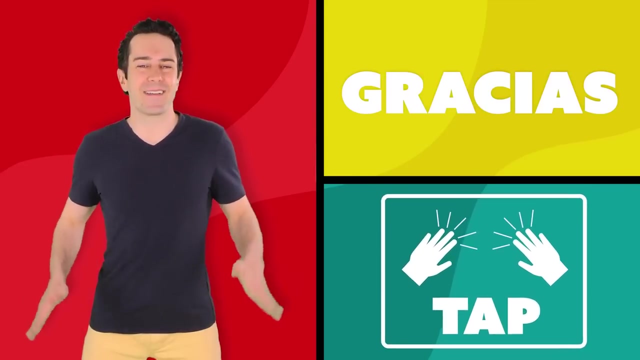 Let's try that again, just like that. Buenos dias, Keep on tapping, Como estas A nice, steady beat. Buenos dias, Como estas Muy bien, Gracias, Gracias Y usted. Can you pretend to strum a guitar? 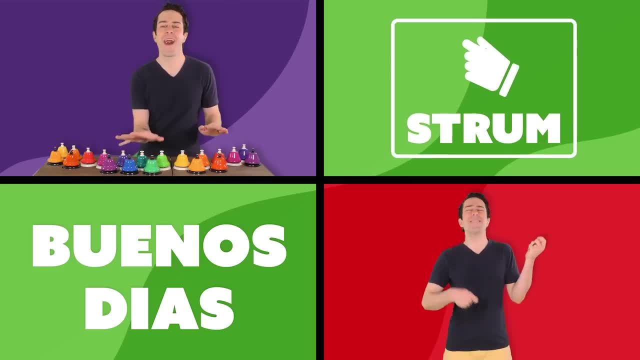 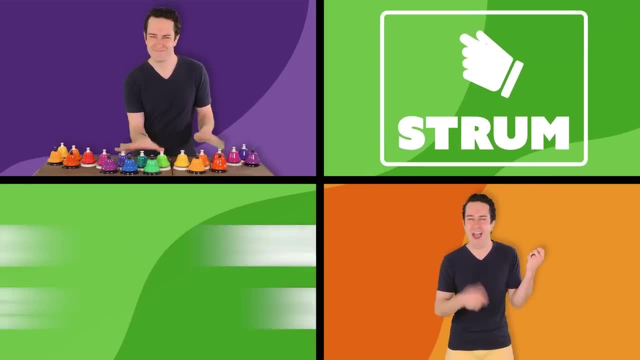 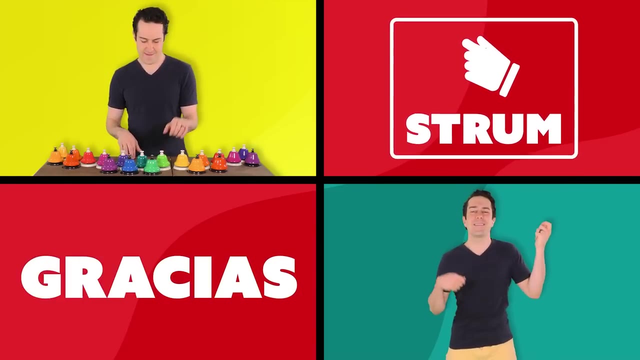 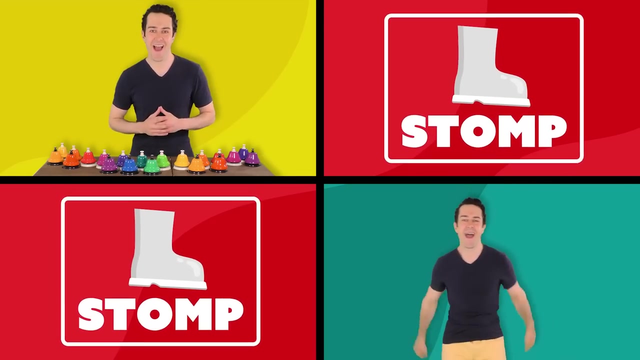 One, two, three. Buenos dias Como estas. Buenos dias, Buenos dias Como estas, Como estas. Muy bien, Gracias Y usted. Y usted Just stomp those feet. Buenos dias, Buenos dias Como estas. 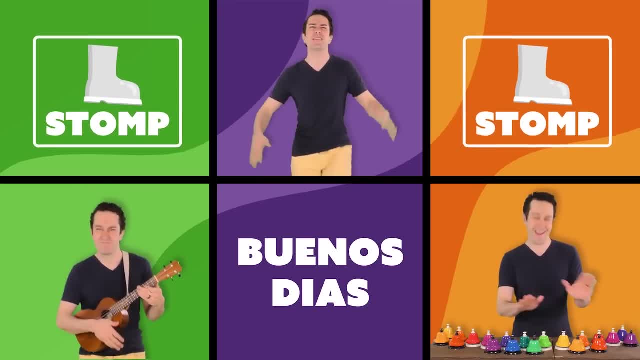 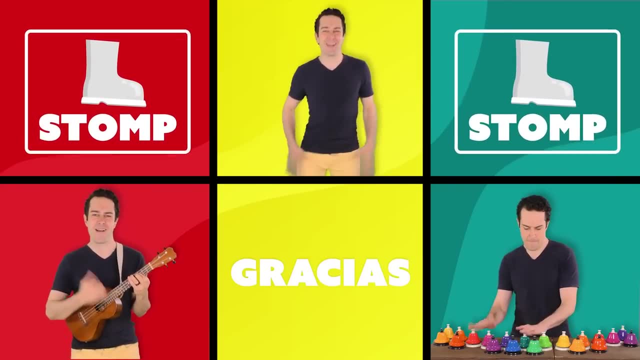 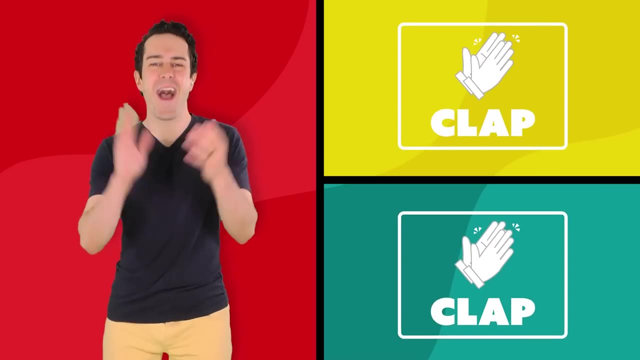 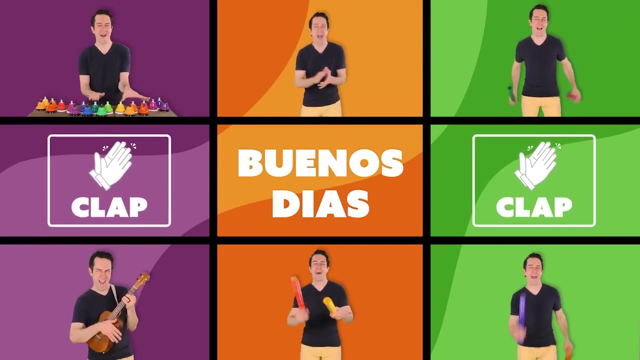 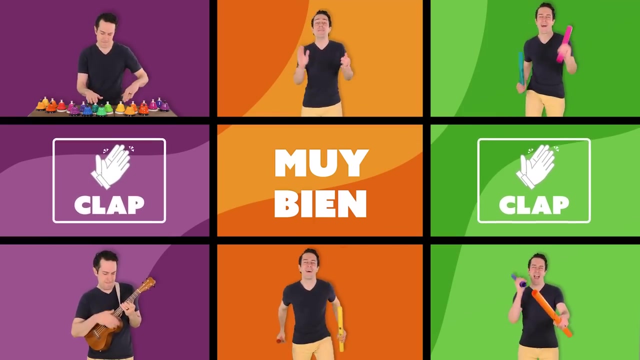 Keep on stopping. Buenos dias, Nice and steady, Como estas Muy bien. Gracias Y usted. Y usted, Alright, clap those hands. Buenos dias, Buenos dias Como estas. Buenos dias, Buenos dias Como estas Muy bien. 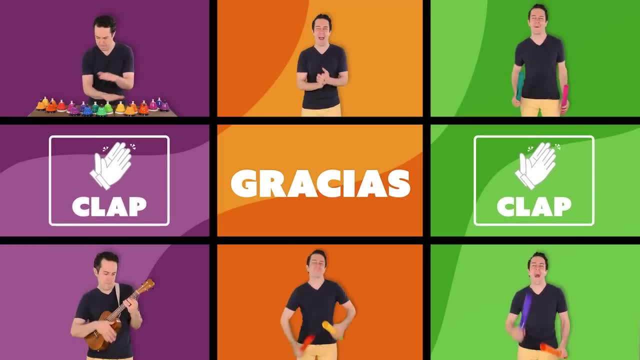 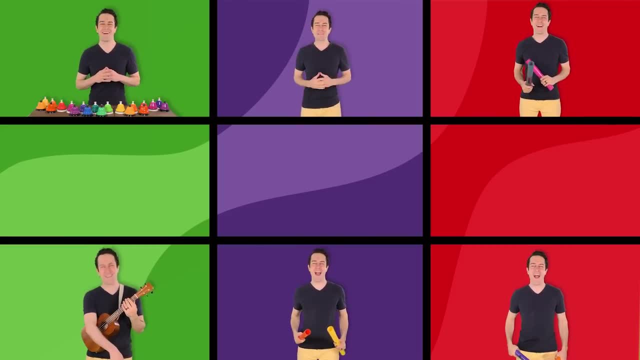 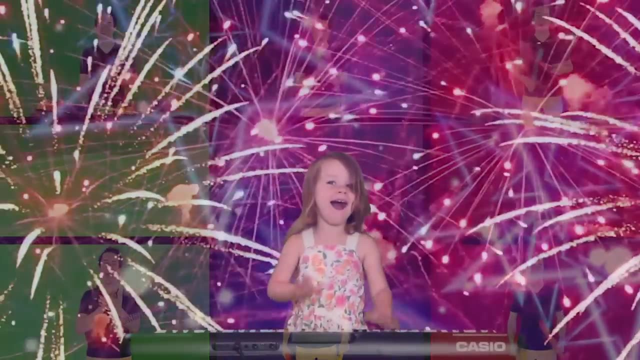 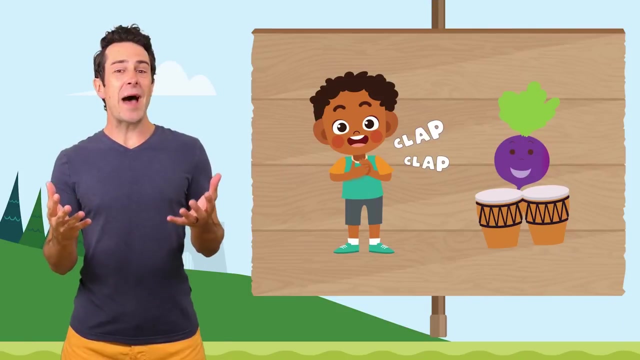 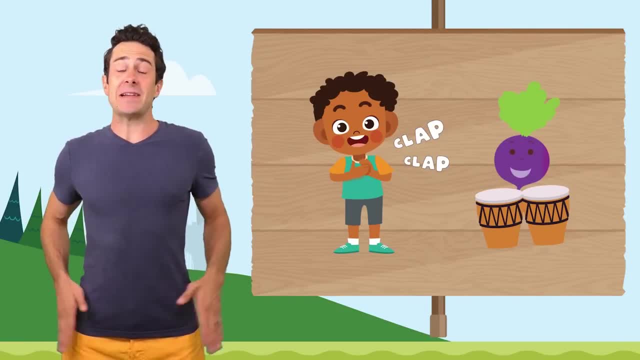 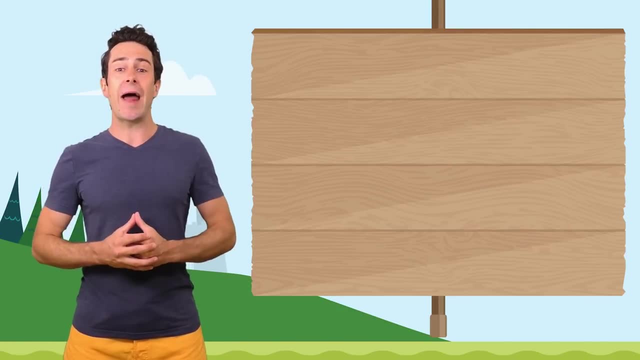 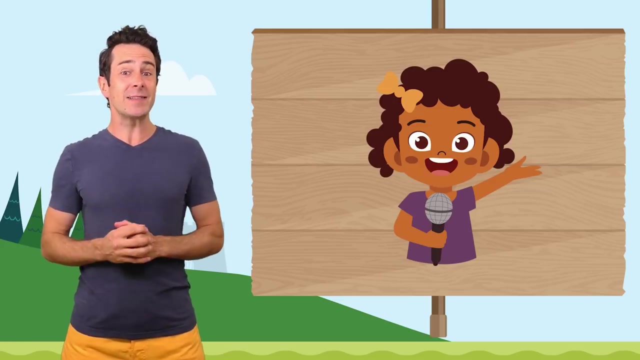 and keeping a steady beat, Having a great sense for rhythm and playing a steady beat is really important, but it's also really important that we focus on our vocals, on our voices, on our musical pipes, and that we work on singing different musical notes. Some of them can be: 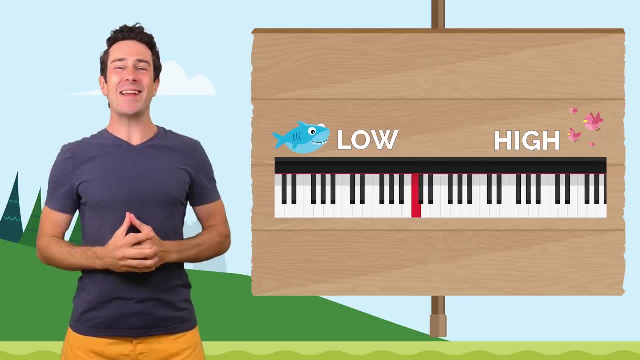 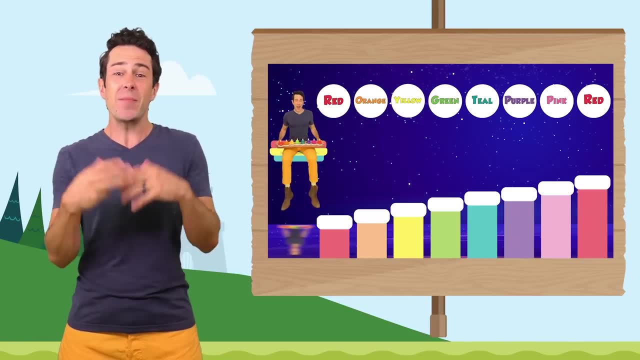 low and some of them can be high, And today we're going to see eight different notes. We're going to sing about the colors, the numbers, the letters, the solfege. It's going to be a ton of fun. Are you ready to sing with me? 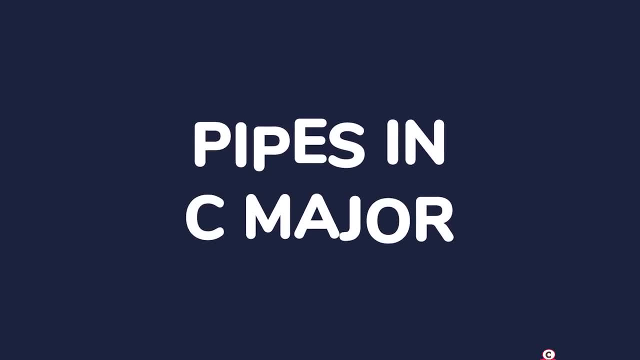 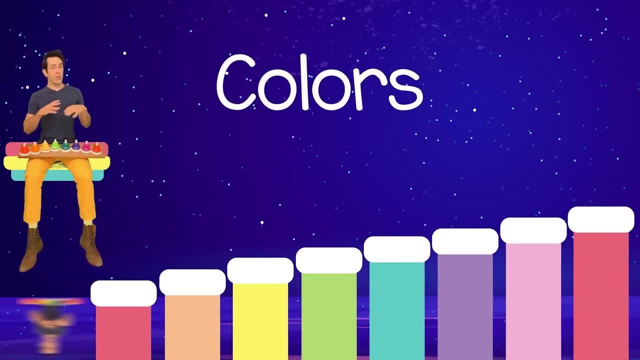 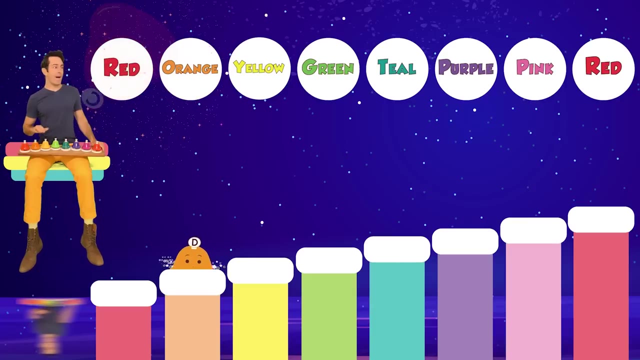 Let's hop into the pipes in C major. Alright, we're going to start out by singing about the colors on red with some really long whole notes. One, two let's sing red, Red, Up to orange, Up to yellow, Then green. 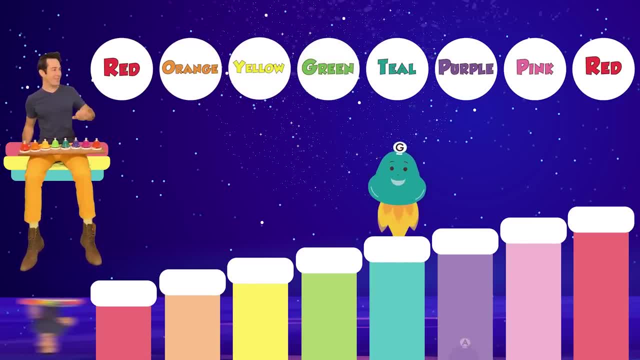 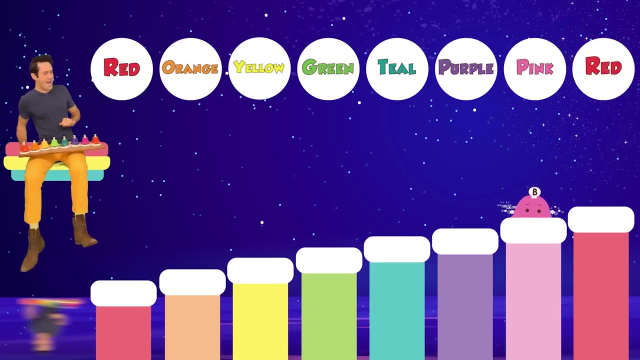 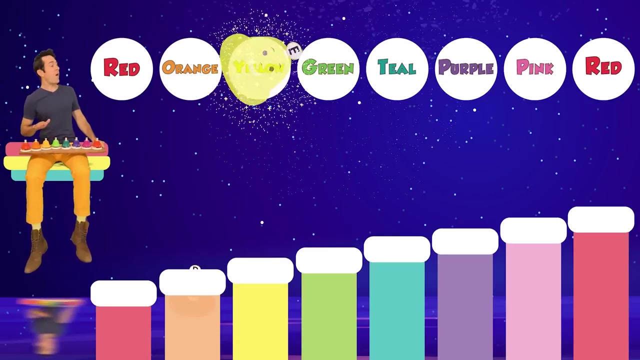 Up to teal, Purple, Pink And red. Let's do it backwards: Red Pink, Red Pink, Red Pink, Purple, Purple, Teal, Down to green, Yellow, Yellow, Orange, Orange And red. 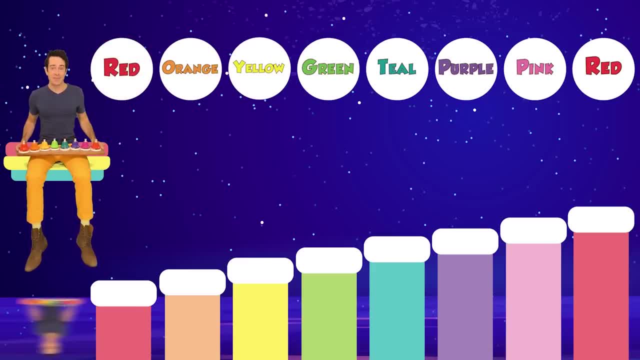 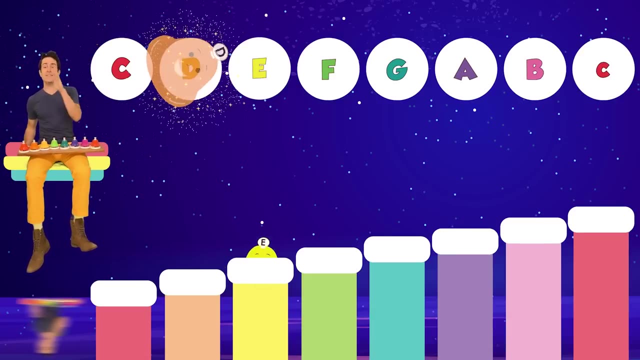 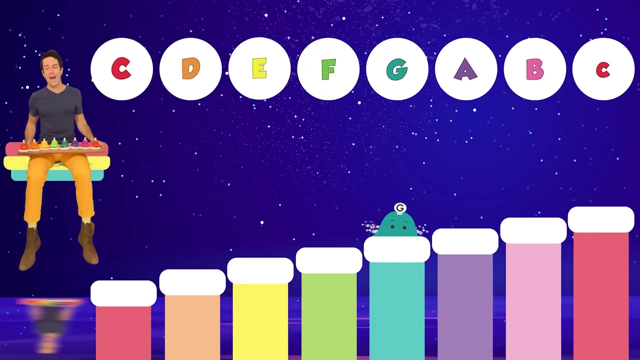 Orange And red. Nice job singing about the colors. Next we're going to do the note names C, D, E. still really slow with some long whole notes C, D, E And F Up to G, A, B. 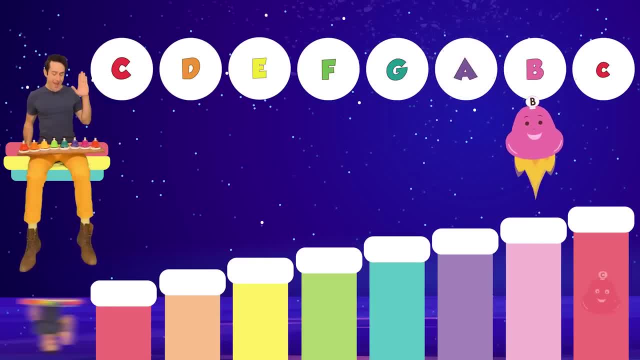 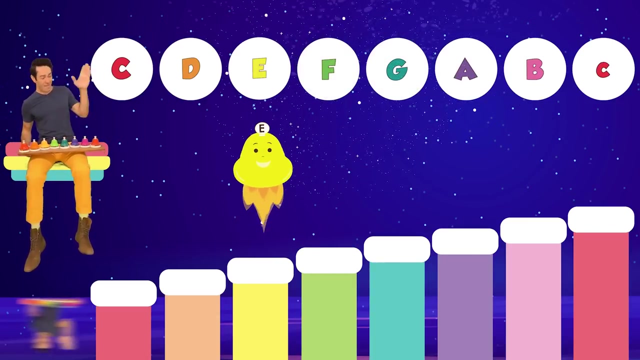 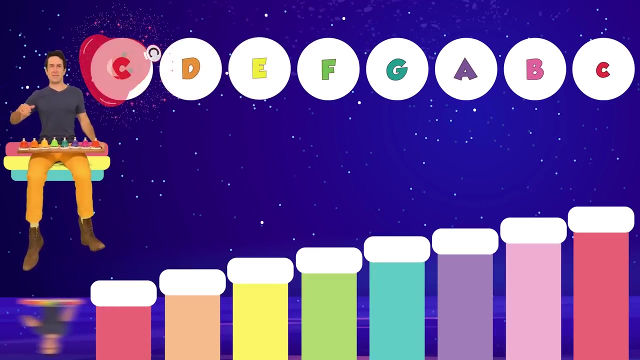 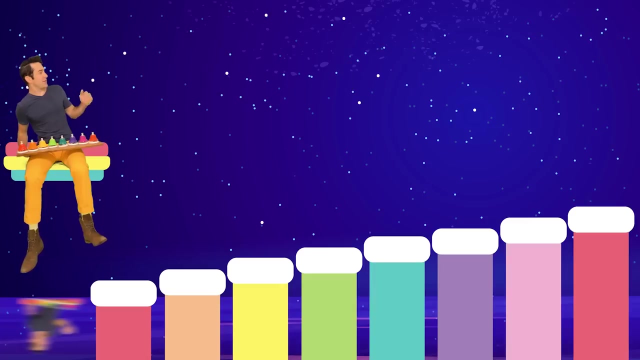 And high C. Back down C, B, C, D, E, A, G, E, F, E, D, D. Down to C, Down to C. Nice job with the note names. Okay, next up we're going to do the solfege. 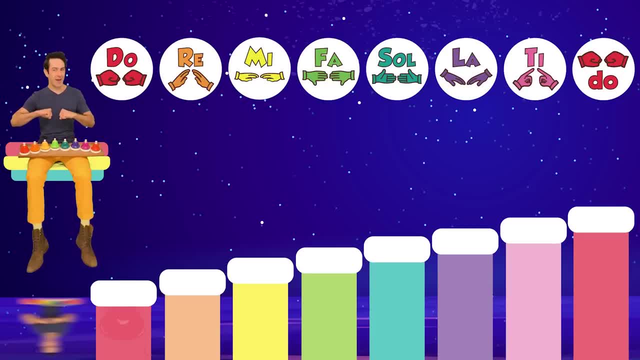 hand signs. You can play your bells or do the hand signs with dough Do, Re, Mi, E And fa. Flip that up For sol To la Piercing tone. Ti And high Do Now backwards. 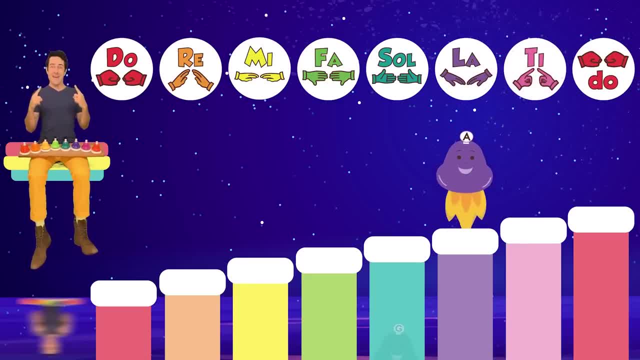 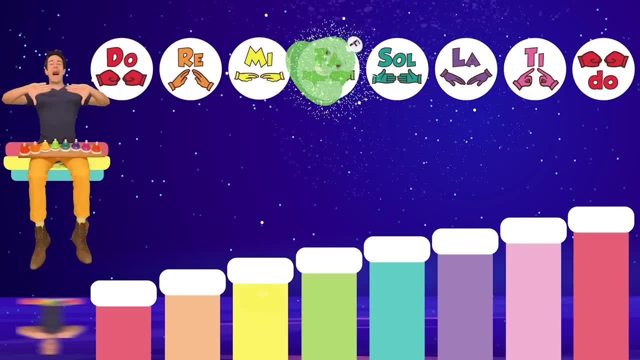 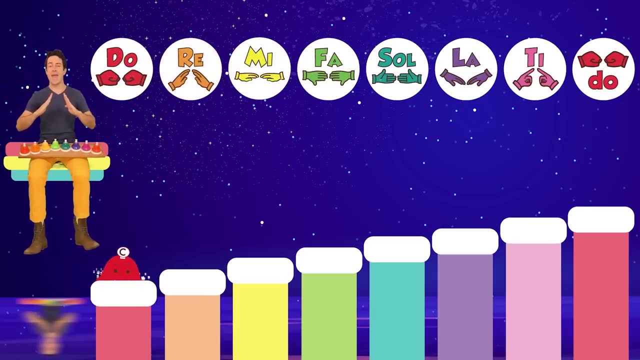 Do Ti La Sol Fa, Mi, Fa, Mi, Re, Do, Re, Do. Nice job with the solfege hand signs everyone. We're going to do the solfege hand signs again, but with faster notes, With half notes. 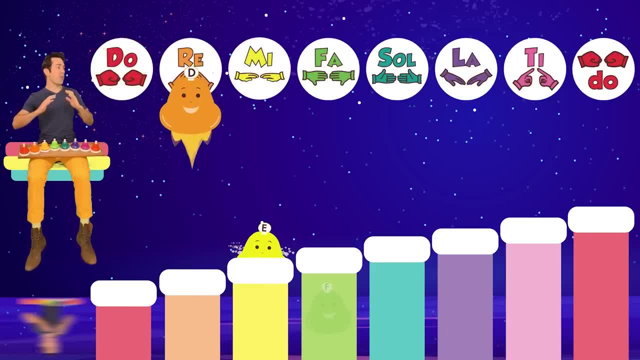 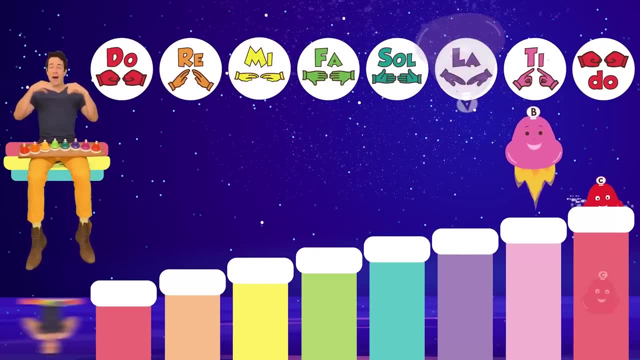 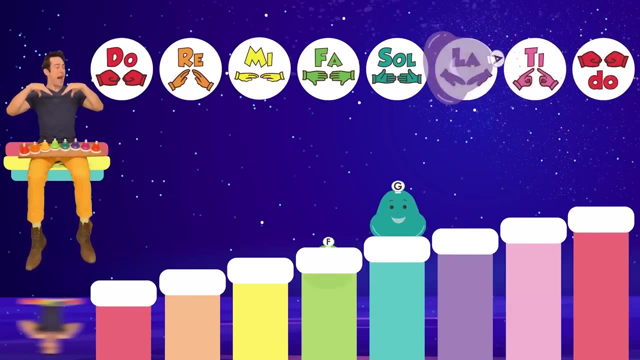 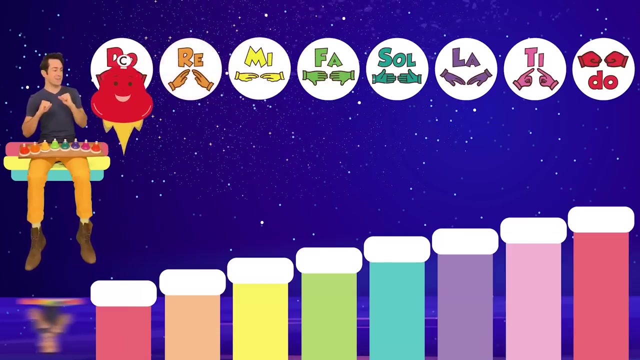 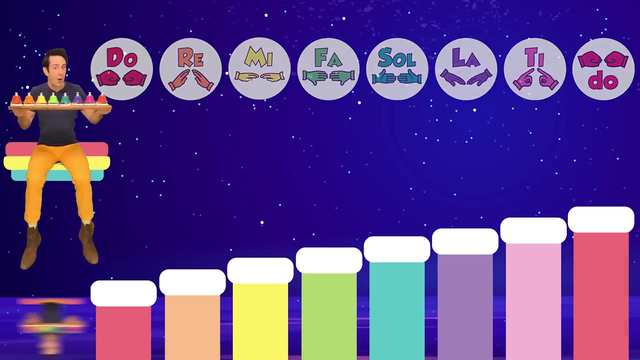 twice as fast Ready. Do Re Mi Fa Sol La Ti Do. Do Ti La Sol Fa Mi Re Do. Nice job, everybody with the solfege hand signs We're going to play. 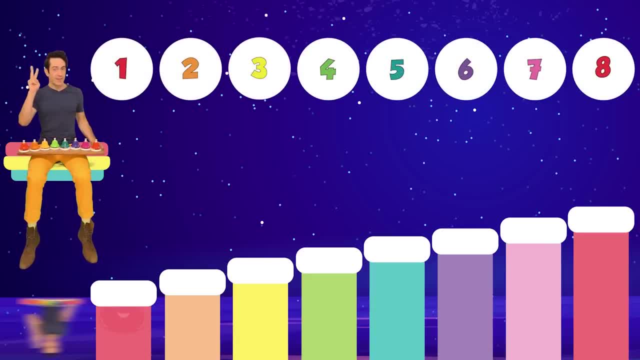 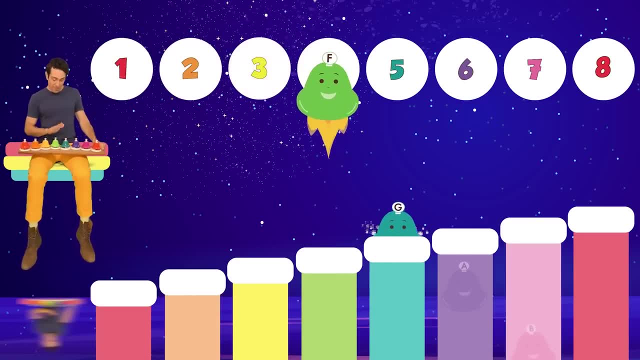 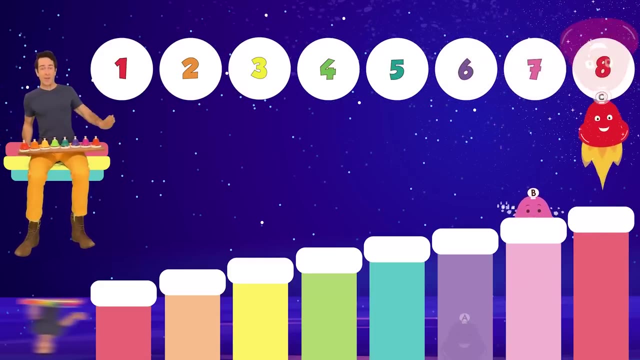 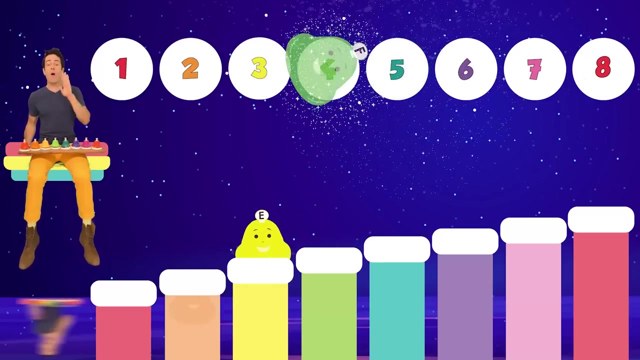 bells Sing about the numbers One, Two, Three. Here we go. One, Two, Three, Four, Five, Six, Seven, Eight Backwards: Eight Seven Six, Five, Four, Three, Two, One. 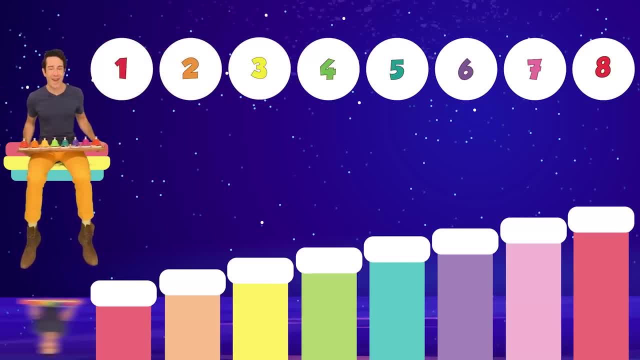 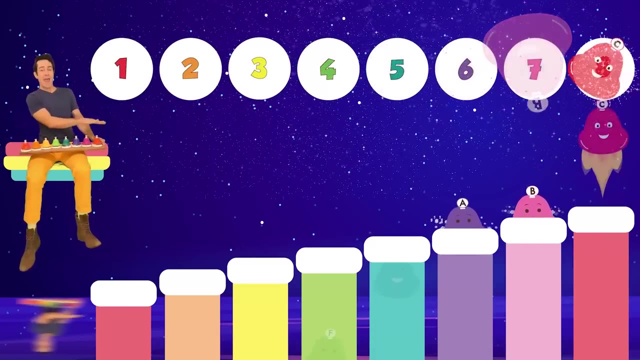 Nice job with that. Do you think we can do it even faster? You ready Even faster? One Two, Here we go. One Two, Three, Four, Five, Six, Seven, Eight, Eight, Seven, Six. 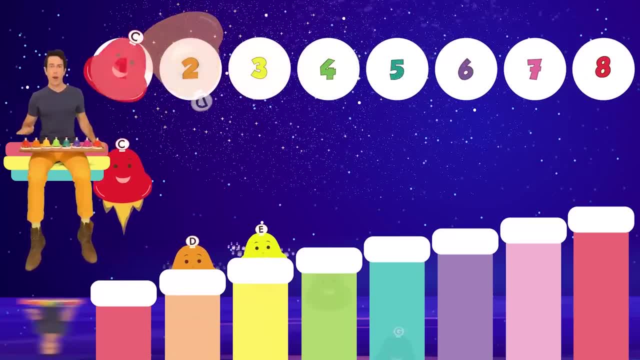 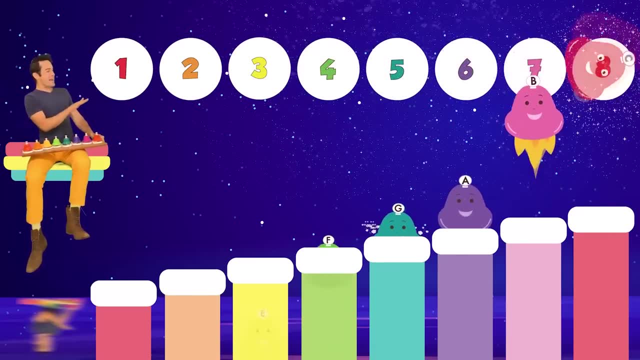 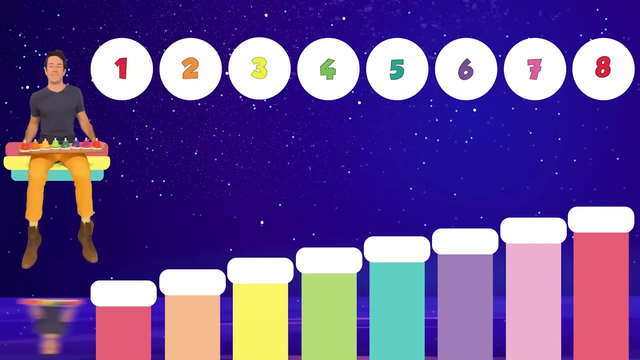 Five, Four, Three, Two, One. Again One, Two, Three, Four, Five, Six, Seven, Eight Eight Seven, Six, Five, Four, Three, Two, One One. Give yourself a huge round of. 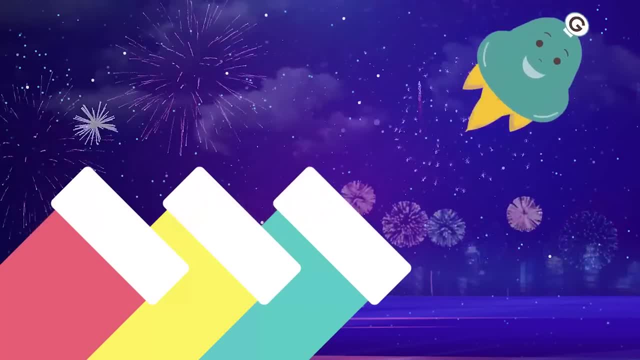 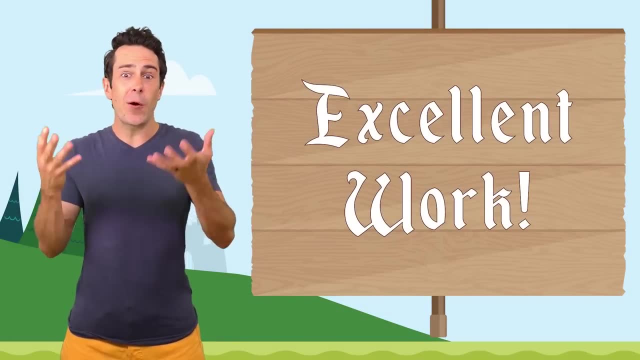 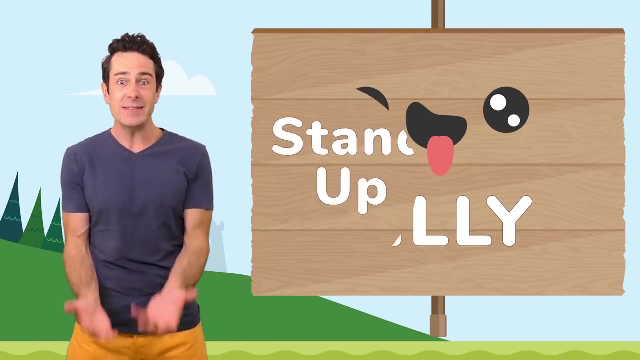 applause. Excellent work with the pipes in C major. Excellent work using your pipes in C major. Now we're going to get pretty silly and move our bodies and do some dancing. So stand up and repeat after me. Can you say hands up? 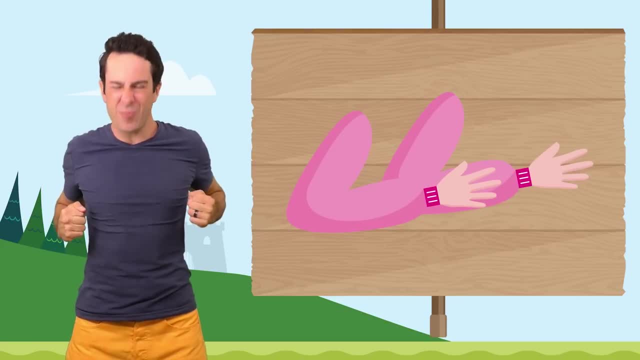 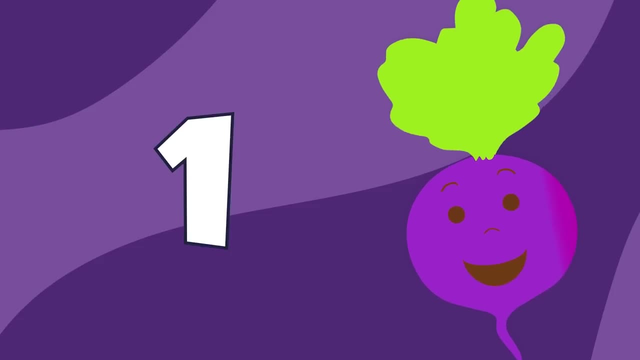 Hands up, Elbows back, Elbows back, And we're going to do lots of silly dance moves like that here in the Tutti-Tah. One, Two, One, Two Ready, Tutti-Tah, Tutti-Tah. 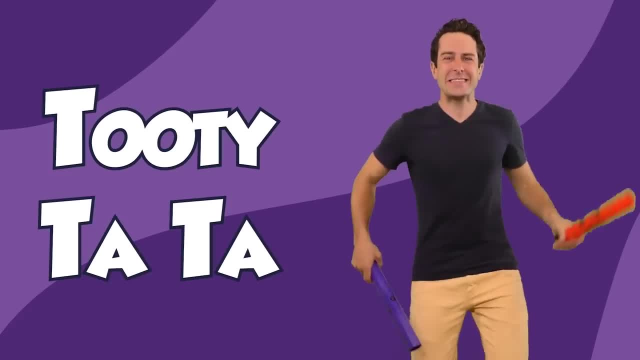 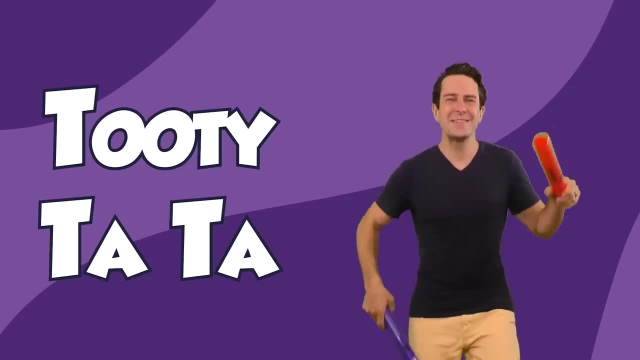 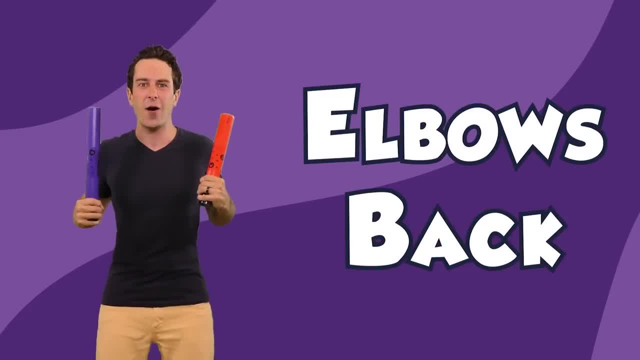 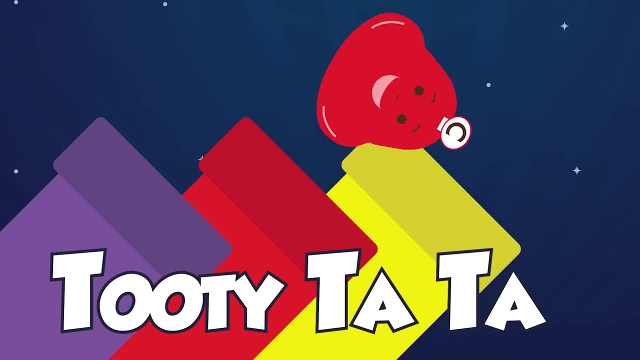 Hands up, Hands up, Elbows back, Elbows back, Feet apart, Feet apart, Knees together, Knees together. Nice Tutti-Tah, Tutti-Tah, Tutti-Tah, Tutti-Tah, Tutti-Tah. 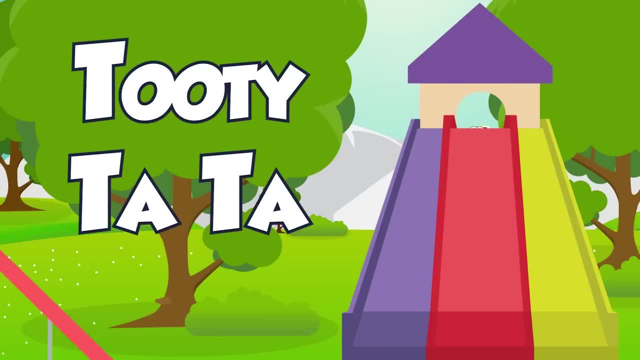 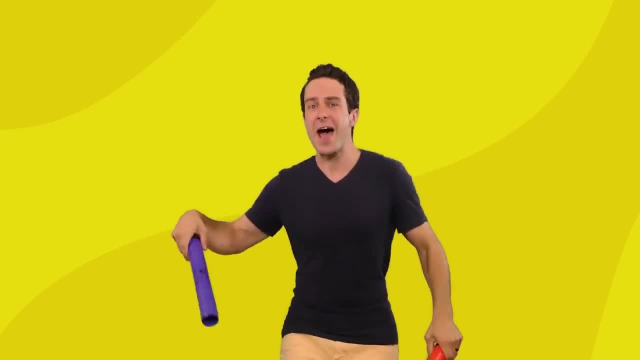 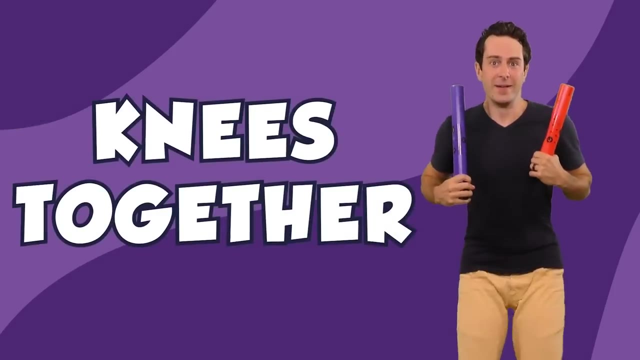 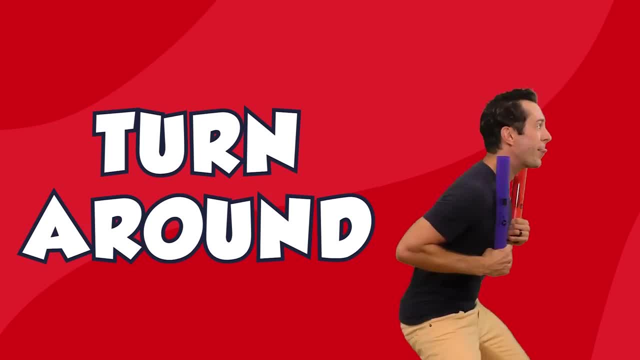 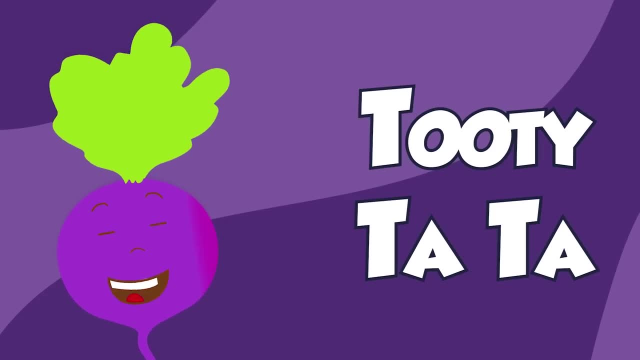 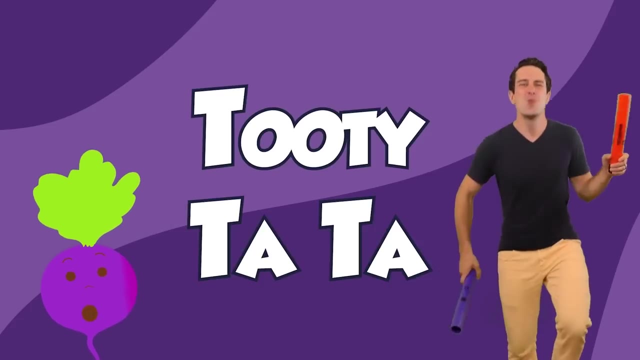 hands up, Hands up, Elbows back, Elbows back, Feet apart, Feet apart, Knees together, Knees together, Bottoms up And up, Tongues out and turns around, And turns around. Nice job, Tutti-Tah, Tutti-Tah, Tutti-Tah. 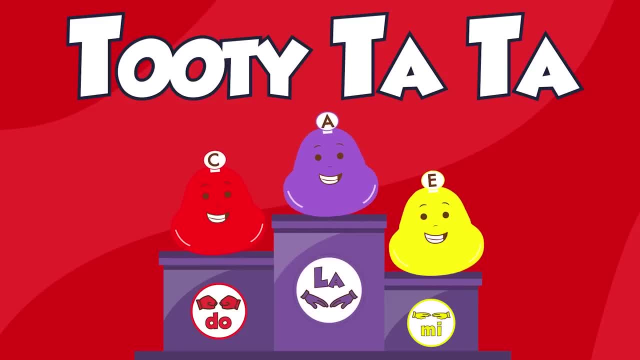 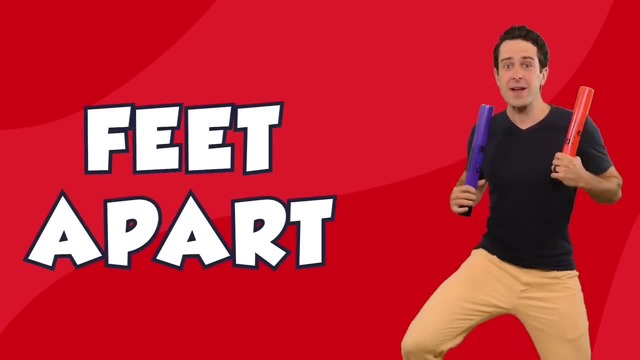 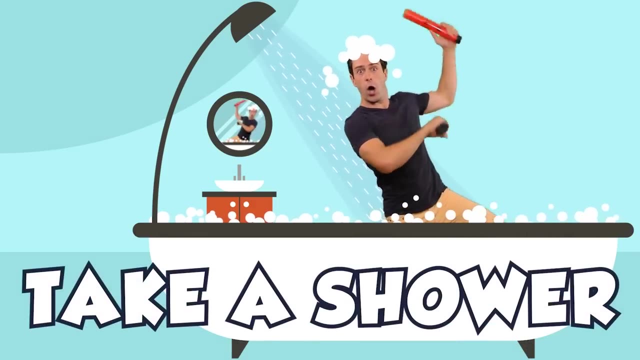 Ta-ta-tootie-ta-ta, Ta-tootie-ta-ta-tootie-ta. Repeat after me. Hands up, Elbows back, Feet apart, Knees together. Take a shower, La-la-la-la-la-la-la-la-la, Brush your teeth. 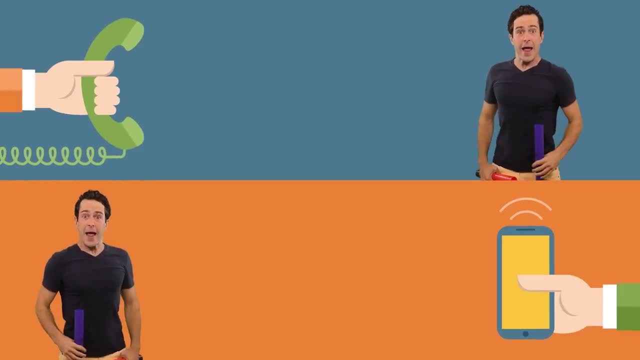 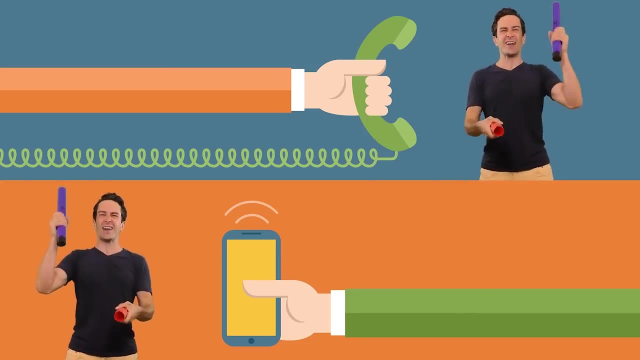 And make a phone call. Hello, how are you doing? It's great to talk, but I've got to go. I'm in the middle of the tootie-ta. I'll talk to you later. Ta-tootie-ta-ta-tootie-ta-ta. 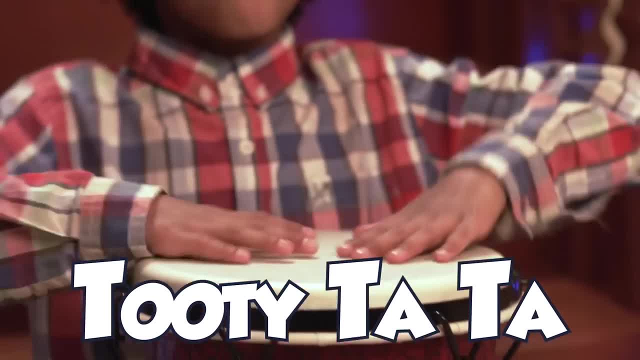 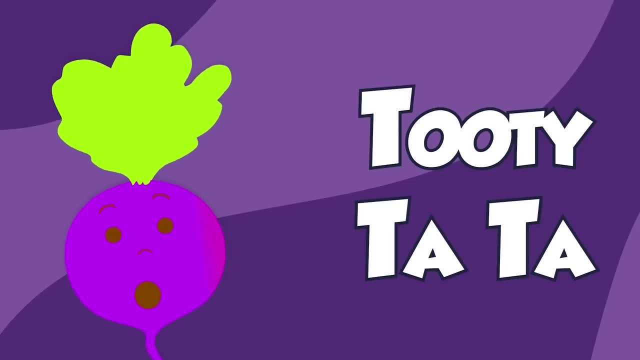 Tootie-ta-ta, Ta-tootie-ta-ta-tootie-ta, Ta-tootie-ta-ta, Ta-tootie-ta-ta-tootie-ta, Ta-tootie-ta-ta, Ta-tootie-ta-ta-tootie-ta. 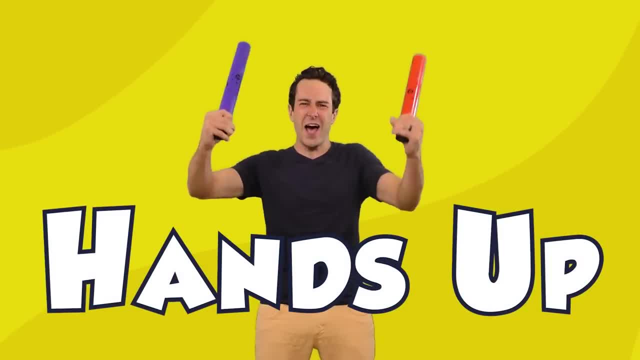 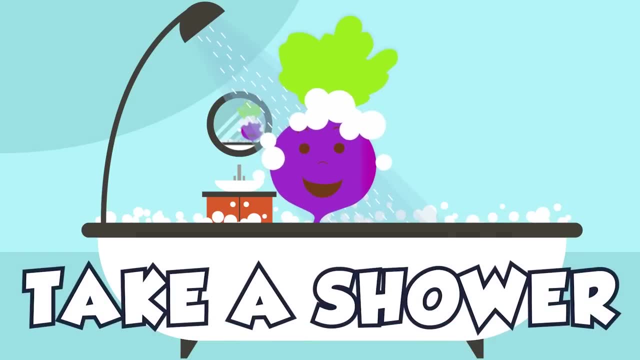 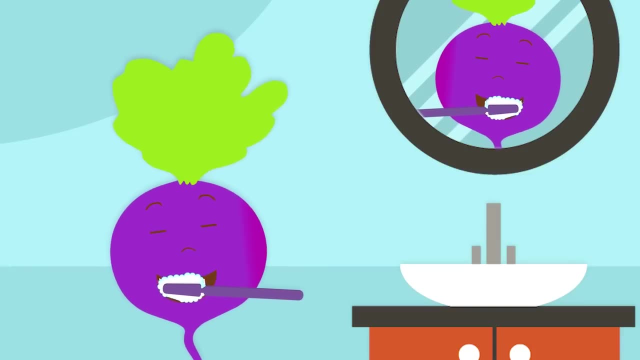 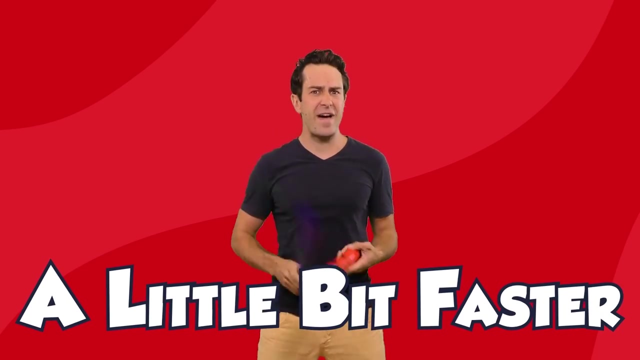 All together. go Hands up, Elbows back, Feet apart, Knees together, Take a shower, La-la-la-la-la-la-la-la, And brush your teeth And make the phone call. Hello, how are you doing? It's great to talk now A little bit faster. try it again. 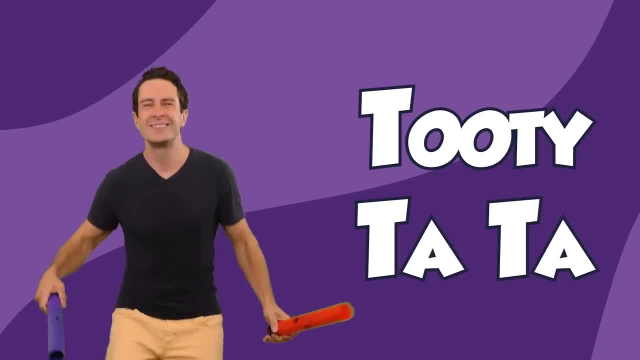 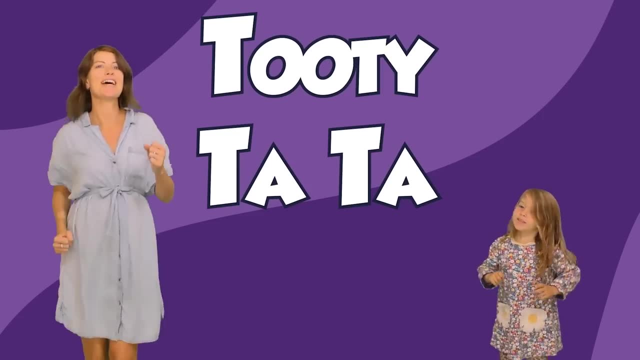 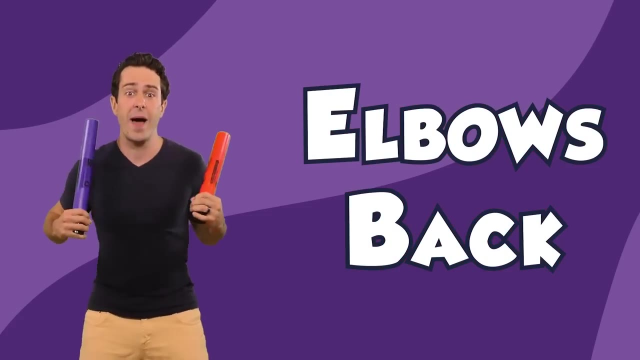 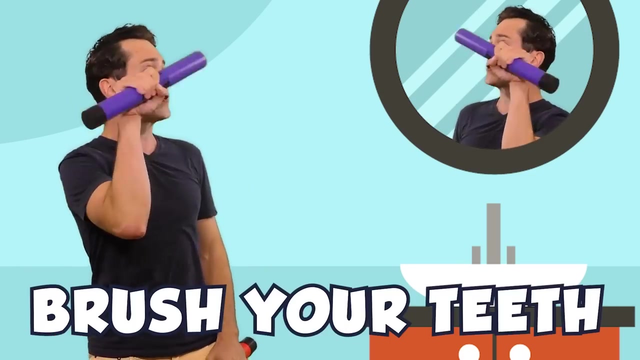 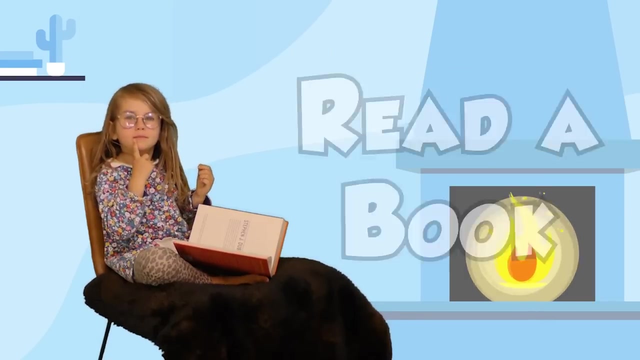 Ready, set, go. Here we go, hands up Elbows back, Feet apart, Feet together. Take a shower, Brush your teeth, Make a phone call. Hello, how are you doing? It's great to talk, Read a book- Very interesting. Hug your mom. I love your mom. 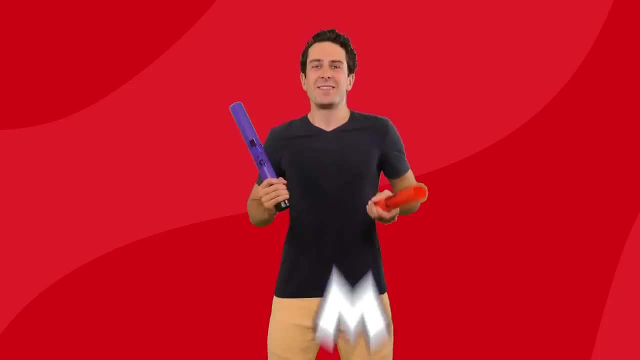 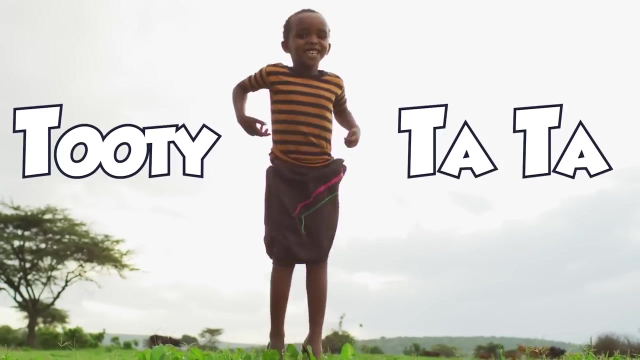 Now jump, jump, jump, jump, Jump and spin. jump and spin One more time While we jump and spin. A-too-dee-dum-dum, too-dee-dum-dum, too-dee-dum-dum, A-too-dee-dum-dum, too-dee-dum-dum. 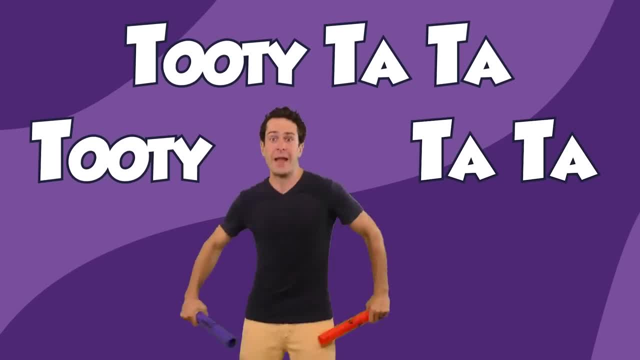 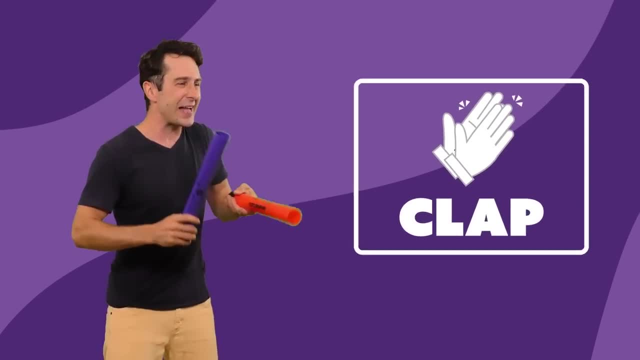 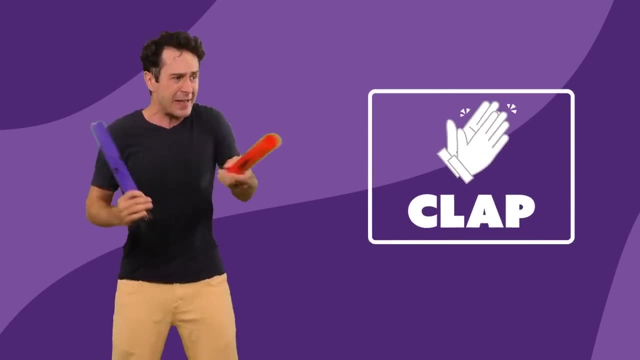 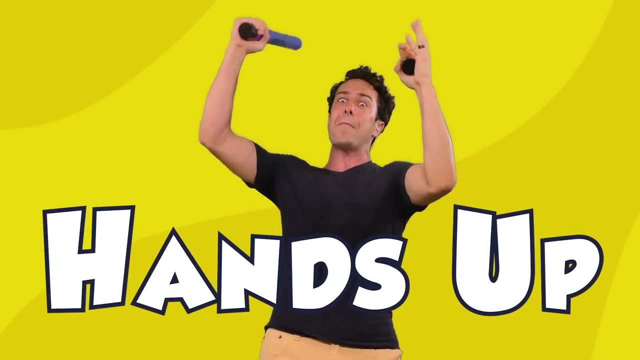 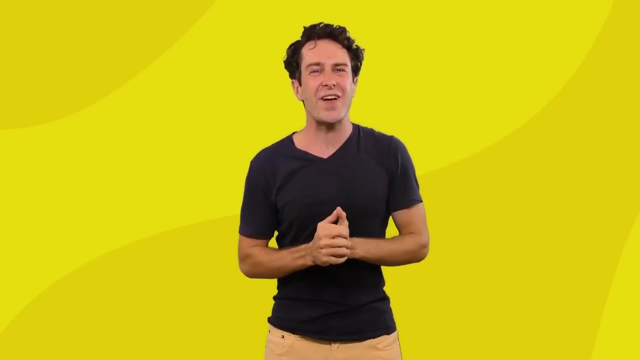 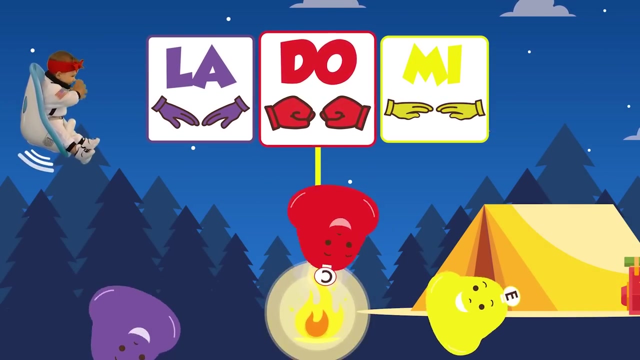 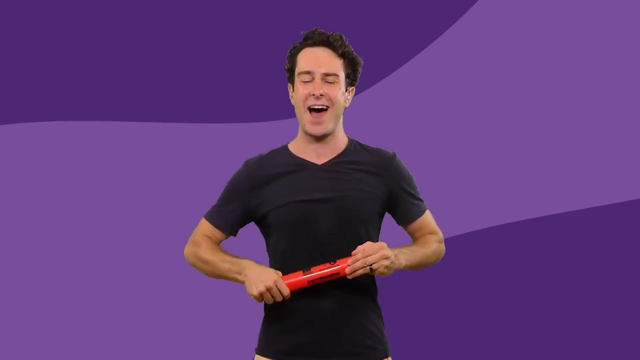 Put your hands up and drop your tubes And give yourself a huge round of applause. Excellent work with the Tutti-Tots. Thank you so much for being here. happy Musicking and until next time I will See ya later. see ya later. see ya. 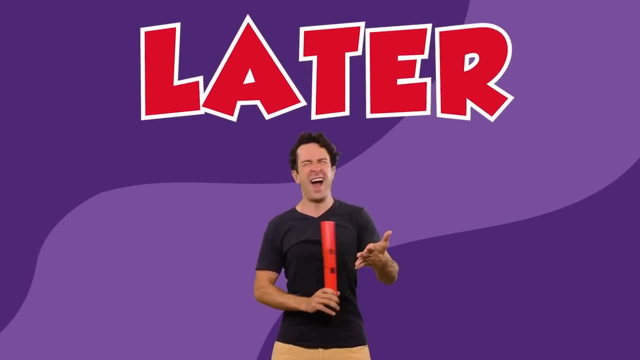 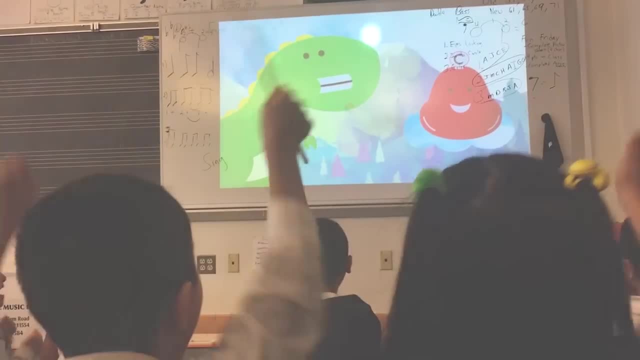 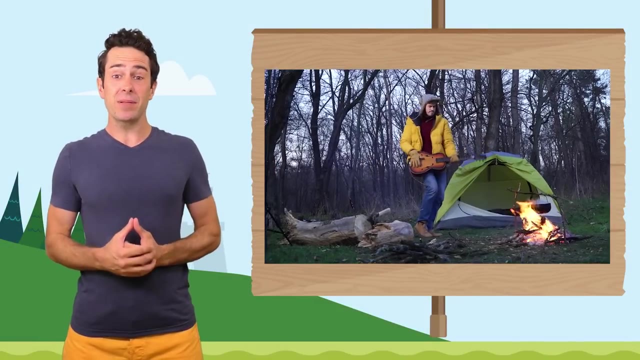 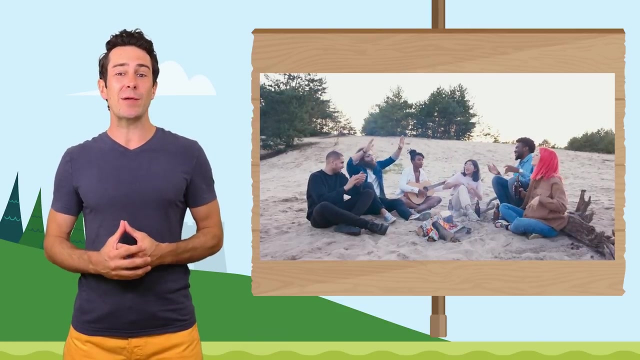 see ya later. Nice dancing with the Tutti-Tot everyone. One of my favorite places to play music is around a bonfire with some friends. Lots of different instruments, lots of different voices, and today we're going to use our voices as we check out lots of different. 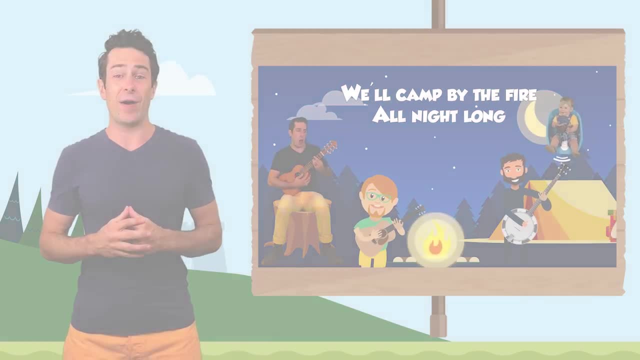 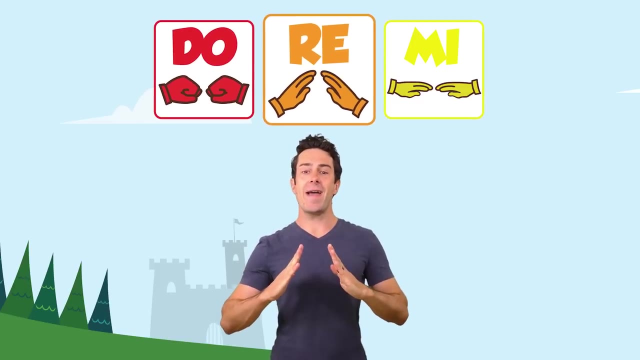 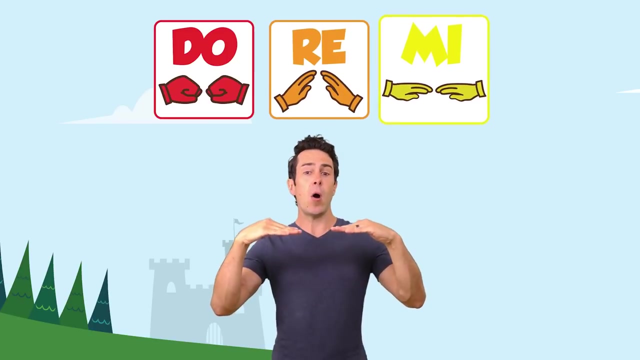 instruments. in one of my favorite songs, Campfire Song, We're going to see these three hand signs a lot. Can you sing with them? And doooo Ray Me, You sing it. go, Doooo Ray Me. 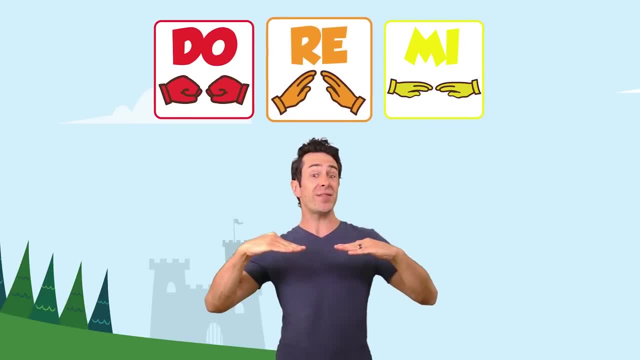 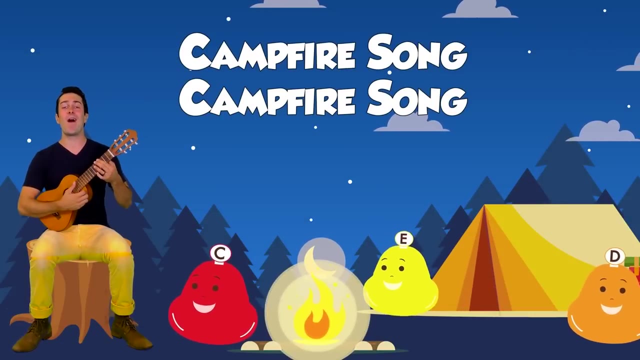 One more time. we have fists and then rising hands and then flat hands for Doooo Ray Me. Nice job, Let's hop into Campfire Song. Campfire Song, Campfire Song. sing and sign and play along Campfire Song. 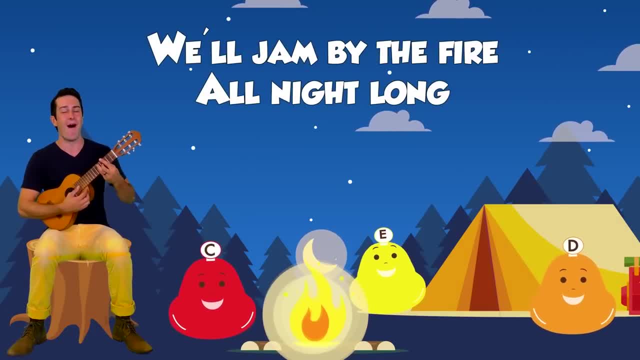 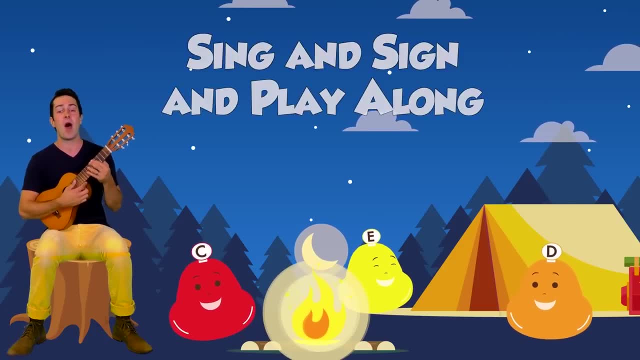 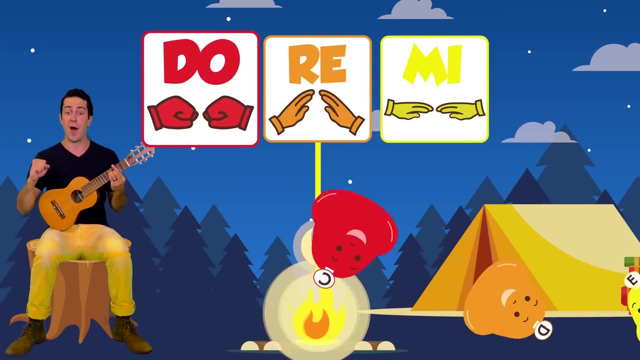 Campfire Song. we'll jam by the fire all night long. Campfire Song, Campfire Song. sing and sign and play along. Campfire Song, Campfire Song. we'll jam by the fire all night long With Doooo Ray. 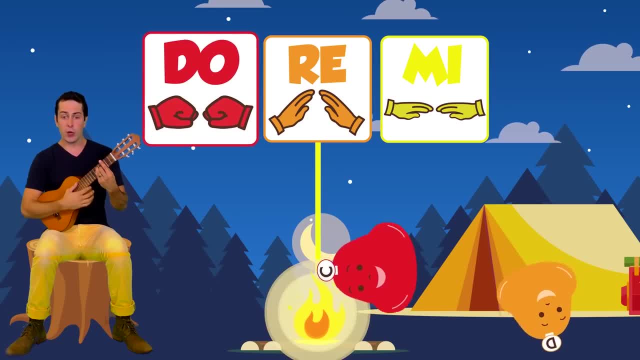 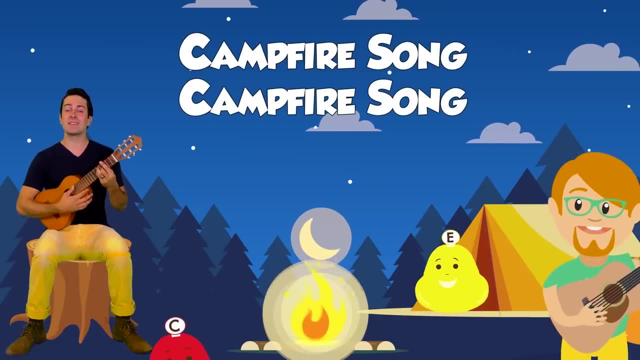 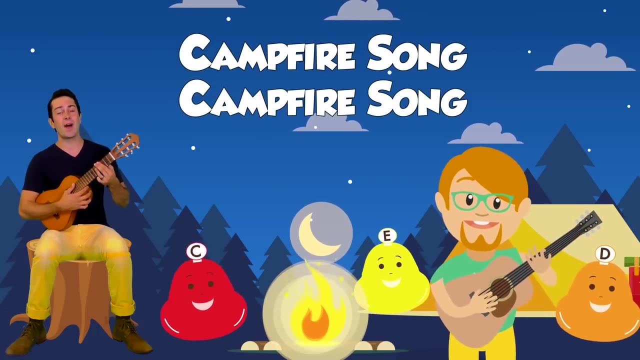 and Me. You sing it. Doooo Ray Me Nice Campfire Song, Campfire Song. sing and sign and play along Campfire Song, Campfire Song. we'll jam by the fire all night long. It's Campfire, John. 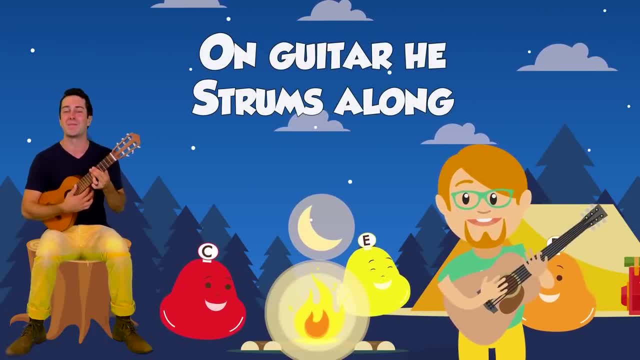 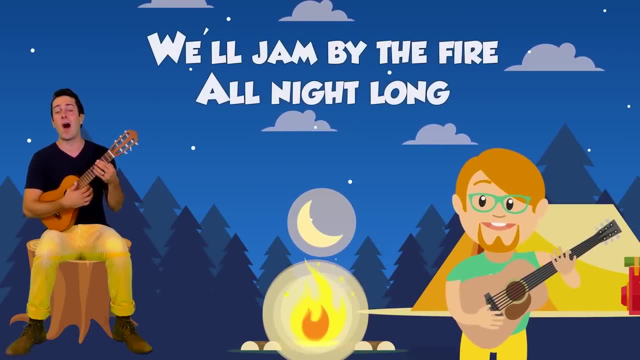 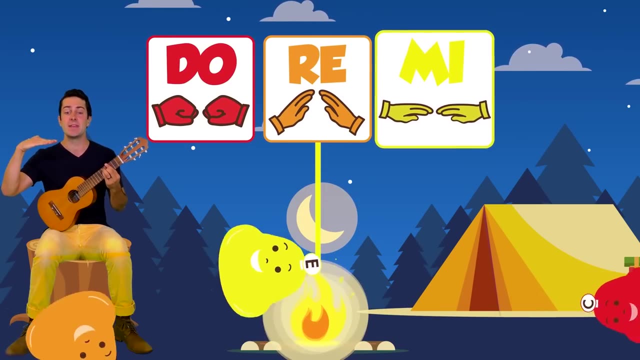 Campfire John on guitar. he strums along To our Campfire Song. Campfire Song, our Campfire Song. we'll jam by the fire all night long With Doooo Ray and Me. You sing it, Doooo Ray and Me. 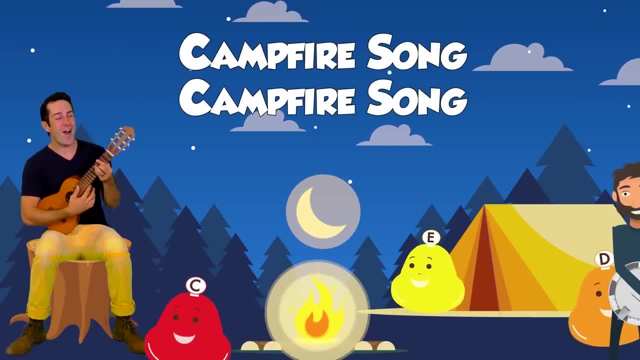 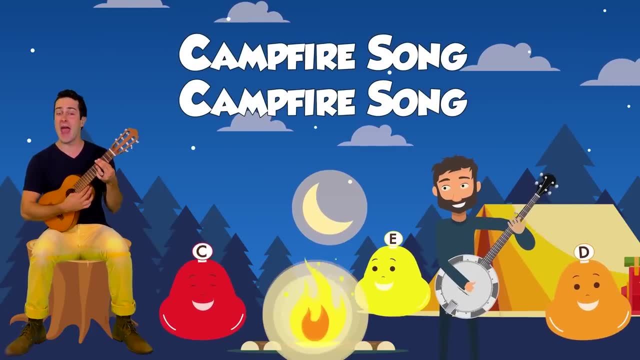 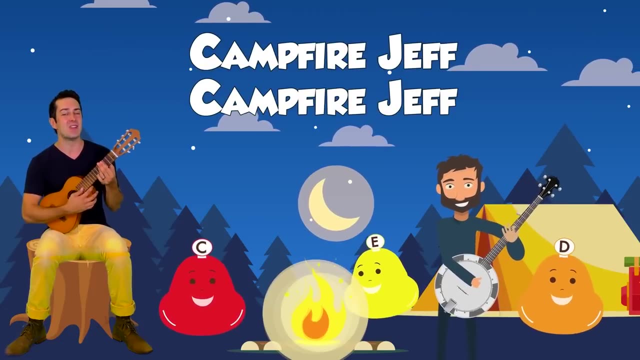 Nice Campfire Song. Campfire Song. sing and sign and play along. Campfire Song, Campfire Song. we'll jam by the fire all night long. It's Campfire Jeff, Campfire Jeff on banjo and he shreds. 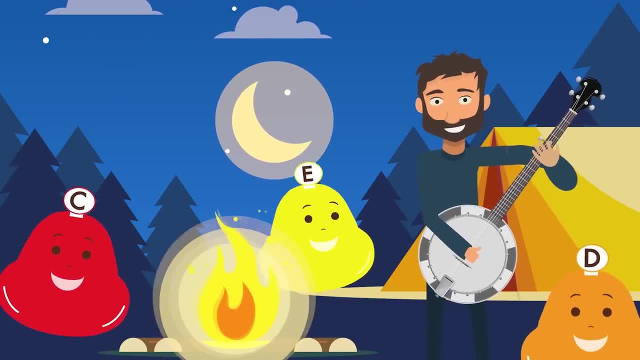 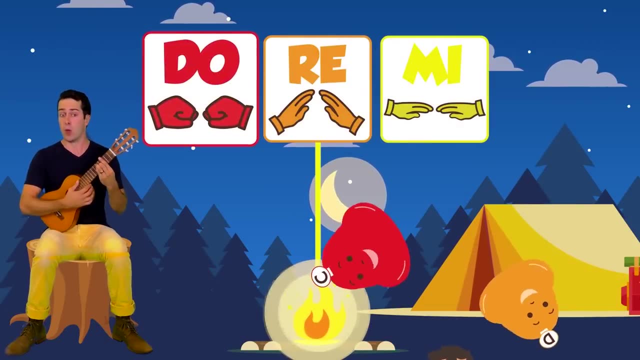 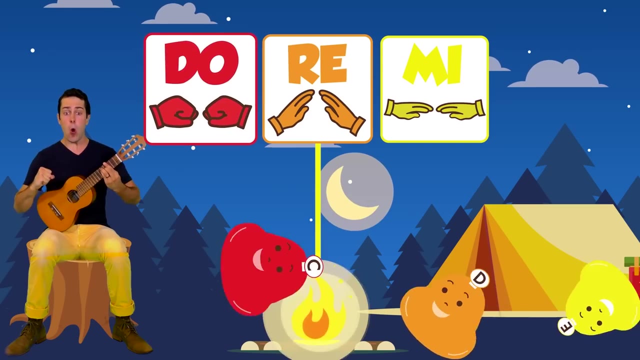 the best To our Campfire Song, our Campfire Song. we'll jam by the fire all night long With Doooo Ray and Me. You sing it, Doooo Ray, Me Nice Campfire Song. Campfire Song. 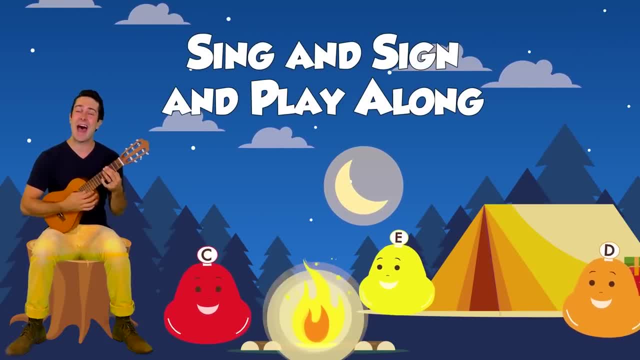 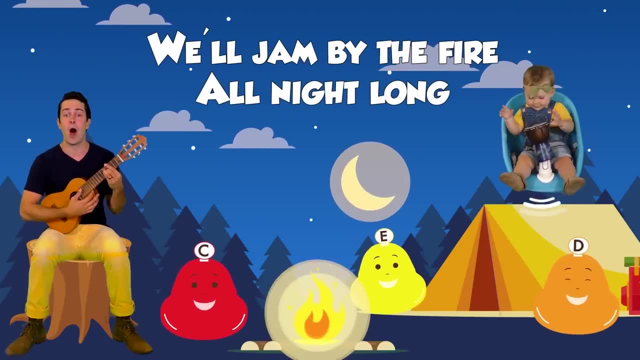 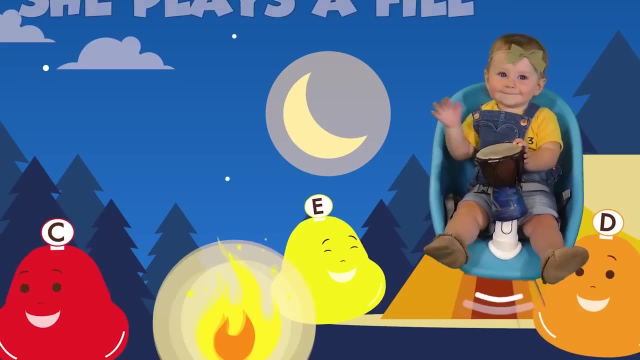 Campfire Song. sing and sign and play along Campfire Song. Campfire Song, we'll jam by the fire all night long. It's Baby Lil, Baby Lil on her drums. she plays a fill, Nice, fill Lil To our Campfire Song, our Campfire Song. 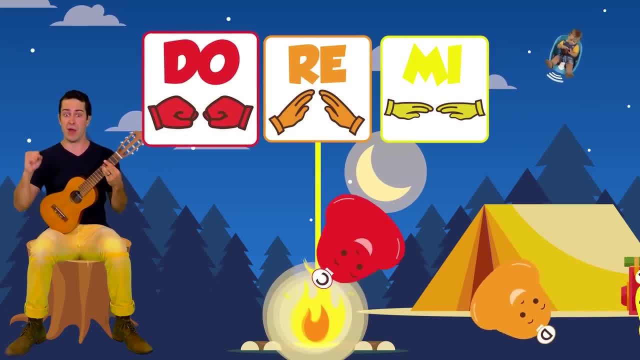 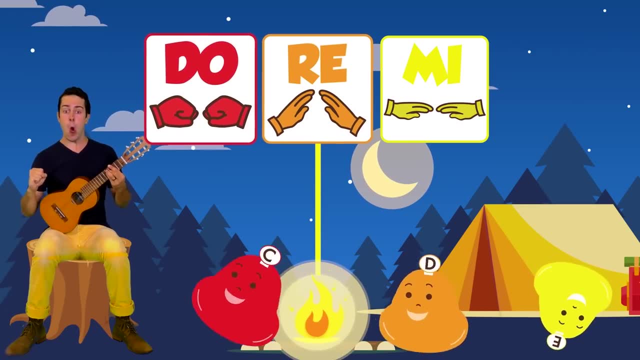 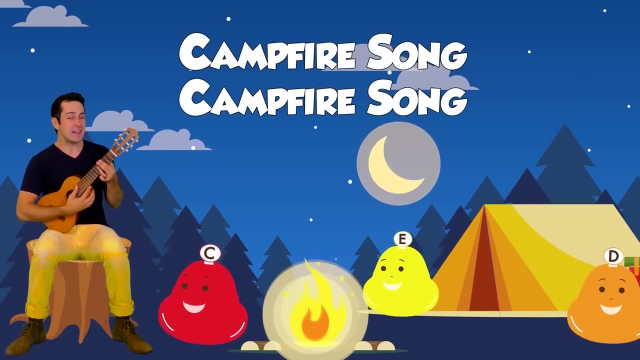 we'll jam by the fire all night long With Doooo Ray and Me. You sing it, Doooo Ray, Me Nice job. Campfire Song. Campfire Song. sing and sign and play along Campfire Song. 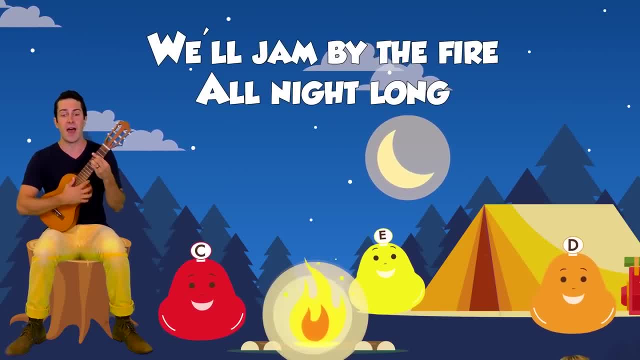 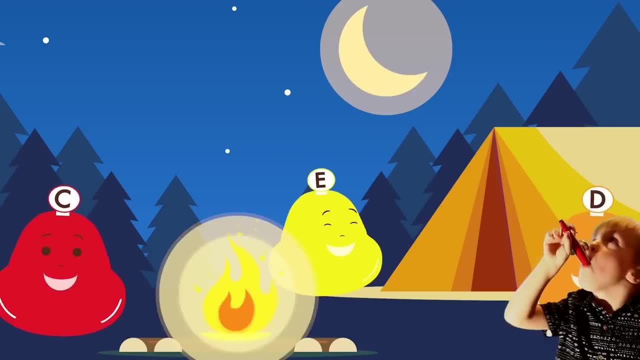 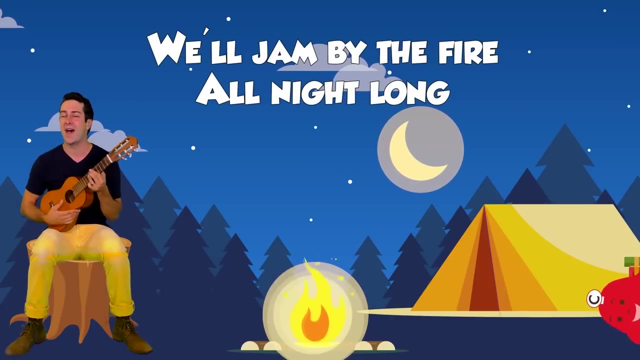 Campfire Song. we'll jam by the fire all night long. It's Campfire Boo, Campfire Boo. on his kazoo he toots a tune Nice To our Campfire Song. our Campfire Song. we'll jam by the fire all night long. 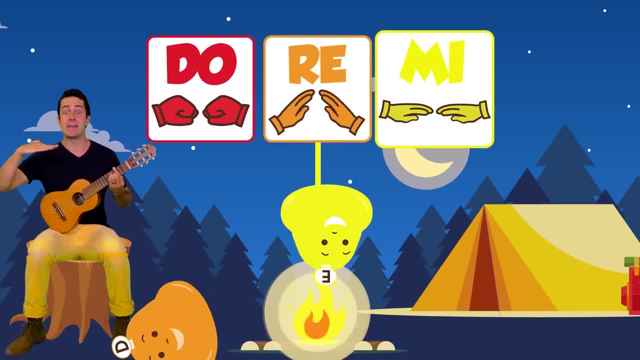 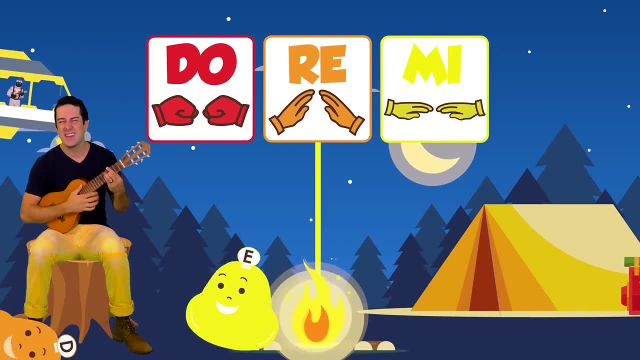 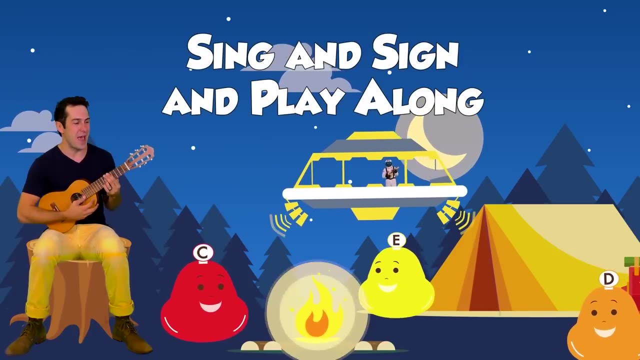 With Doooo Ray and Me. You sing it, Doooo Ray and Me, Nice job. Campfire Song, Campfire Song. sing and sign and play along. Campfire Song, Campfire Song. we'll jam by the fire all night long. 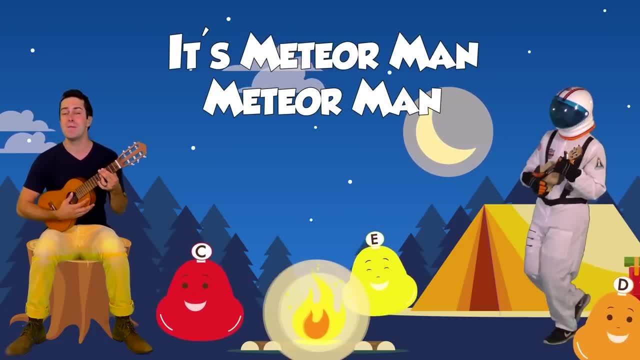 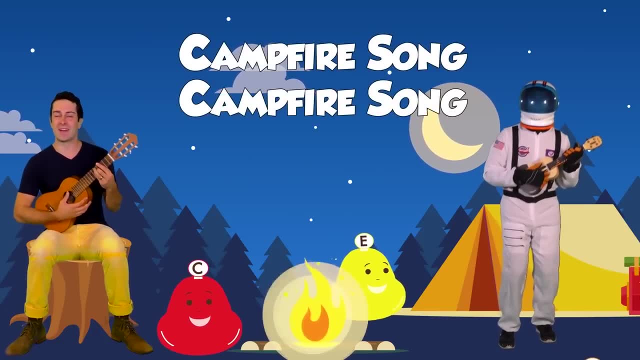 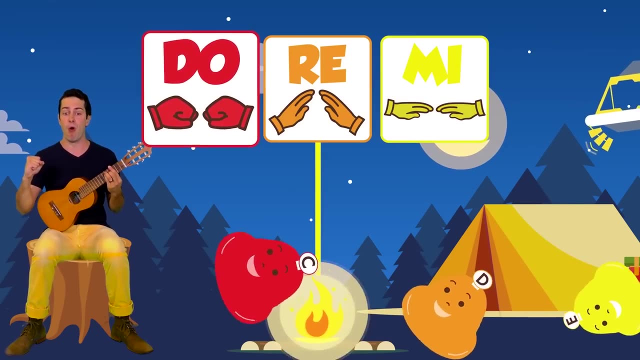 It's Meteor Man, Meteor Man. one small step for Campfire Jams. With our Campfire Song, our Campfire Song, we'll jam by the fire all night long. With our Campfire Song, our Campfire Song, we'll jam by the fire all night long. 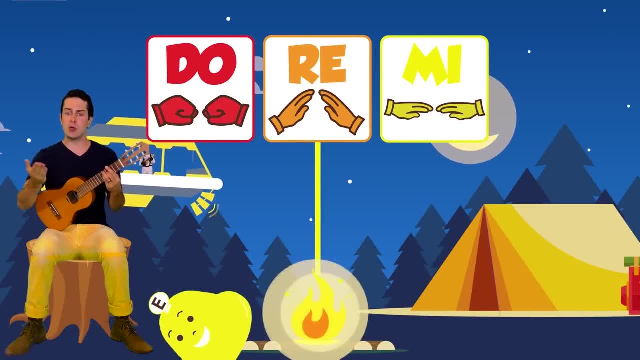 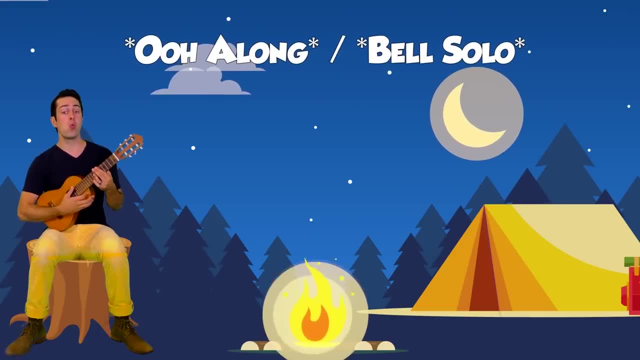 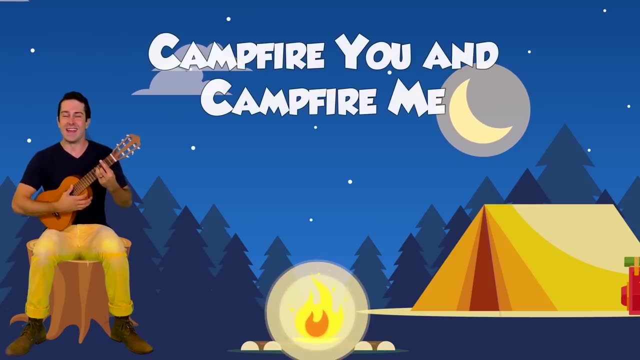 We'll jam by the fire all night long. Doooo Ray and Me. You sing it. Doooo Ray and Me. Can you OO along or take a little balance along? You sing it, Doooo Ray and Me. 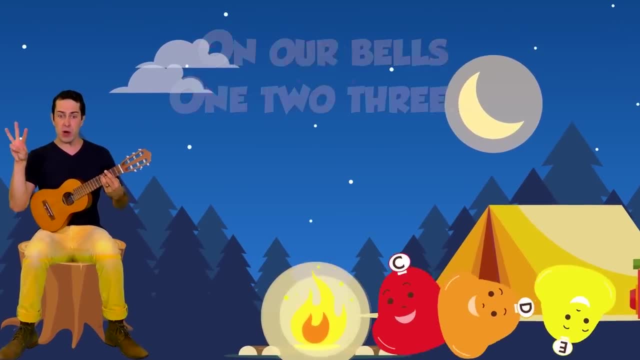 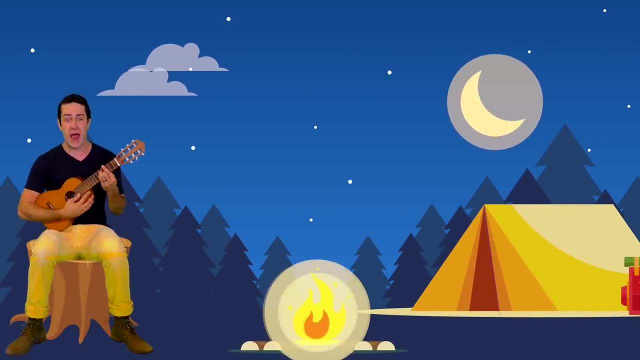 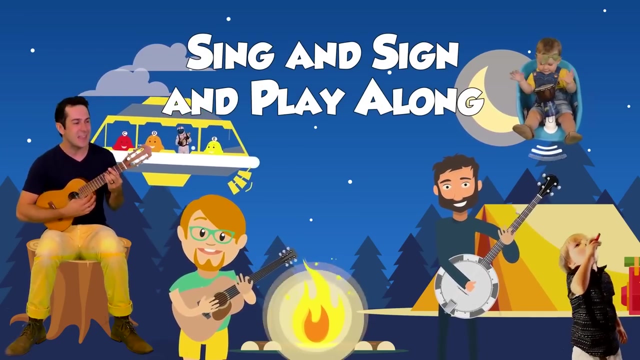 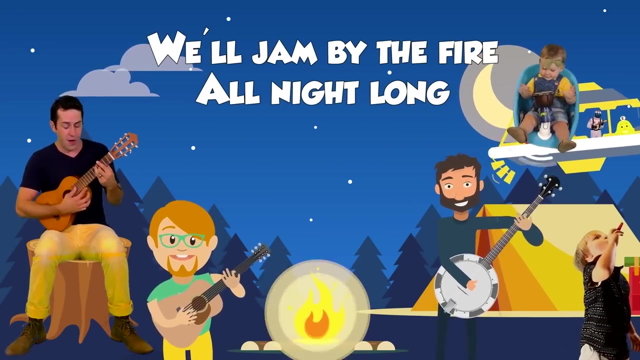 fire me on our bells: one, two, three. one, two, three, four. campfire song, our campfire song, we'll jam by the fire all night long. campfire song, campfire song. sing and sign and bend along campfire song, campfire song, we'll jam by the fire all night long. 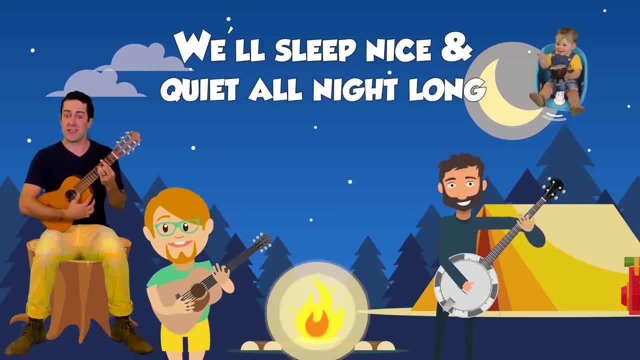 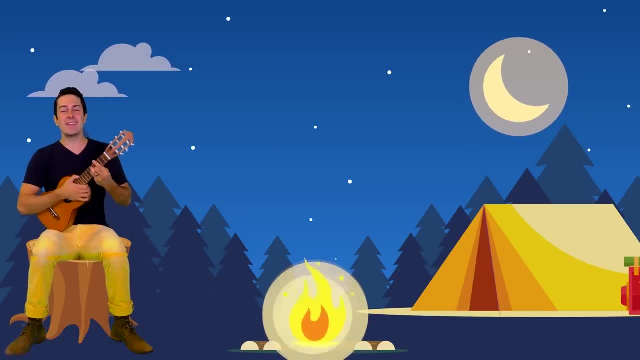 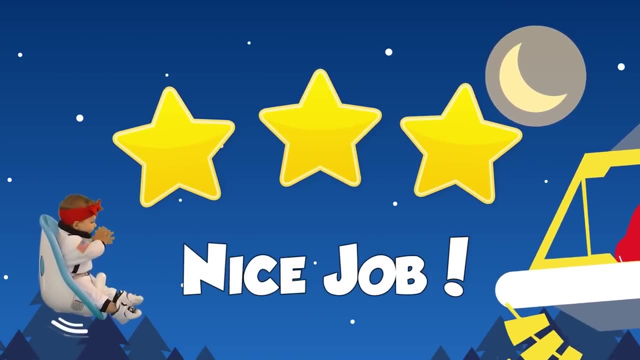 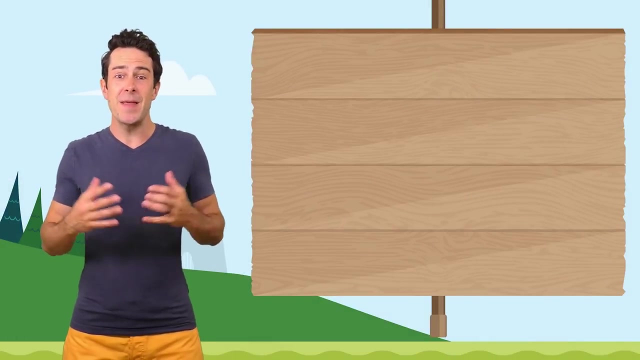 campfire song, campfire song. we'll camp by the fire all night long. give yourself a huge round of applause. excellent job playing campfire song, everybody Man. I just love having campfires with my friends and in this next one, one of our friends, boo, is going to use his voice to guide you. 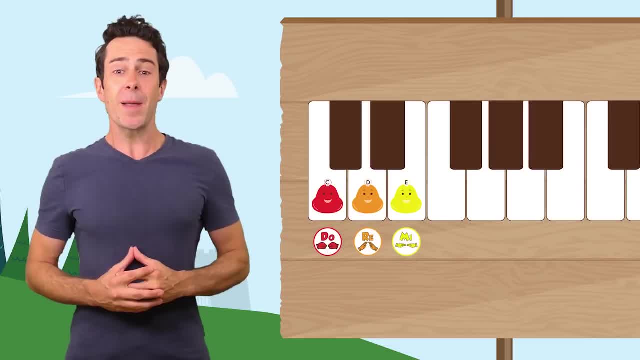 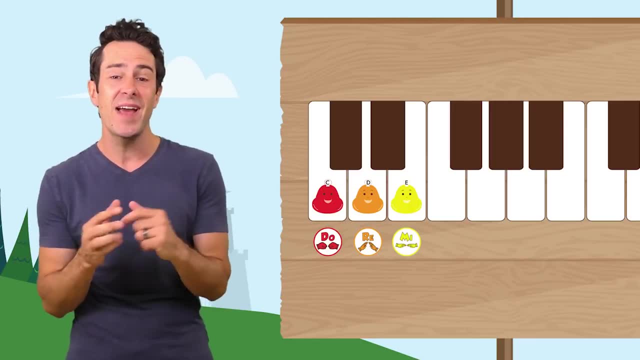 through our campfire song, learning a few more hand signs. In the last song we did do re mi, which are musical steps. There are little tiny steps that we can take, but now we're going to do some musical skips. These are: 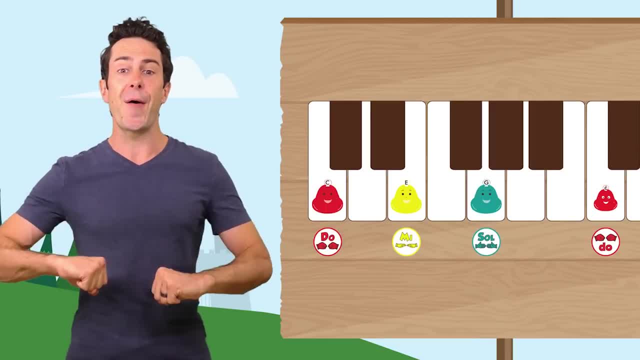 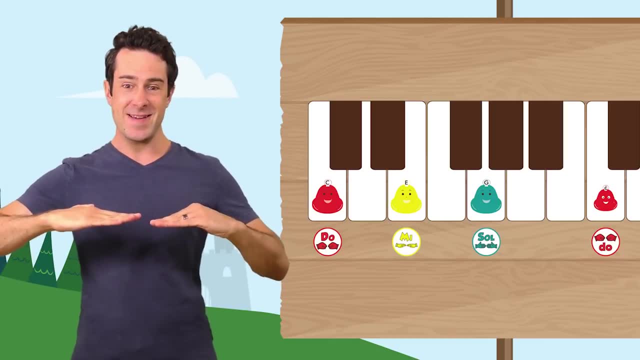 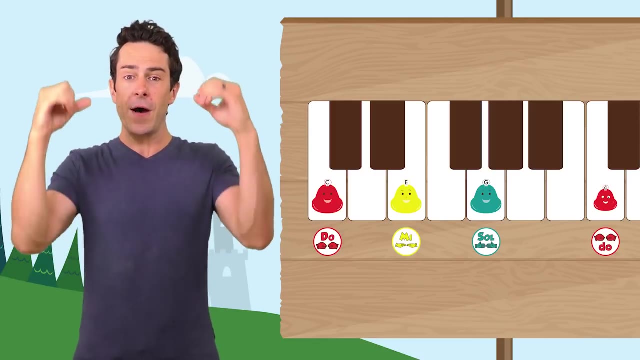 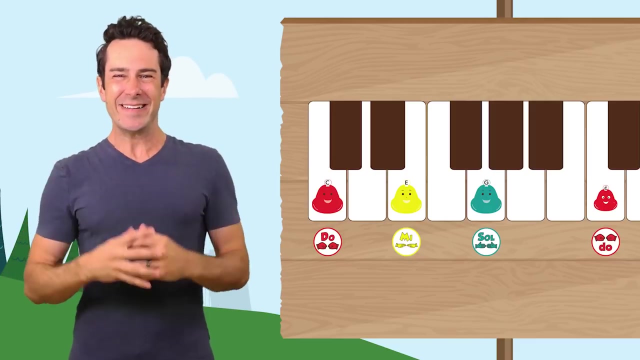 bigger skips that we can take in music and we're going to go. do mi sol, do You sing? Do mi sol do Again. Do mi sol do One more time. Do mi sol do- Nice, Now that we've got the hand signs warmed up. 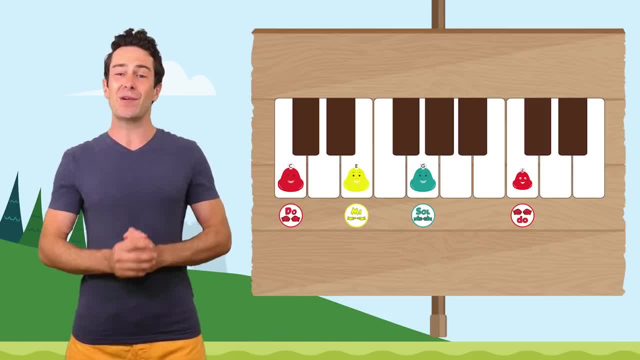 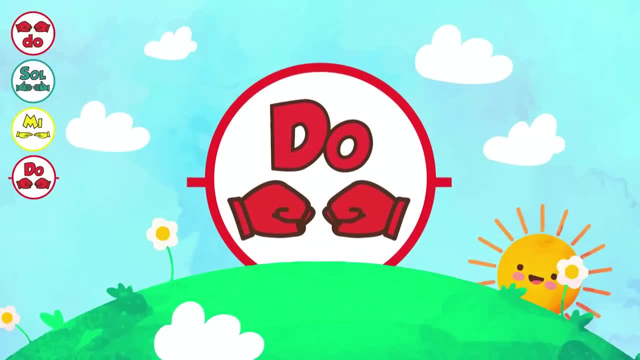 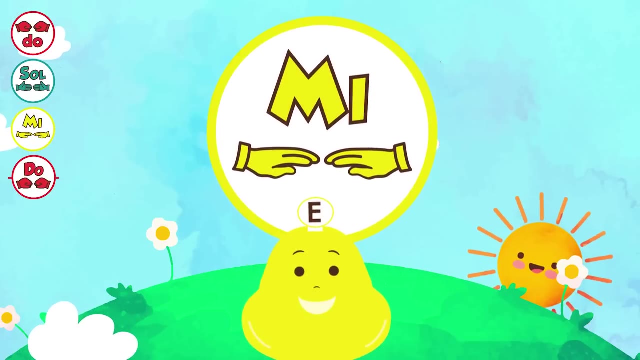 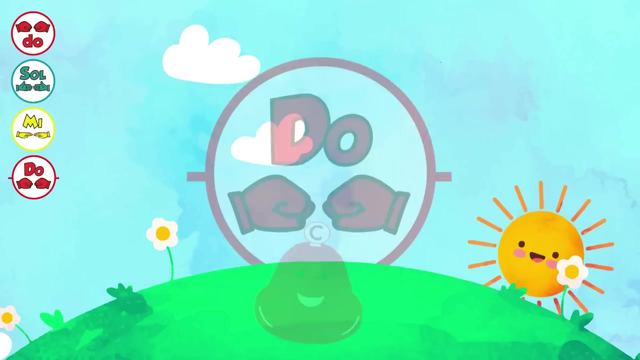 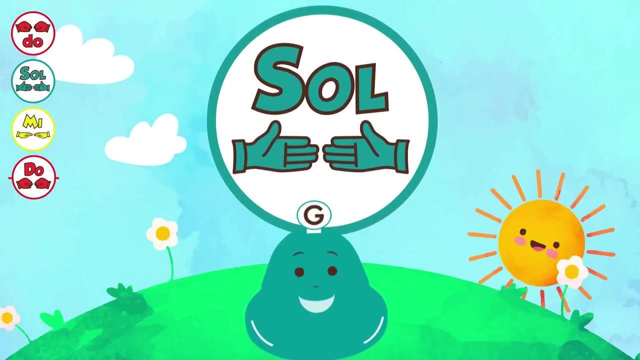 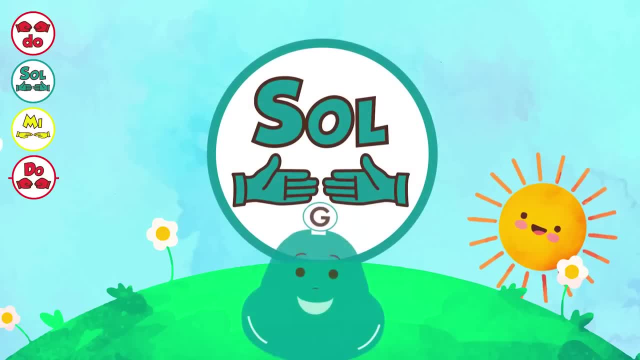 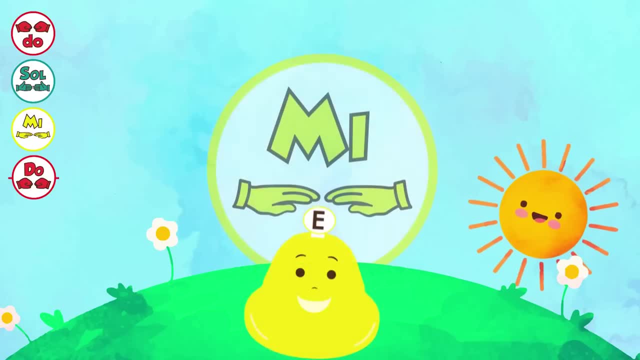 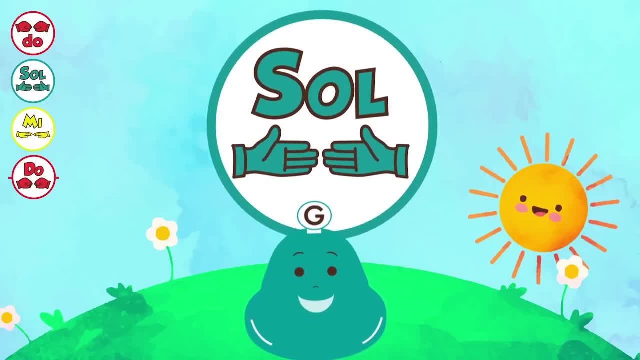 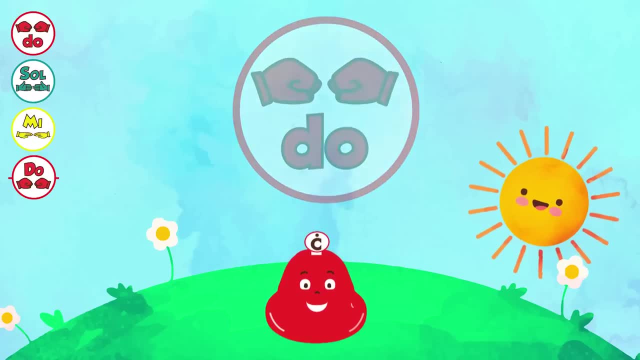 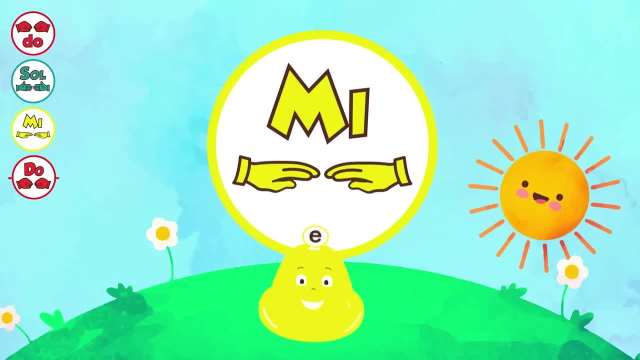 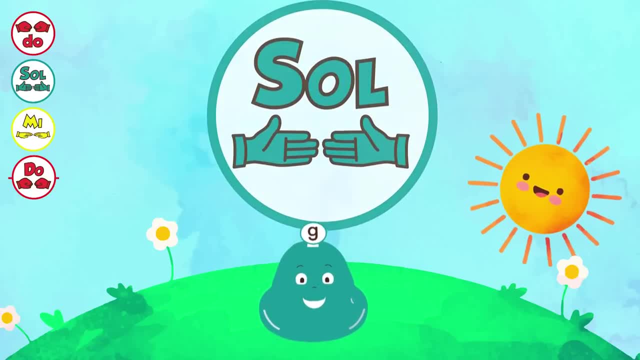 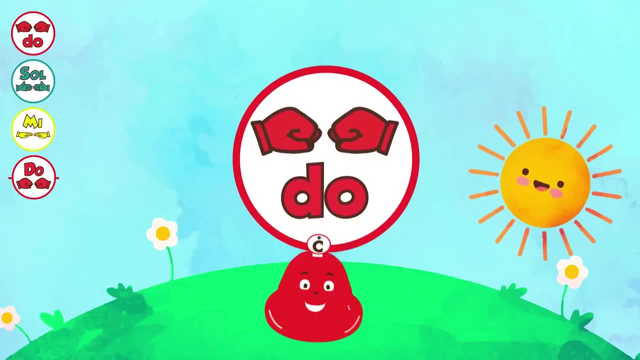 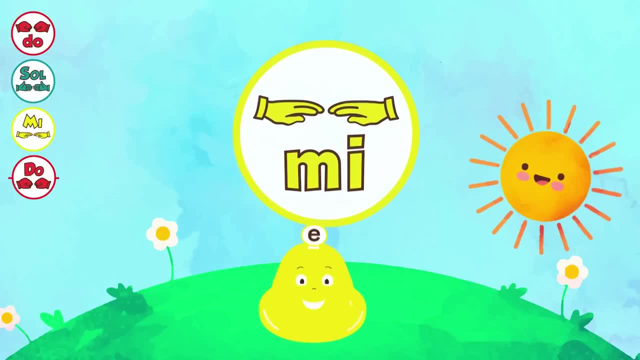 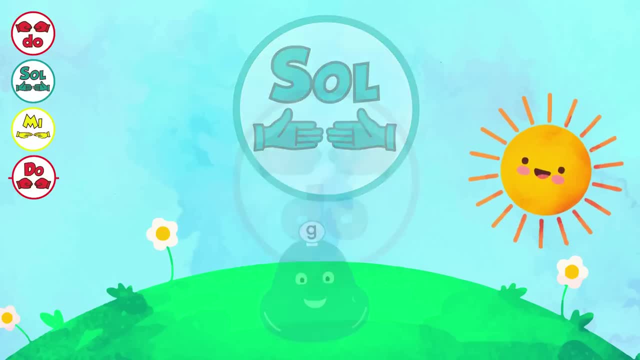 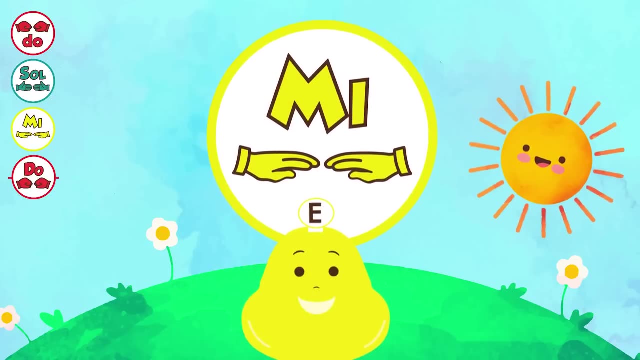 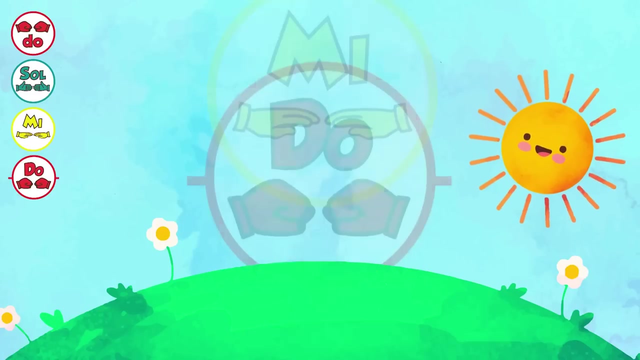 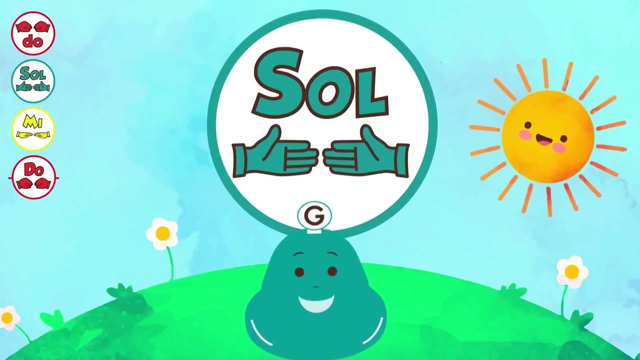 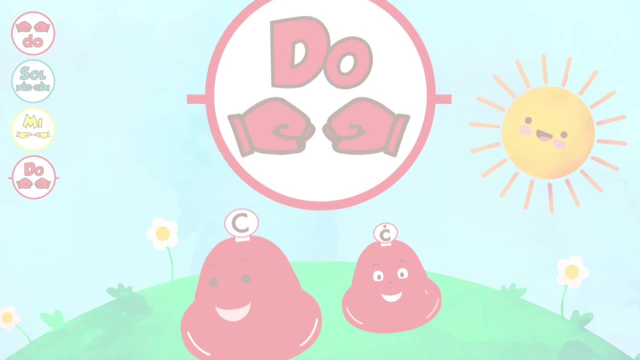 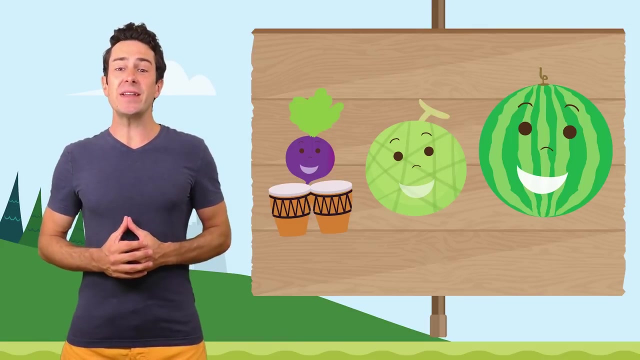 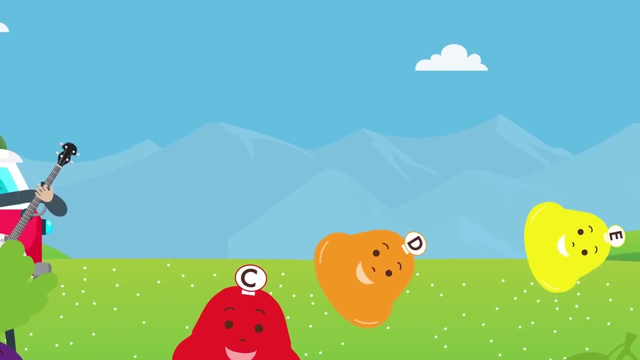 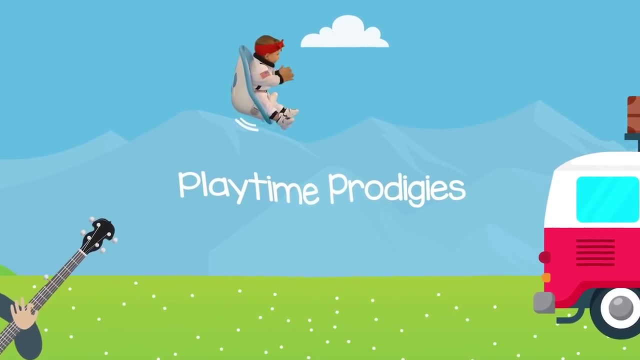 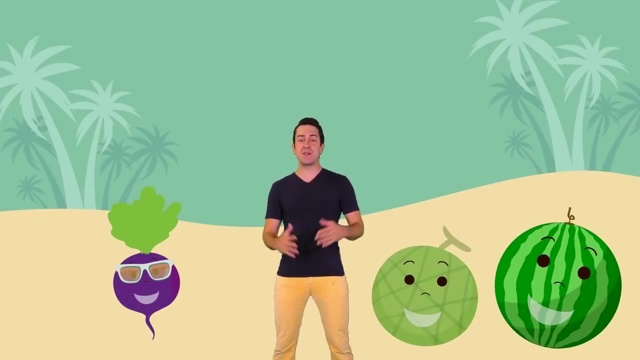 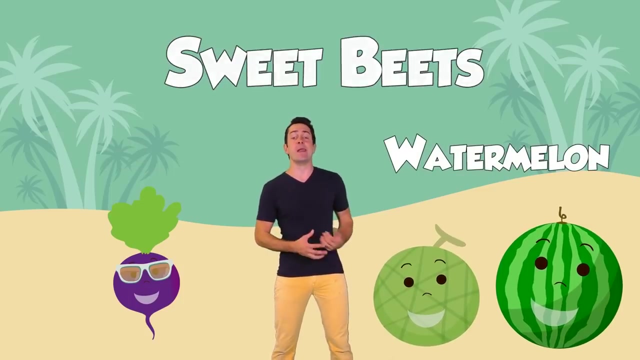 🎵. Nice work with all of those hand signs, everyone. Let's hop back into singing some sweet beats, but this time with beat MELON and WATERMELON. Hey, everyone, and welcome back to Sweet Beats. Today we're going to play Sweet Beats with beat melon and watermelon. 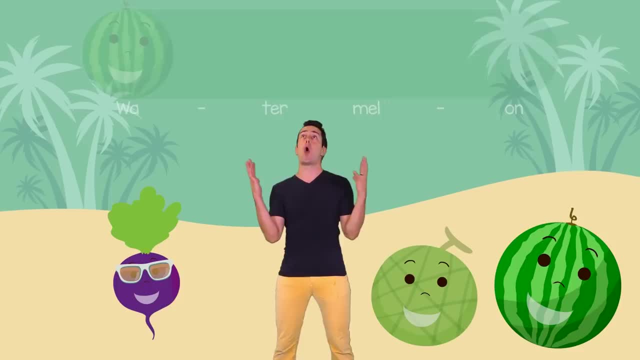 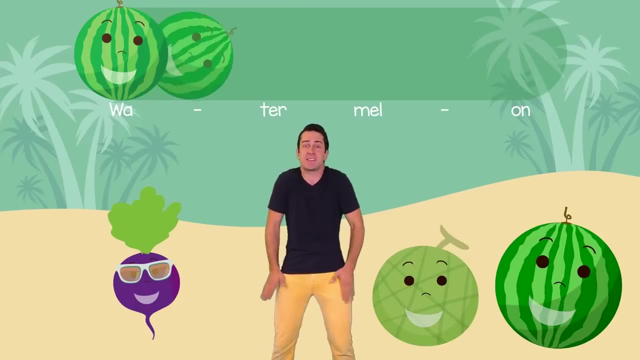 The watermelon is even bigger than the melon. it's going to take up our whole musical space and when we see that watermelon we're going to roll on our legs really quick like this. Can you roll with me? Yeah, Just like that. 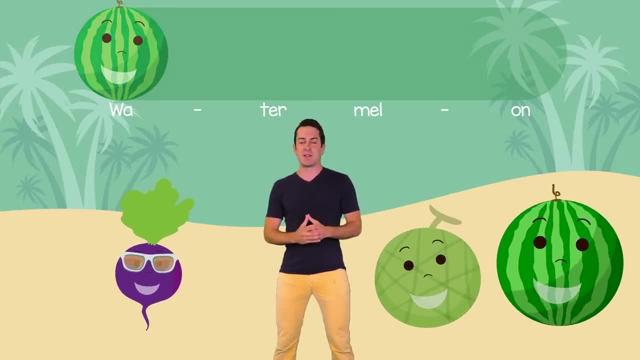 So, whenever you see the watermelon, we're going to roll on our legs really quick, like this: If you see the watermelon, that is what we are going to do. Alright, so we're going to tap on our legs and have a lot of fun playing Sweet Beats. 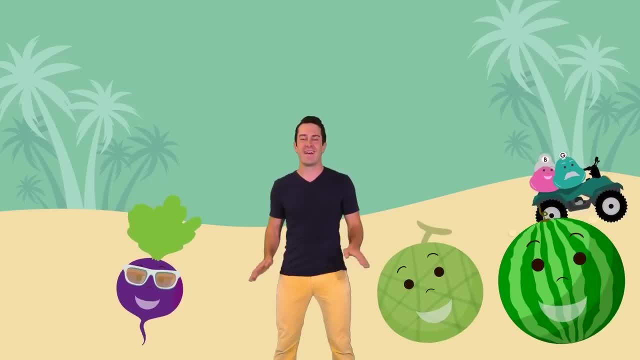 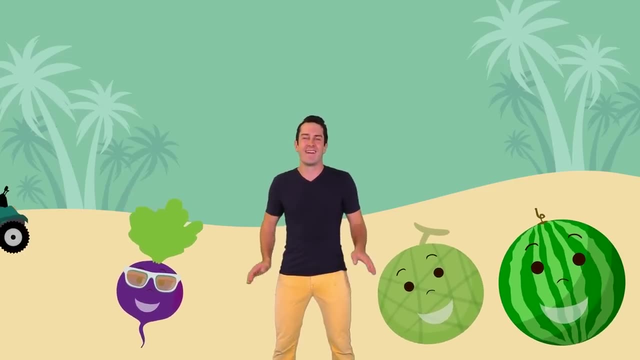 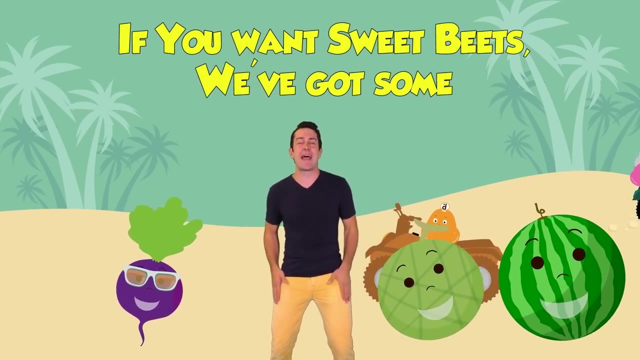 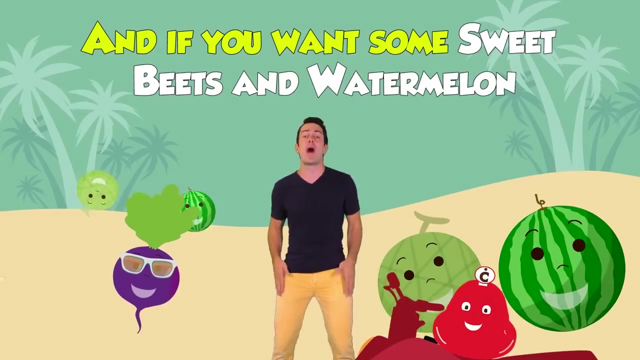 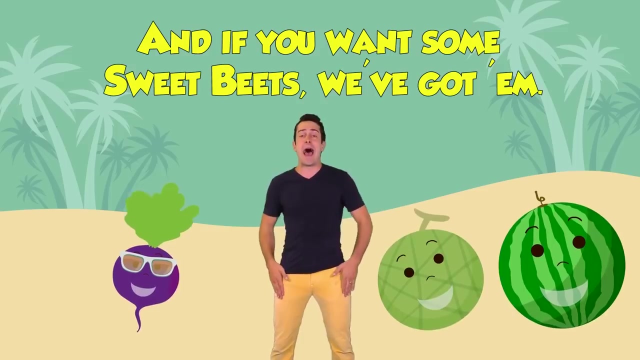 together. Ready set. Make sure you sing those choruses nice and loud with me. alright, You fruits ready. If you want sweet beats, we've got some. And if you want some sweet beats, we've got some. And if you want some, 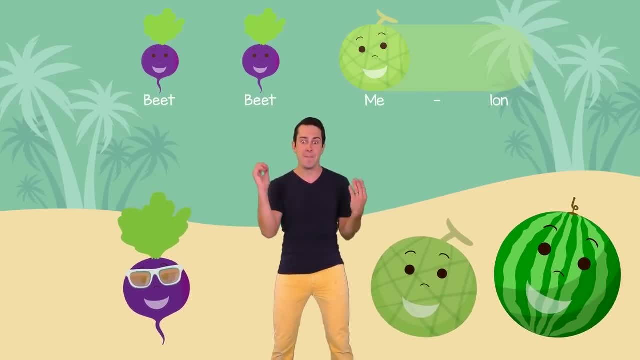 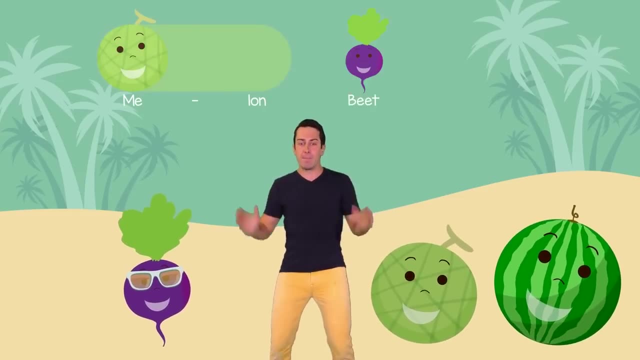 sweet beats, we've got some. And if you want some sweet beats, we've got some. Alright, repeat after me. Beat, beat, melon, Watermelon, Melon. Beat beat Watermelon, Melon, melon, watermelon. 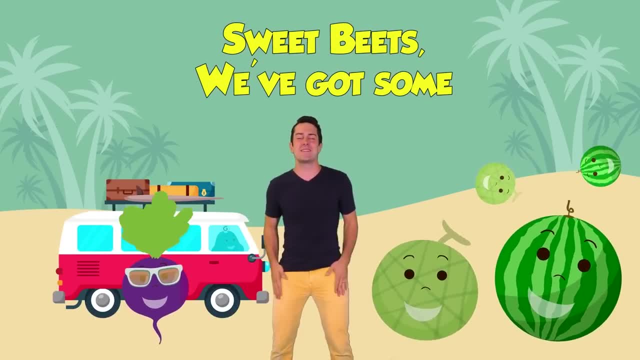 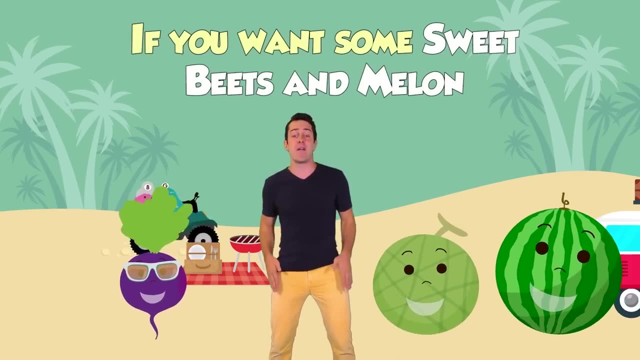 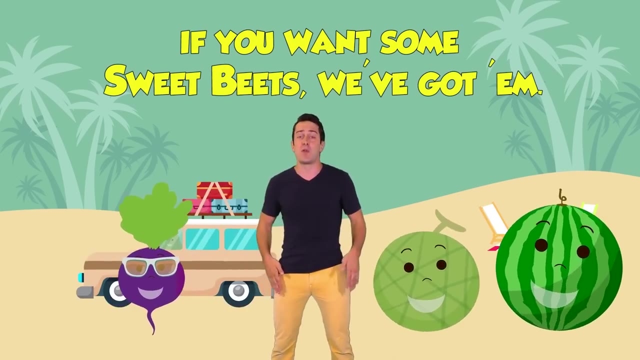 Watermelon, Melon, Sweet beets- oh, we've got some. And if you want some sweet beets, oh we've got them. And if you want some sweet beets and melon, And if you want some sweet beets, oh, we've got them. 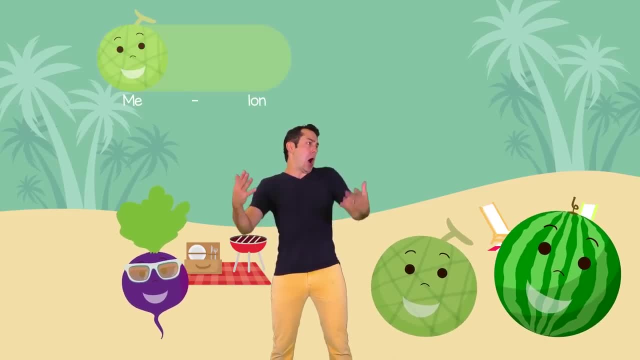 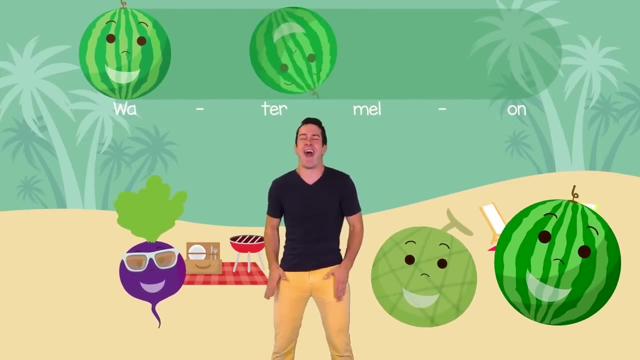 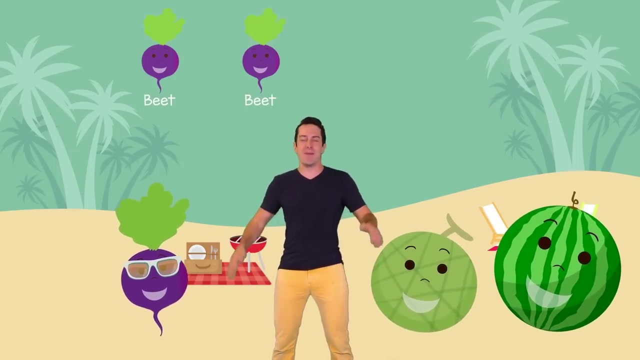 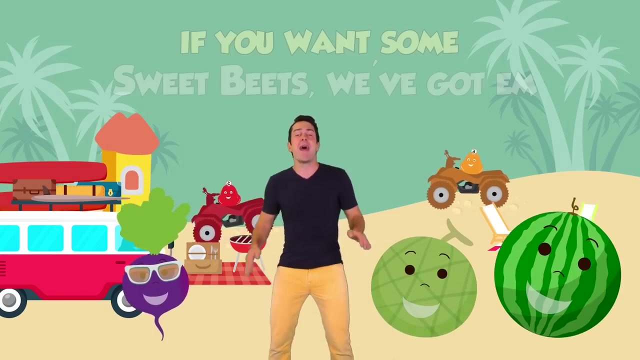 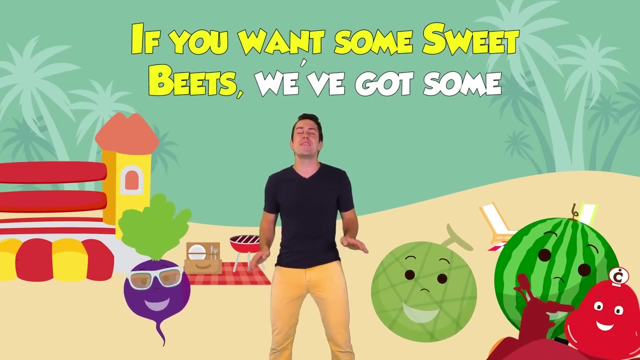 Repeat after me again: Melon, melon, Watermelon, Beet, beet, melon, Beet, beet, beet, beet. Nice job. Sweet beets, oh, we've got some. And if you want some sweet beets, oh, we've got them. And if you want some sweet beets, oh, we've got some. And if you want some sweet beets, oh, we've got them. 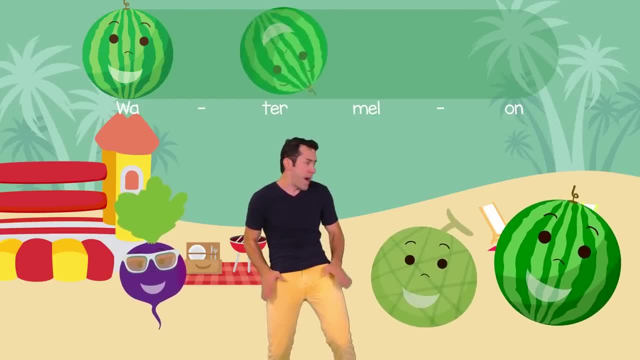 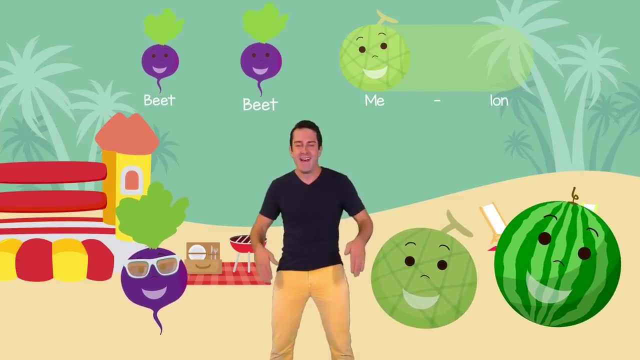 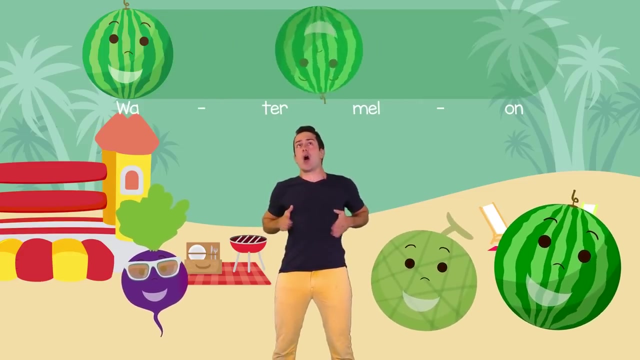 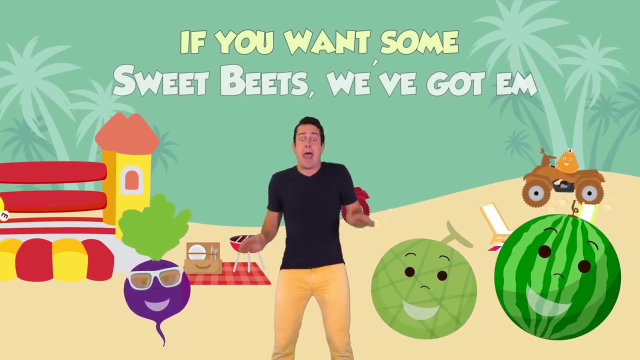 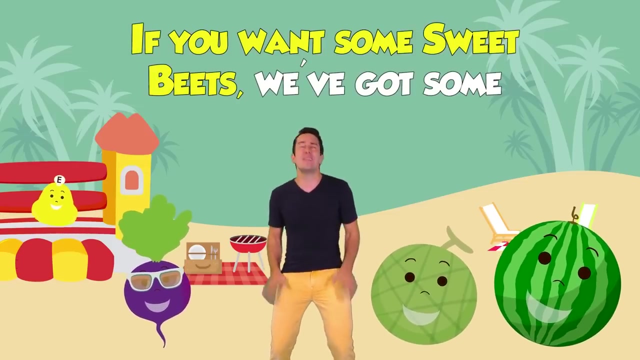 Alright, all together, we've got Watermelon, Watermelon, Beet beet, melon, Nice melon, Beet beet, Watermelon, Sweet beets- oh, we've got some. And if you want some sweet beets, oh, we've got them. Yeah, And if you want some sweet beets, oh, we've got some. 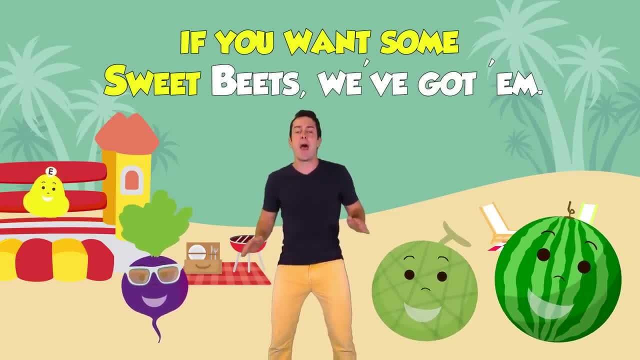 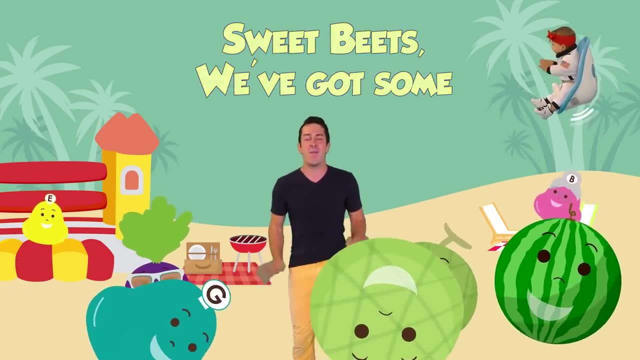 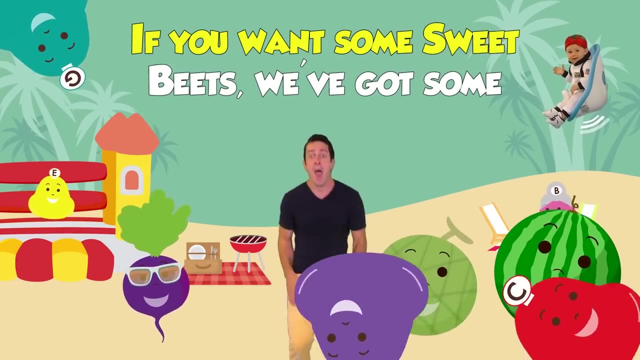 And if you want some sweet beets, oh, we've got them. Let's stomp those beets as we tap ready set Sweet beets- oh, we've got some. And if you want some sweet beets, we've got them. And if you want some sweet beets, oh, we've got some. And if you want some sweet beets, oh, we've got them. 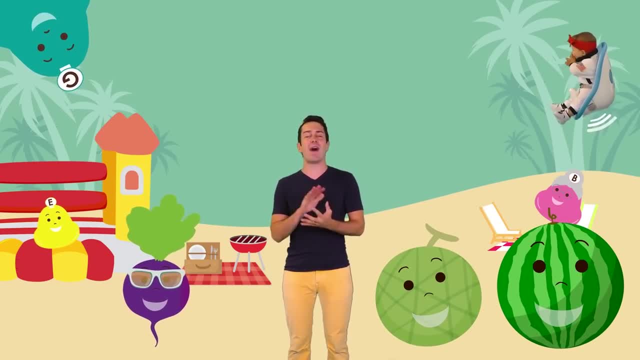 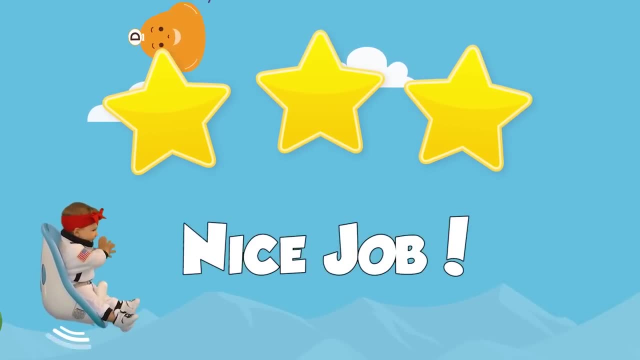 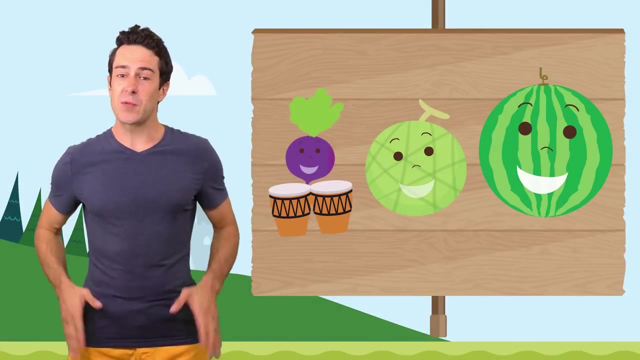 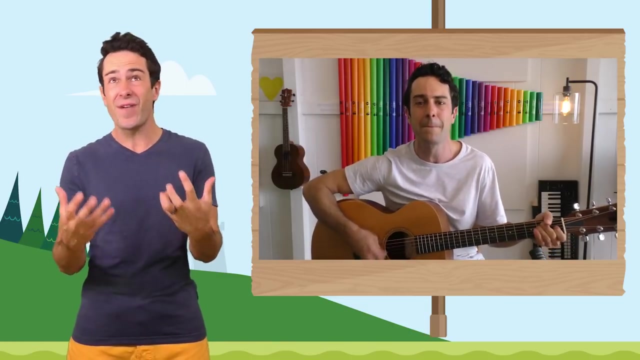 Give yourself a huge round of applause. Excellent job playing Sweet Beets with Beet Melon and Watermelon. everybody, You've been doing such a great job practicing with Sweet Beets and with the SoulFedge hand signs. So why don't we take a little break? head over to the studio and we'll sing a super fun and silly song by Yvonne Aultz called Fire Truck. 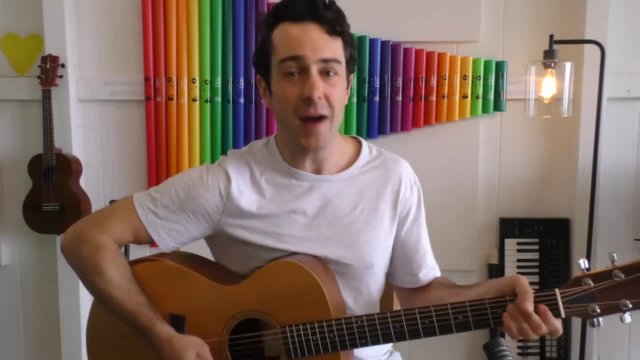 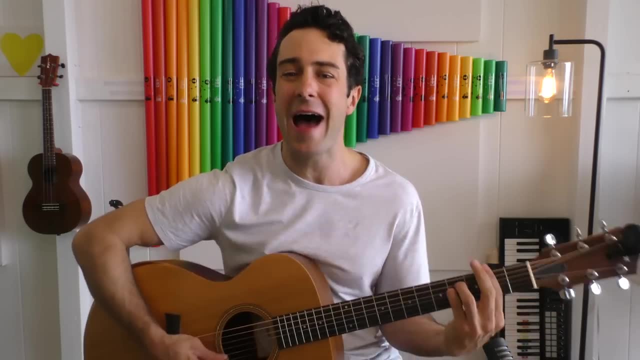 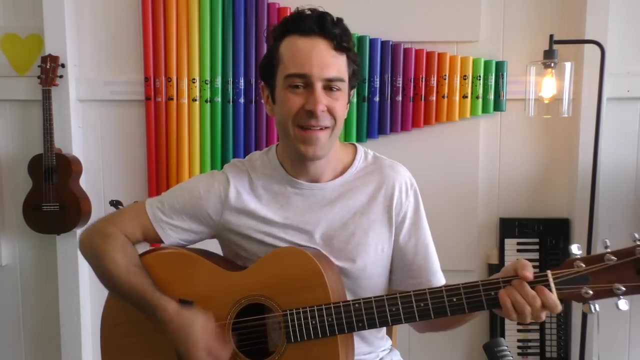 The main part of the song goes: Fire Truck, Fire truck, Fire truck. You sing Fire truck, Fire truck. And then I want to ride on a fire truck. You try, I want to ride on a firetruck. Um Yeah, that's it, I'm just a little bit faster. 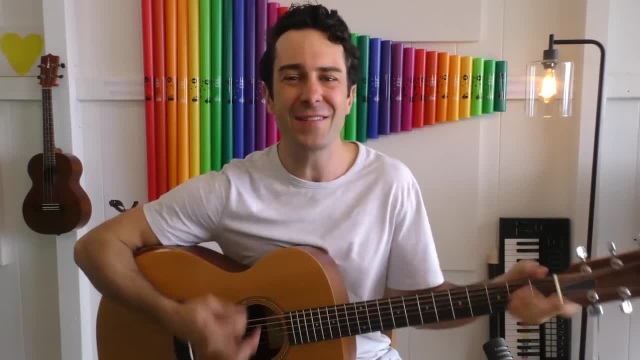 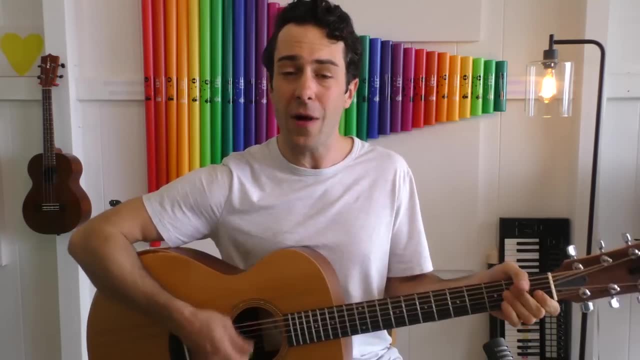 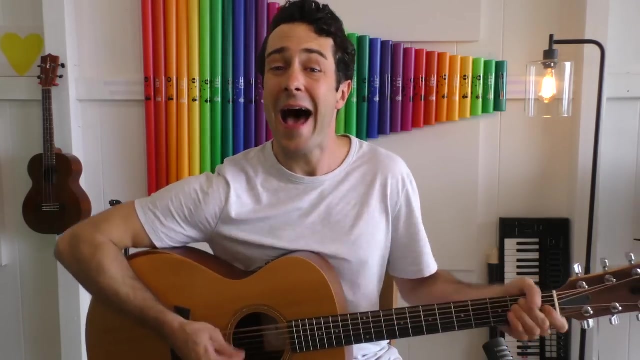 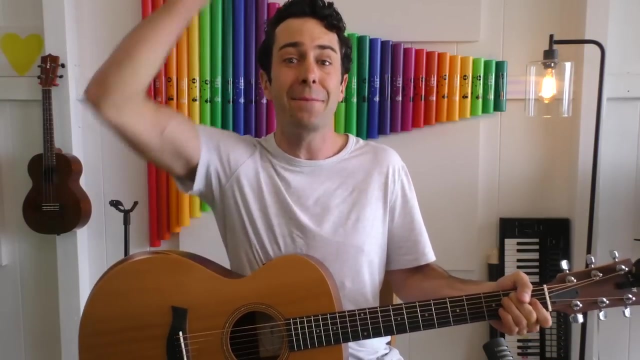 Here we go. Fire truck, Firetruck. I want to ride on a firetruck, Firetruck, Firetruck. Well, I want to ride on a fire truck. Well, I want to sleep at the fire station. Wake me up when the fire bell rings. I'm gonna put on my hat and put on my coat. 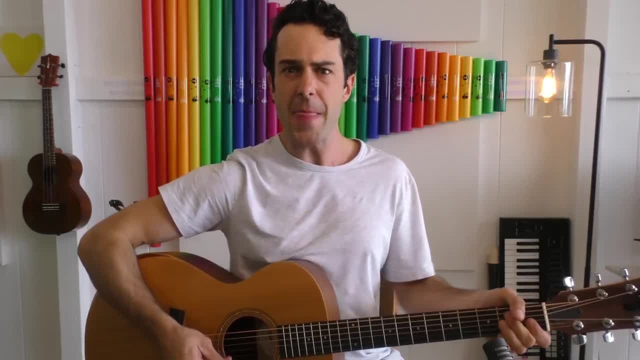 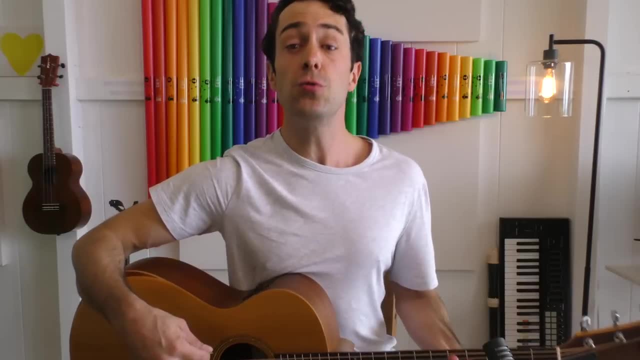 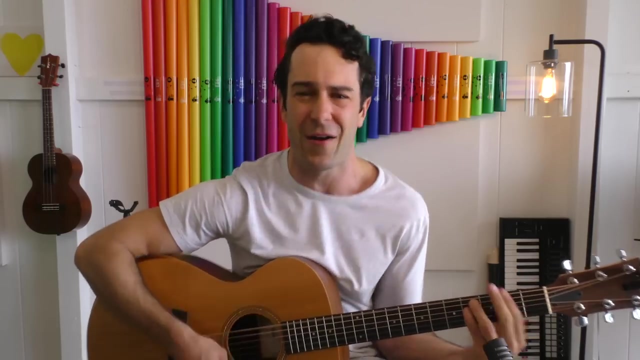 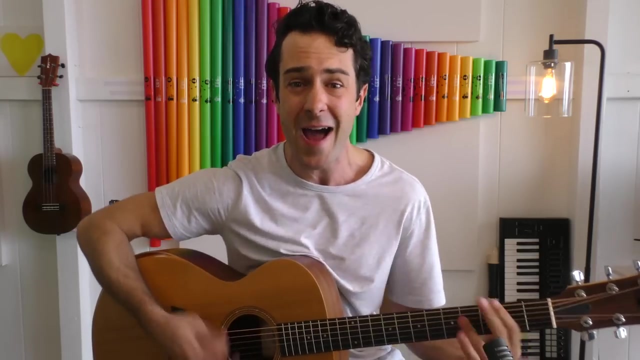 I'll put on my boots, I'm gonna slide down a pole, And then we say a-wee, And then I'm gonna get into my Fire truck, fire truck. I want to ride on a fire truck, Fire truck, fire truck. Well, I want to ride on a fire truck. 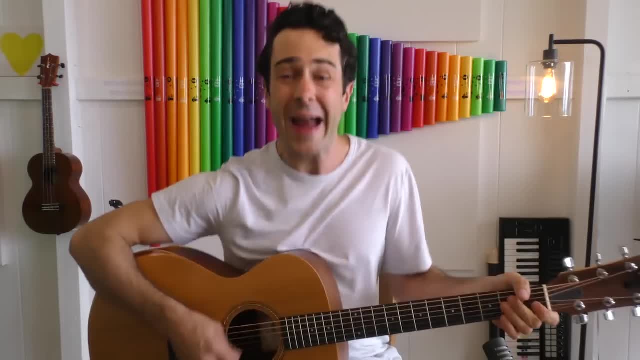 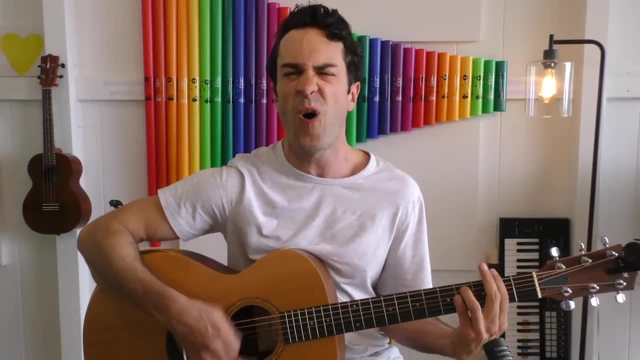 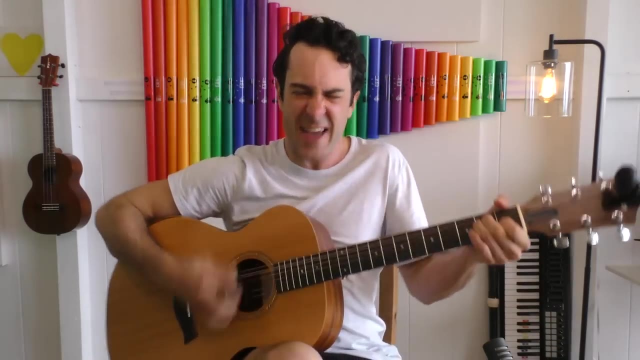 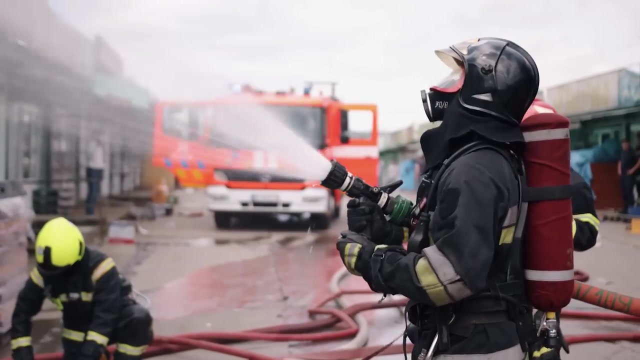 I've got a hook and ladder. a hook and ladder. I climb that ladder and I hold on tight. Alright, get out your hose. I'm gonna get out my hose And I'm gonna shoot that water. Shoot that water. Shoot that water from the hose on my 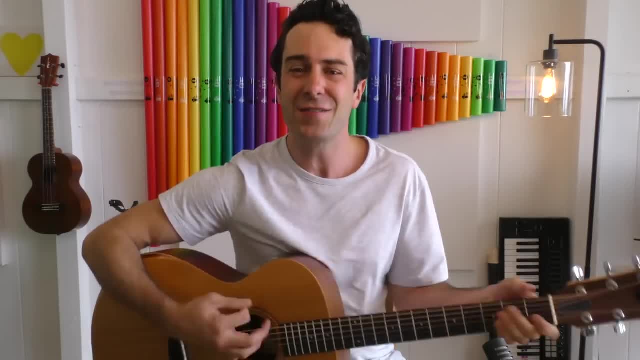 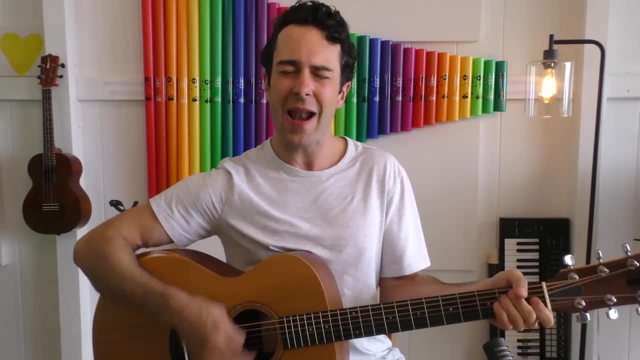 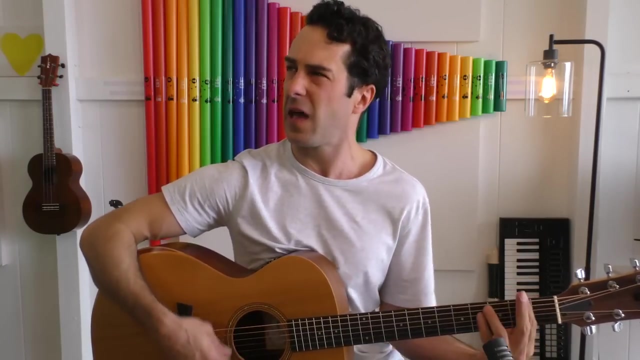 Ready Fire truck, fire truck. I want to ride on a fire truck, Fire truck, fire truck. Well, I want to ride on a fire truck. What does a fire truck sound like? I'll be-wee-wee-wee, I'll be-wee-wee-wee. 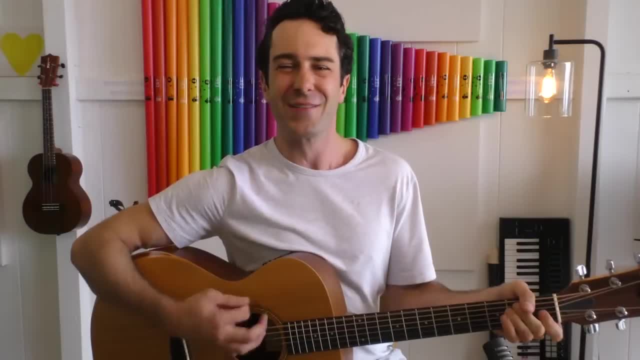 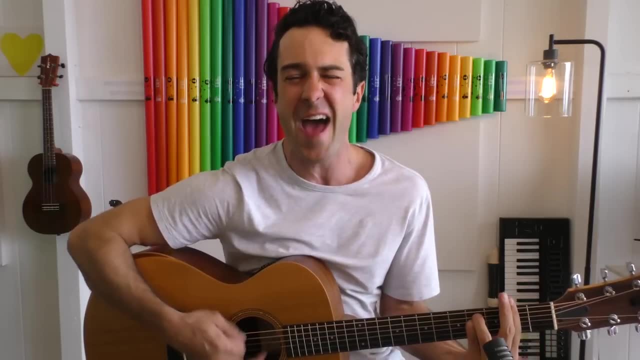 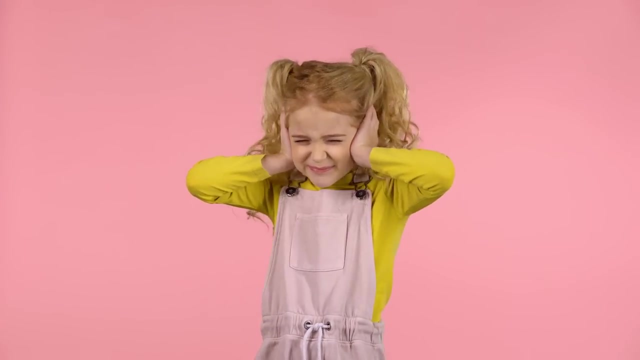 I'll be-wee-wee-wee Cause when that fire truck comes near. Alright, cover your ears. The people put their hands right over their ears, And they do that because the siren is so loud On Power. What does a fire truck sound like? 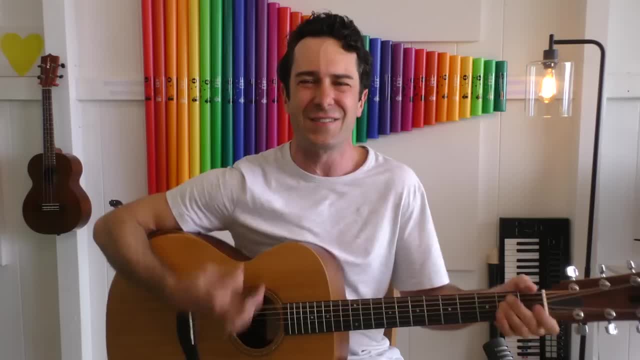 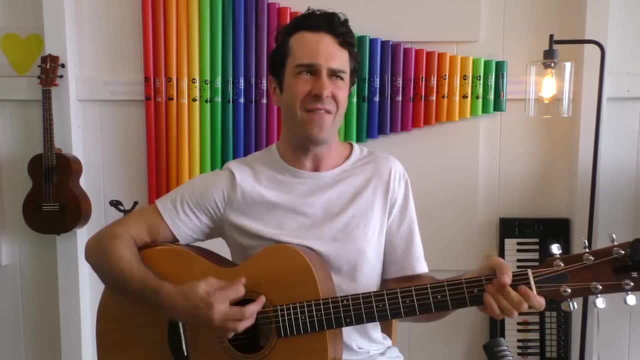 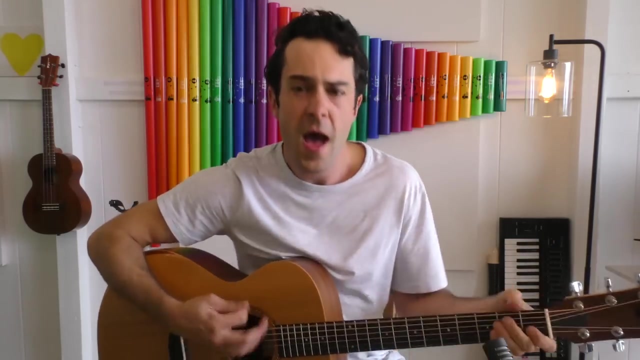 I'm gonna get out my hose, I'm gonna get into my hose. Fire truck, fire truck. I want to ride on a fire truck, fire truck, yeah, fire truck, I want to ride on a fire truck, Alright. so we got out our hoses and we sprayed down the fire. What happens to it? Yeah, it goes out Nice job. So when that fire is all put out, I'm going to jump into my fire truck and turn it around. I'm going to go back to the fire station and have a hot, hot bath. 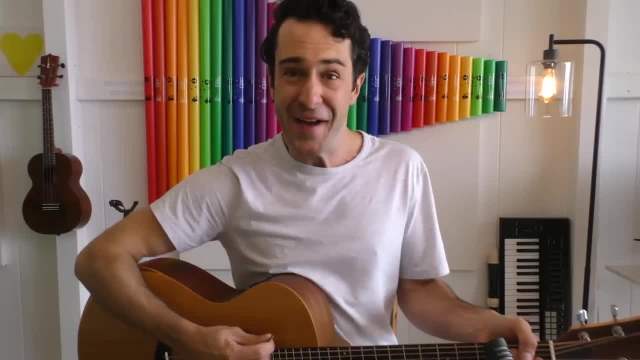 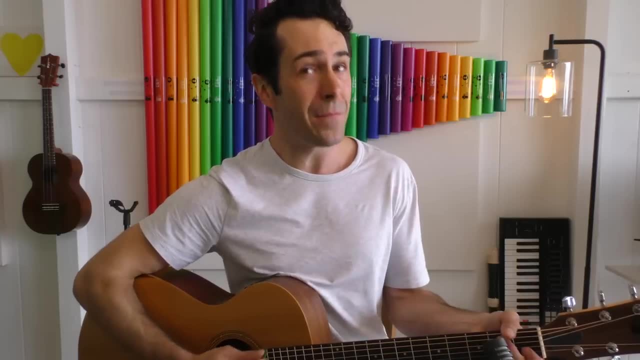 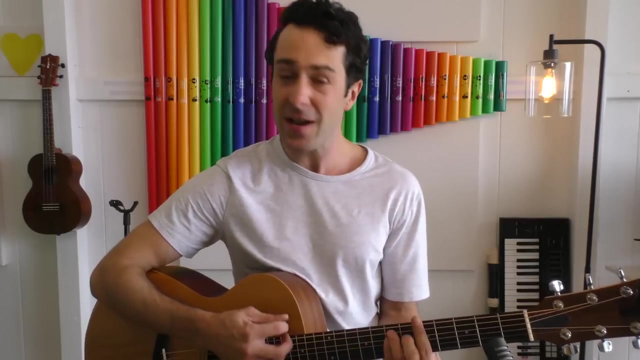 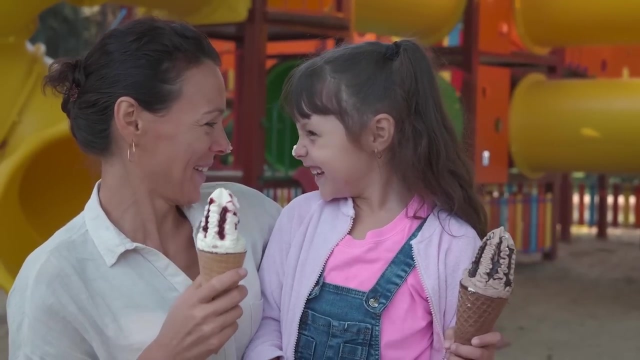 And some hot hot dinner, Yummy. And some hot hot food like hot hot chicken Or hot hot macaroni and cheese, With some sweet tomatoes and lima beans and broccoli. And for dessert I'm going to have some cold, cold ice cream. 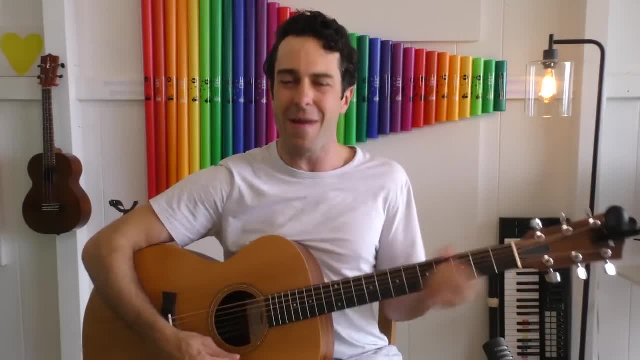 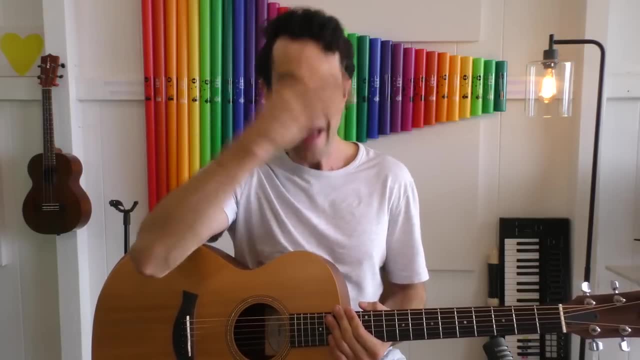 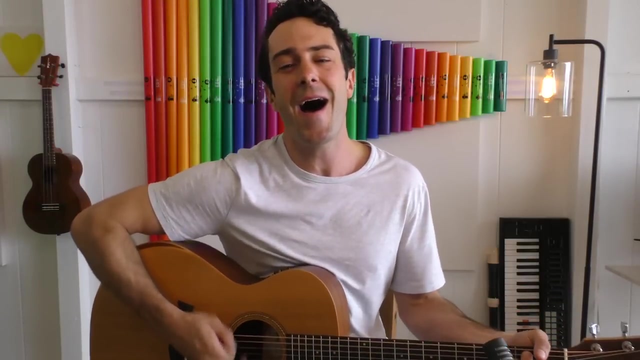 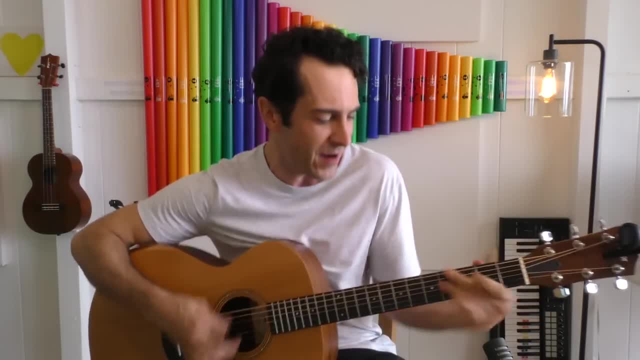 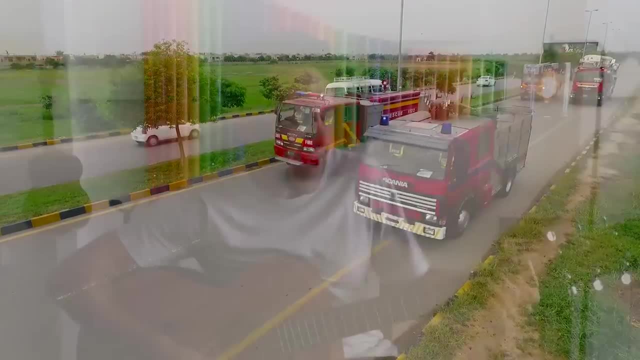 Fire truck. Well, I want to ride on a fire truck. Really loud Fire truck. Woo, Fire truck. Yeah, I want to ride on a fire truck. Fire truck, Fire truck. Well, I want to ride on a fire truck. 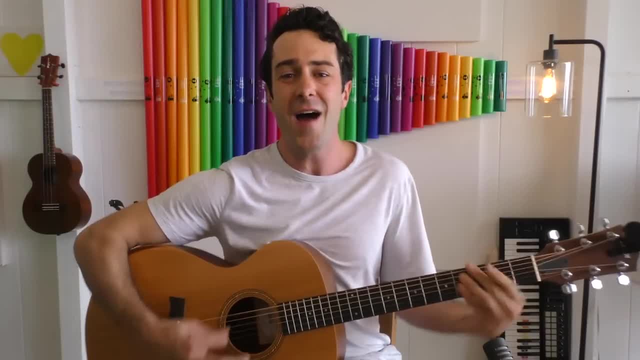 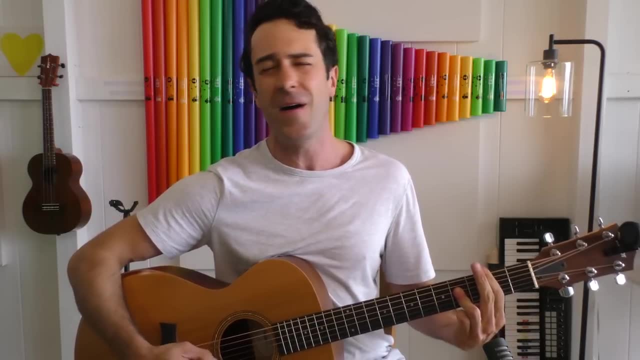 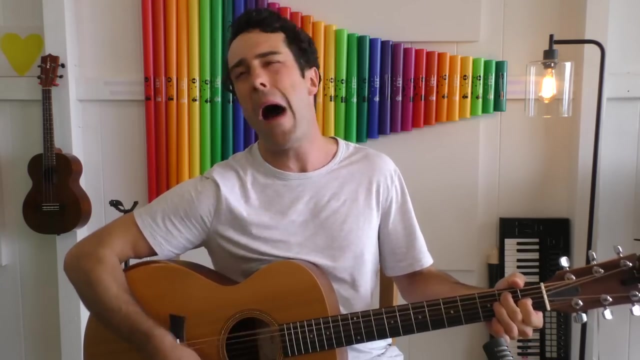 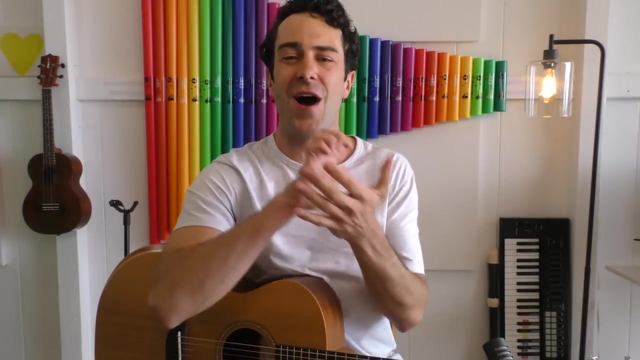 Last one: Fire truck, Fire truck. Well, I want to ride on a fire truck. I want to ride on a fire truck, A fire truck. Give yourself a round of applause for singing along with the fire truck song. everybody, Nice job with that one. 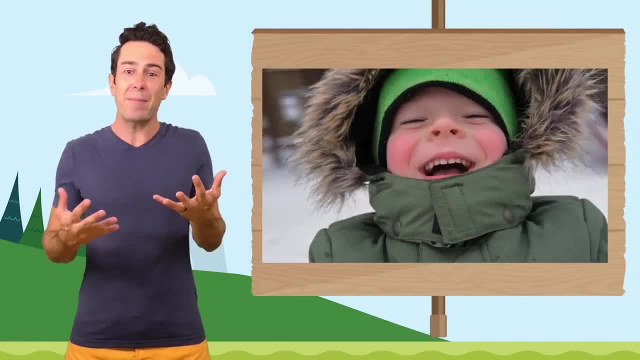 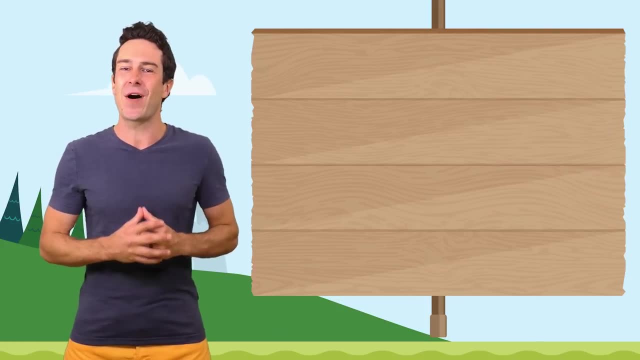 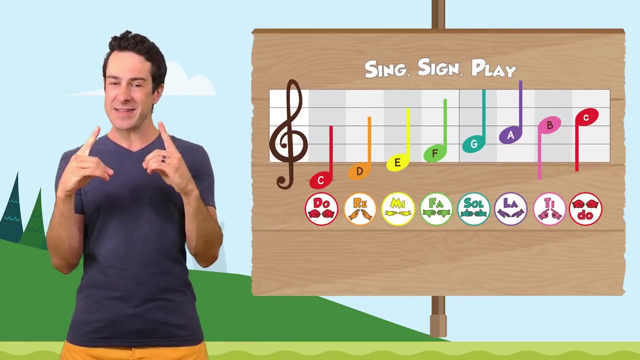 Playing that fire truck song always makes me feel really happy and really upbeat and energized and ready. So I hope that you are feeling good. So I hope that you are feeling good after singing that fun little song together. The different musical notes: Do Re, Mi, Fa, Sol, La, Ti and Do. 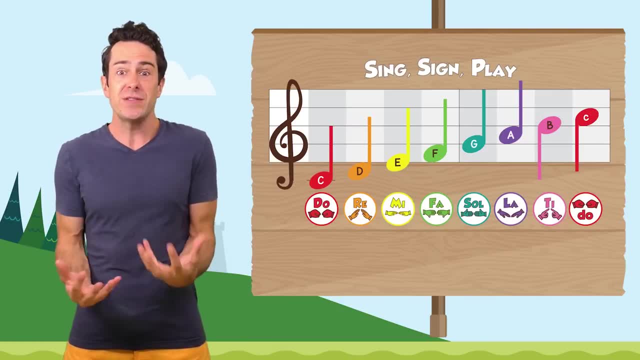 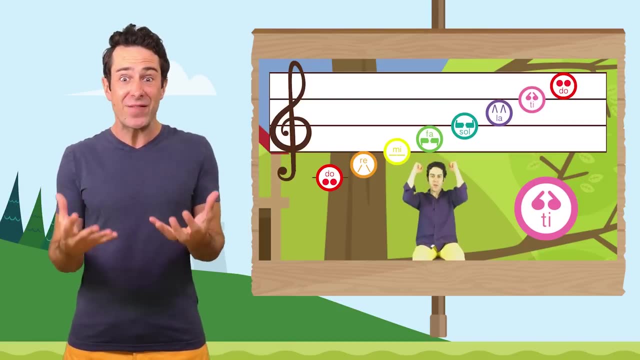 All have a different feeling that they can give us when they're used in our music. And in this next lesson we're going to practice some more with those hand signs and learn all about the different feelings that these hand signs and these musical notes can give us. 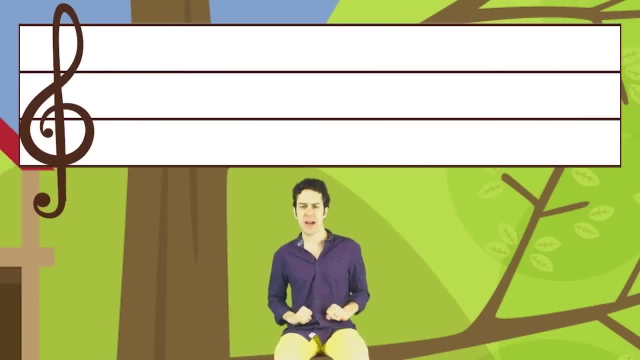 So the Kerwin hand signs start out down here We're two little hands, Two little fists, kind of by your waist, And we like to sing. Do You try, Do Again, Do, Do, Nice job. Then we go from that strong Do to a rising tone. 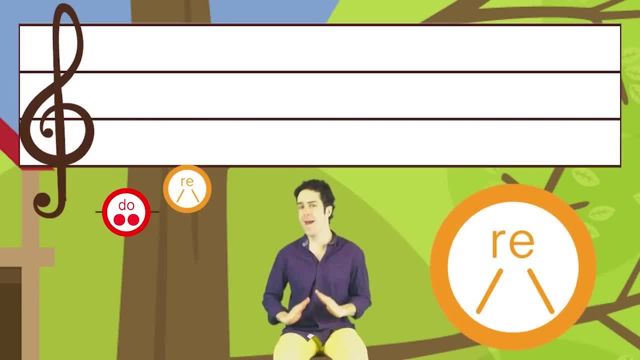 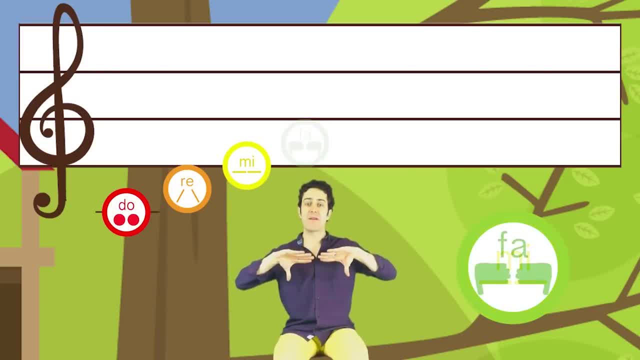 Mi, Mi Mi. The flat hands are nice because it shows us that Mi is sort of a restful tone or a peaceful tone. Then we do a thumbs down for the inspiring tone. Fa Fa, You sing Fa Yeah. 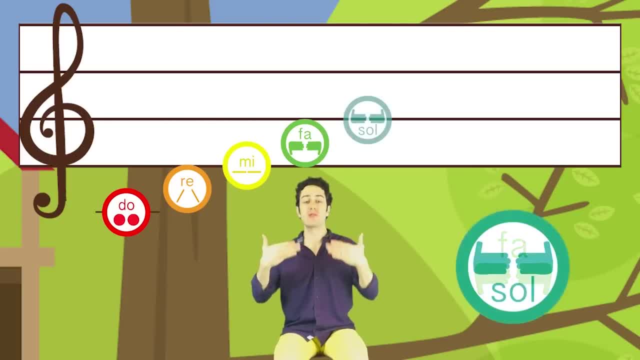 Fa. Thumbs down for Fa, Thumbs up for Sol. You sing Sol. Yeah, Sol, Sol, Sol, Sol. Sol is the grand tone or the bright tone. Then we go from sol up to la. Can you sing la again? 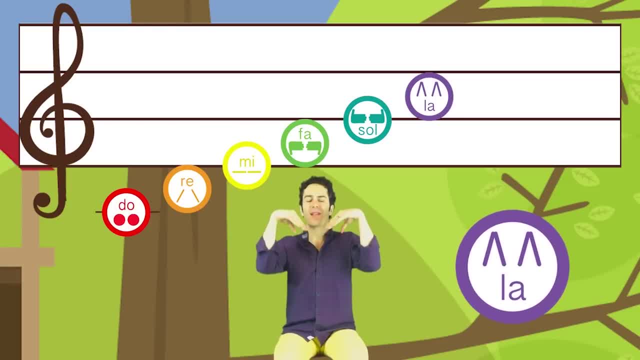 La la La is kind of the sad or the weeping tone and if you put your hands up here and just go like that, they will fall right into la From la. we keep on going up like this: to ti Ti, you sing ti again, ti ti. 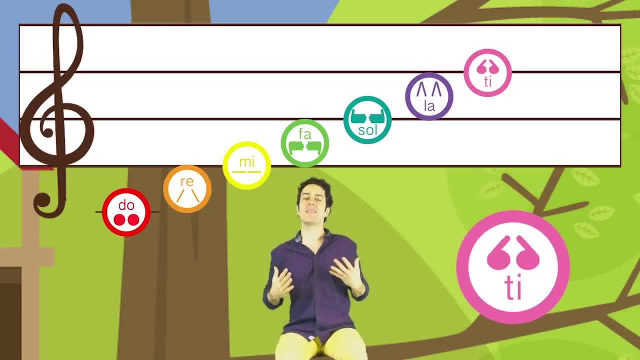 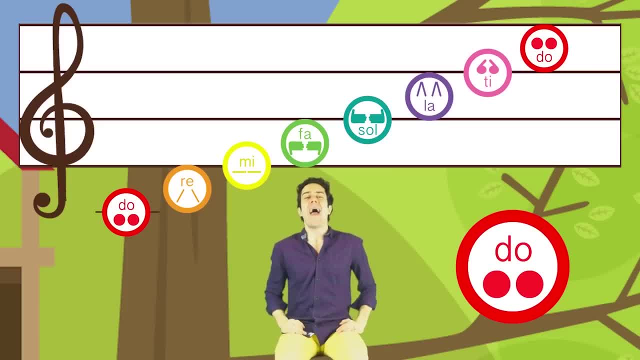 Do, do, Hey, nice job. So those are all the hand signs. Let's just talk about that. ti, real quick, Ti. it's kind of like two little balls pointing up, kind of showing us that we're gonna go up into the do. 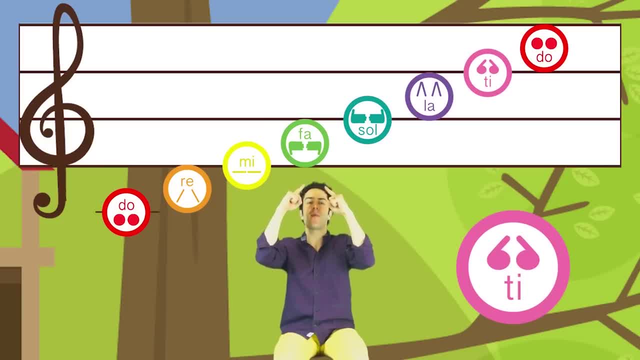 Some people like to put their fingers like this, but either way, if you got a little ball and you're pointing up, that's your ti, up to your high do. So we started out with do and we ended with do, and that's because the musical notes 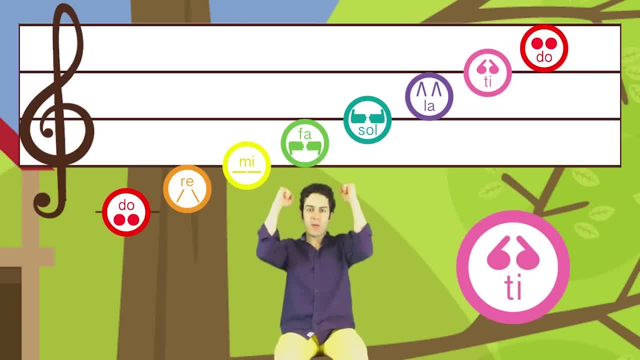 always repeat in a pattern. We start with do, we end with do. we can sing some higher notes. We'll have re higher than that high do or notes even lower. Let's try it real quick. Let's try a really low. 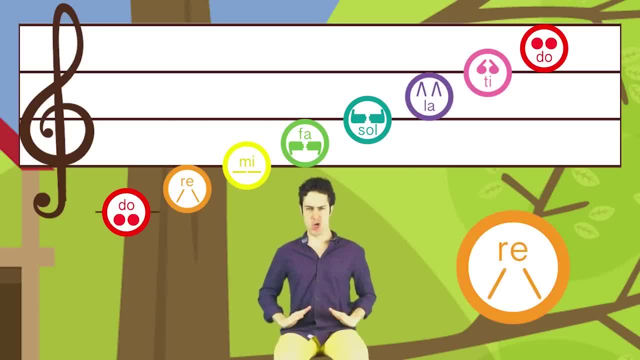 Do up to a really low. re mi fa sol la ti do. That do is where we actually started before. Do re mi fa sol la ti. do re mi fa sol la ti do. 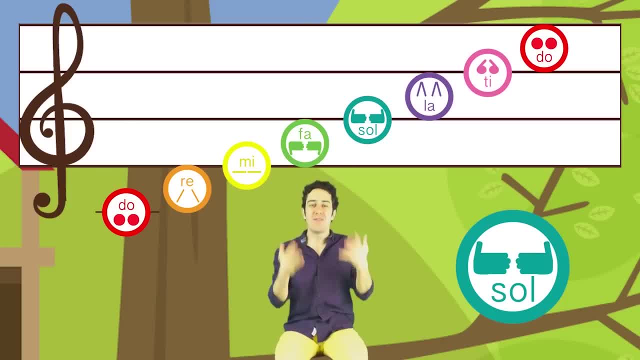 I can't really sing up that high but if you can, you can keep on going practicing the solfege up way, high, way down low and you can hear how that musical pattern repeats. I hope that helps with the solfege hand signs. 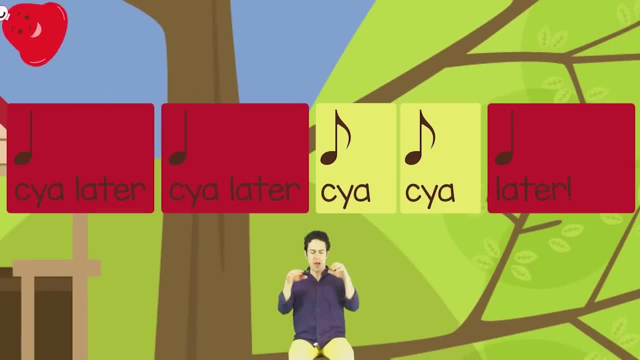 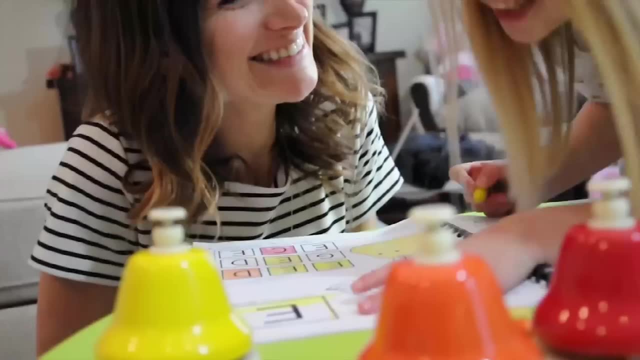 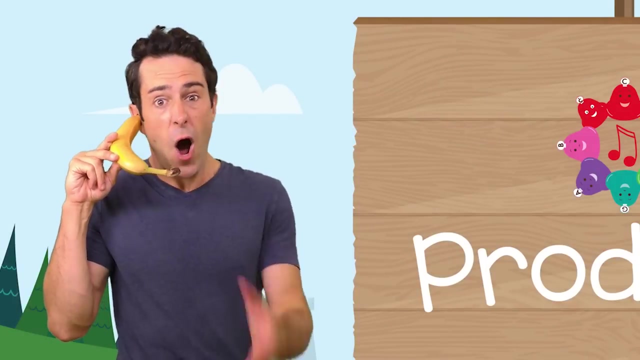 I hope you had a lot of fun and until next time, I will see ya later. see ya later. see ya, see ya later. Uh-huh, yup, that's awesome, but I've gotta go. I'm in the middle of a music lesson. 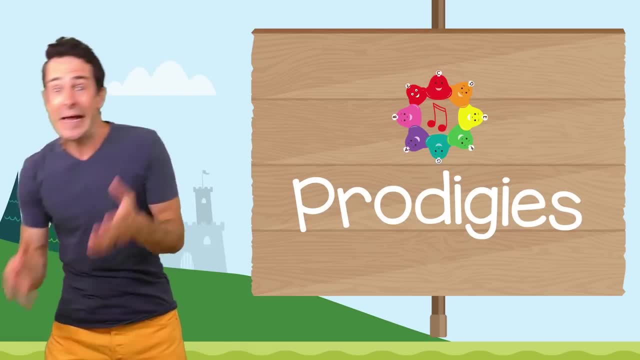 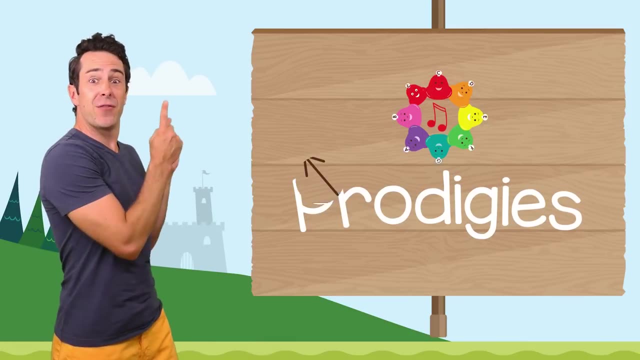 Yeah, right now. All right, bye, Sorry about that. We're gonna do some more practicing. Are you ready, Nice? In this one, we're gonna be looking at the treble clef and our solfege hand- signs that we've been learning. 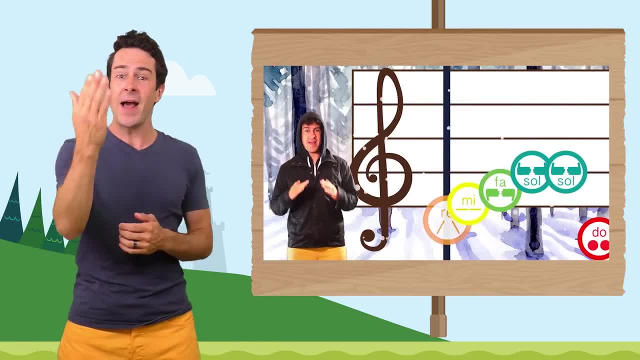 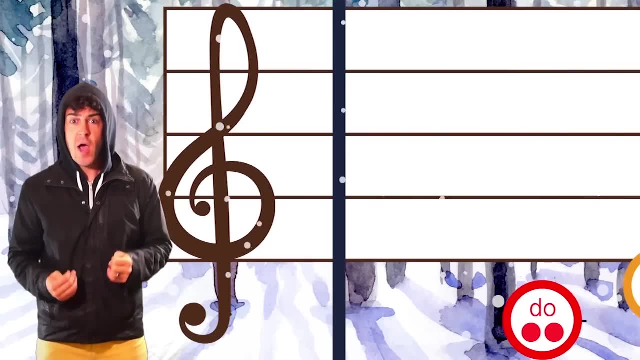 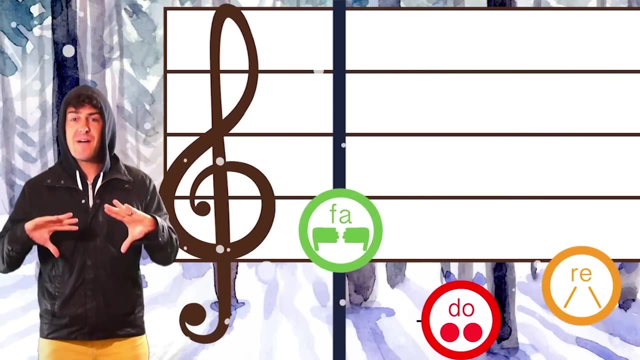 are gonna come this way, and when they hit the blue line, that's when you're gonna sing and hand sign. Are you ready? Let's hop into this short little exercise. Let's start out with: do Ready, Do re mi fa. you say. 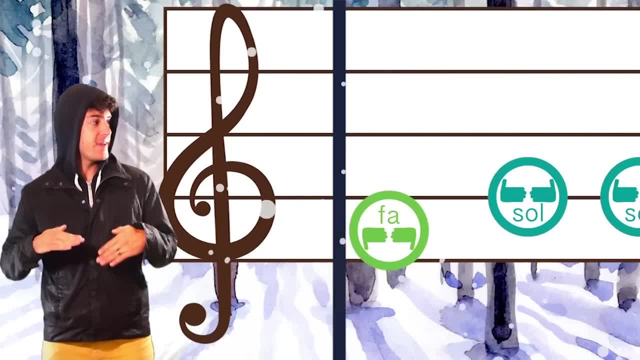 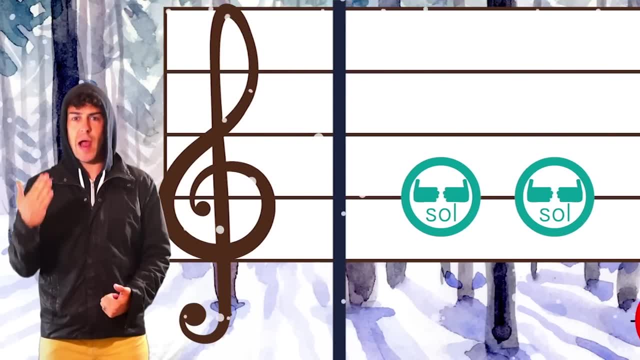 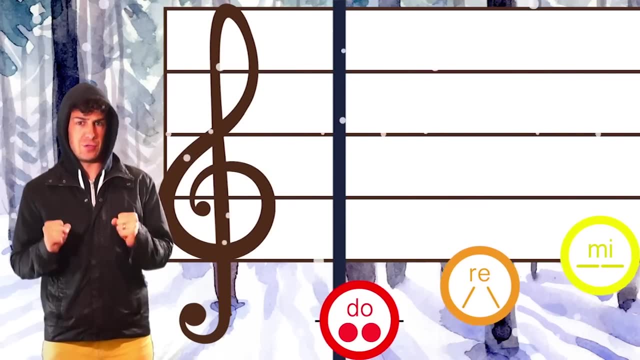 Do re mi fa. then we say sol sol down to do. You try it ready. Go, Sol sol do. Hey, back to the beginning. Let's try. Do re mi fa, you say it. 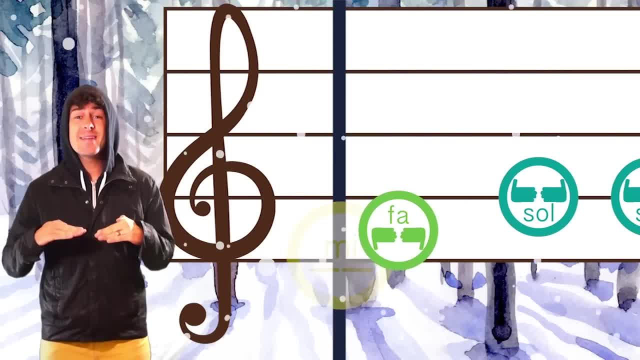 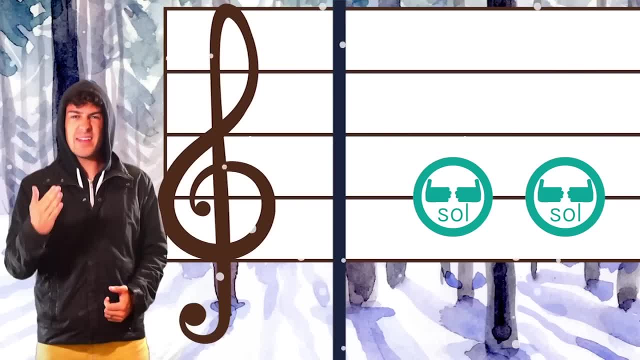 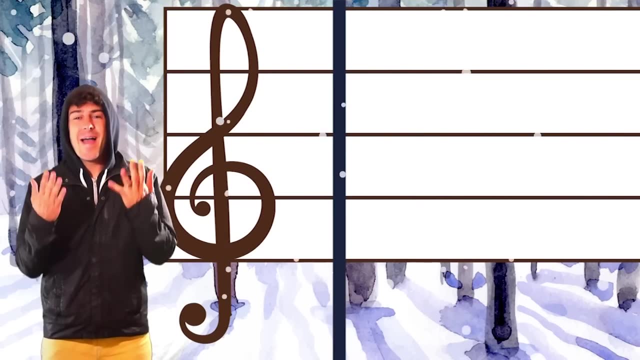 Do re mi fa. then hop to sol sol do. nice and loud. Sol sol do Hey. nice job with today's melody. Sounds nice and slow. Let's try it a little bit faster Ready. 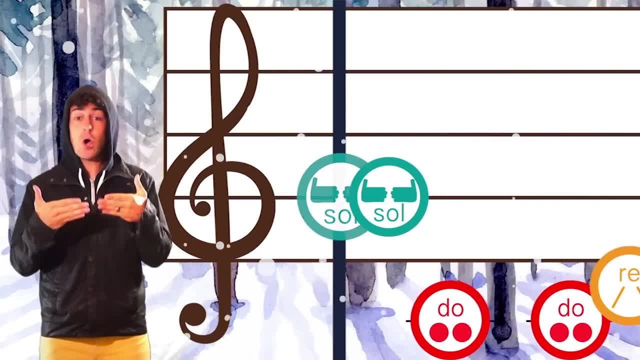 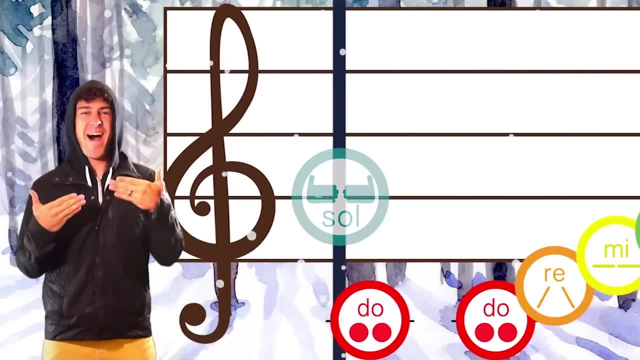 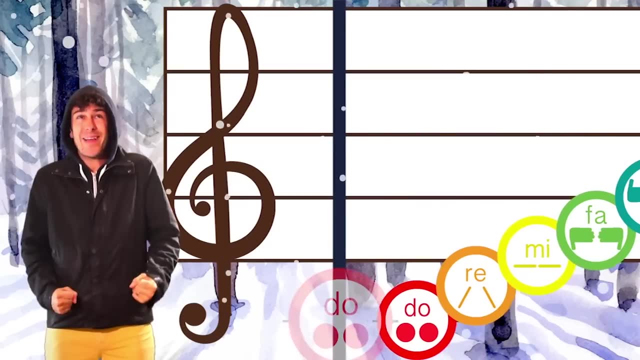 Set: do re mi fa sol sol, do you do it? Do re mi fa sol sol, do all together. Do re mi fa sol sol, do nice and loud. 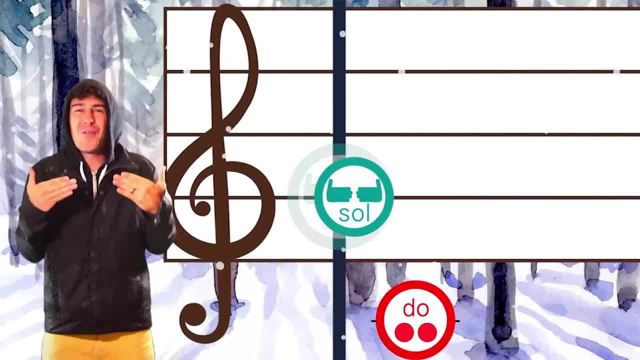 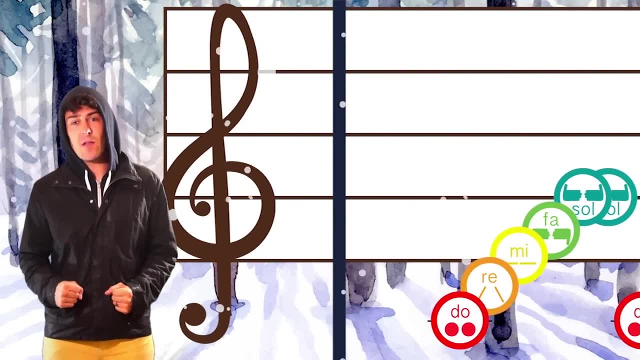 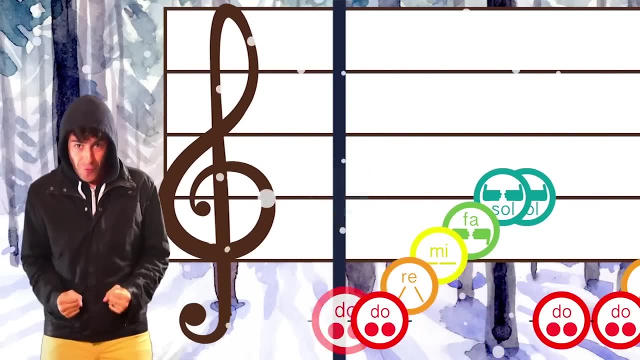 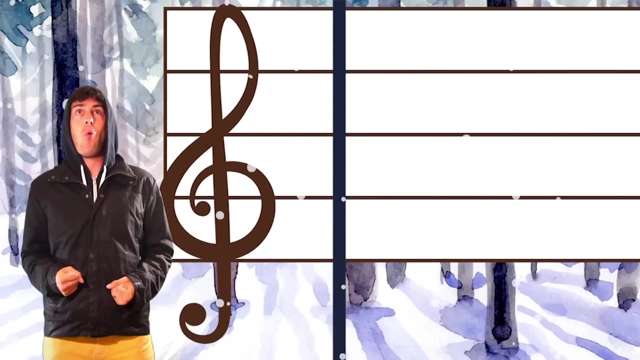 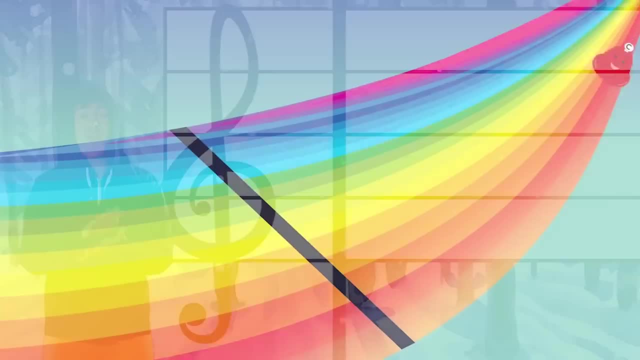 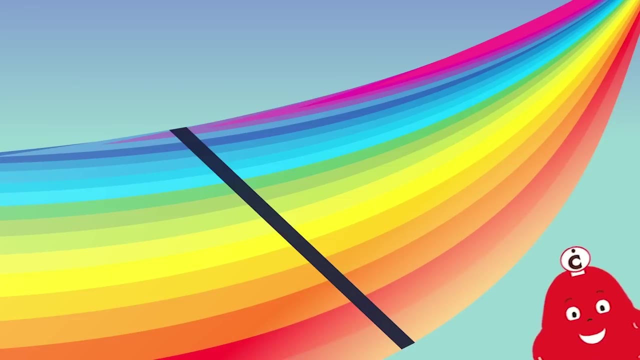 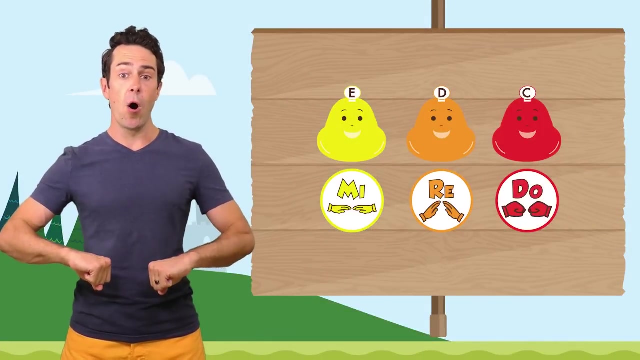 Hey, keepers have a huge round of applause. Nice job with today's episode of PSP Melodies. I love singing about the sol. I love singing about the solfege, like mi re do, But those words don't really mean anything. 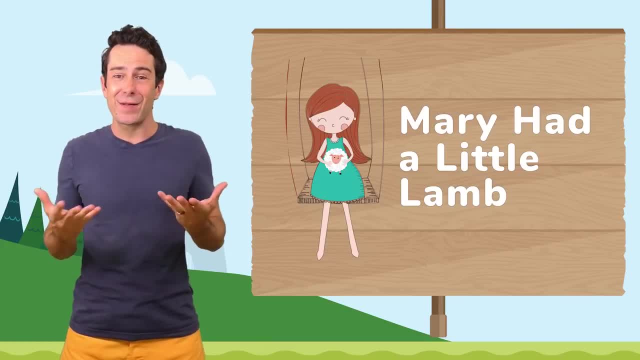 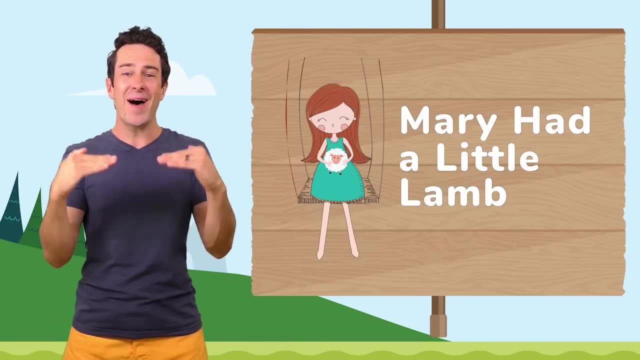 And in this next one we're going to sing Mary had a little lamb, by adding some of the words Mary had a little lamb to our solfege hand signs. We're going to sing about the solfege and the note names. 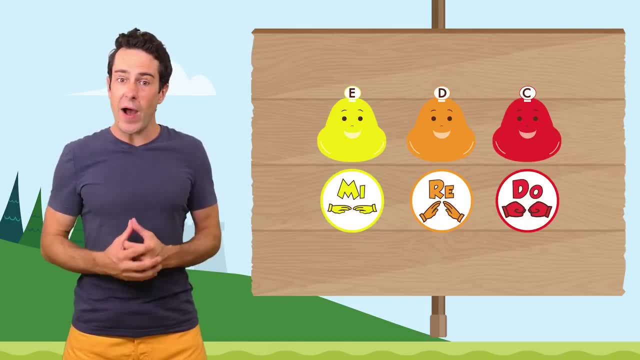 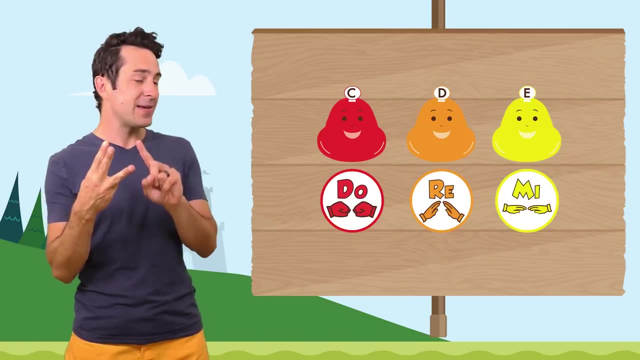 and the colors, And we're going to play our instruments as well. If you have an instrument, we need three notes: OK, C, D and E, red, orange and yellow, do re and mi. And if you don't have an instrument, 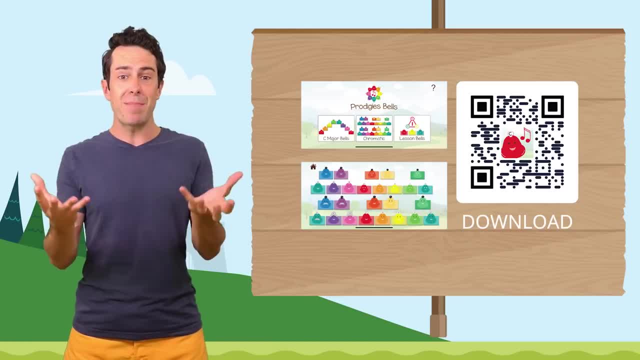 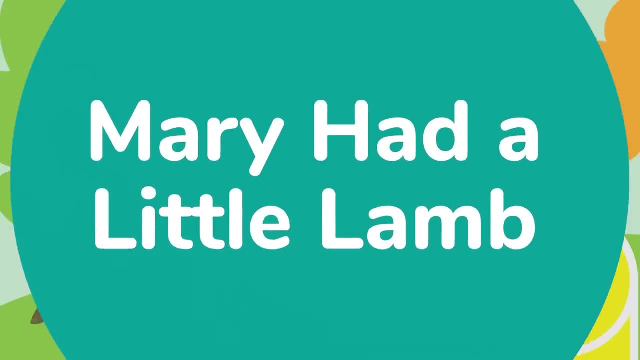 you can either download our free app Prodigy's Bells, or you can continue to sing and hand sign here in Mary Had a Little Lamb. We're going to start by singing and playing about the colors. We'll move on to the solfege. 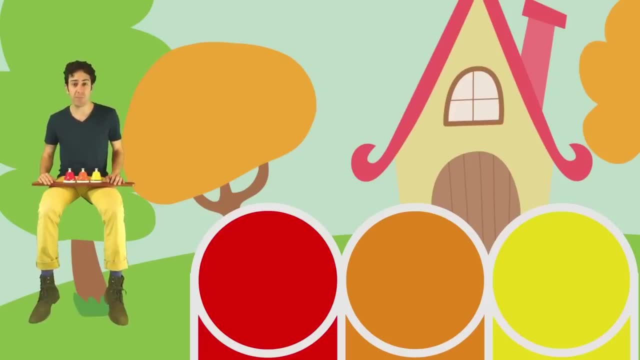 Then we'll practice some hand movements And then we'll finish up by singing the whole thing while we play our bells. So make sure your bells are set up like this. Here we go, One, two ready: Yellow, orange, red orange, yellow, yellow, yellow. 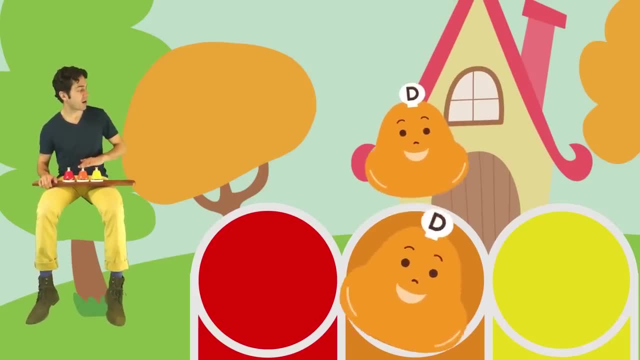 down to orange, orange, orange, orange. back to yellow, yellow, yellow, yellow. Great job. Yellow, Orange, red, orange, yellow, yellow, yellow. down to orange, Orange, orange, yellow, orange, red. 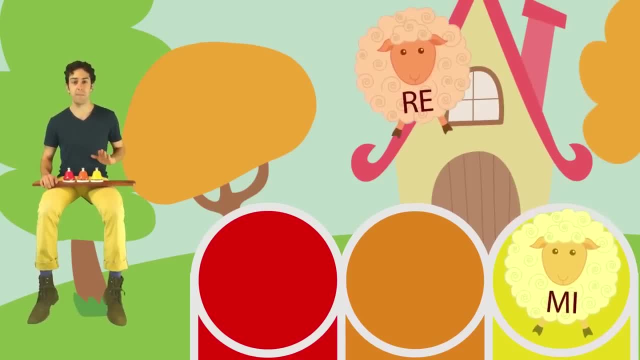 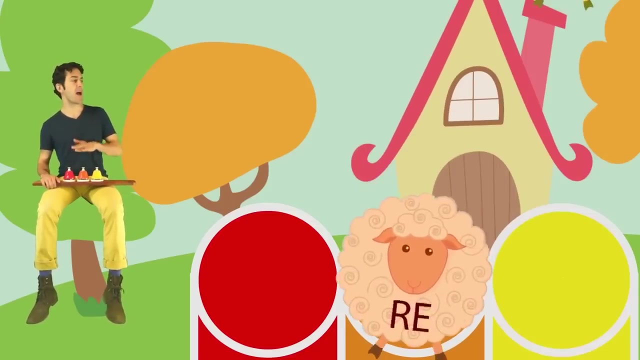 Nice job. All right, let's sing about the solfege: Mi re do re mi mi mi Nice and loud Re Re, re, re back to mi Mi mi mi nice. 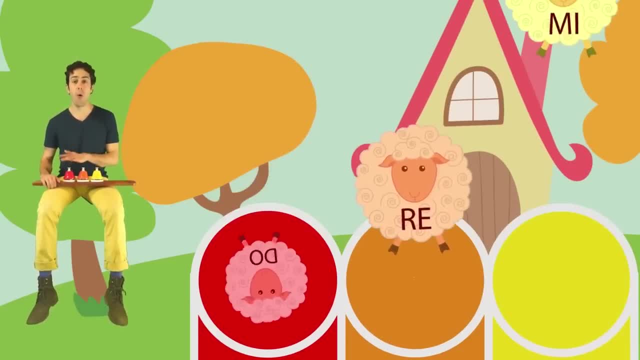 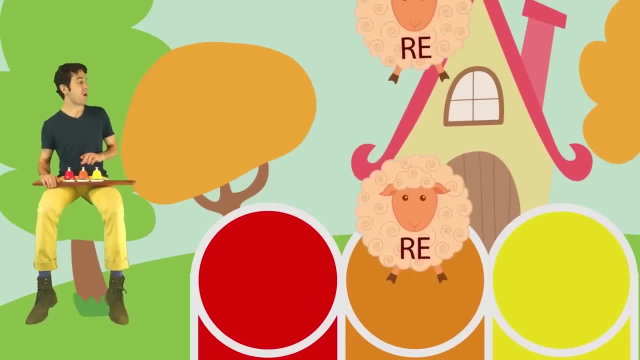 Mi re do re, mi, mi mi. down to re Re, re, mi, mi re, Re, re do. We're going to sing the same thing, but use our hand motion. Mi re, do re, mi, mi mi. 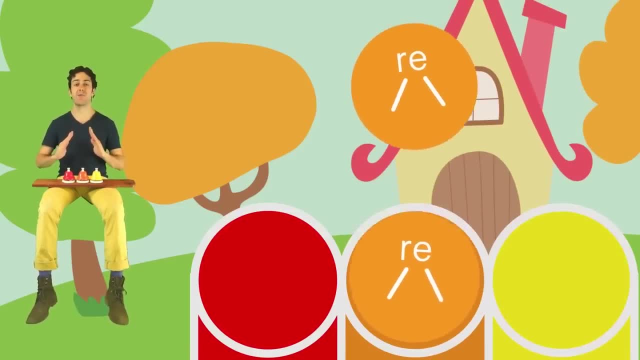 Let's go down to re, Re, re, re, back up to flat mi Mi mi mi. nice flat hand Mi Mi, Ray doh, ray me me me, Ray, ray me, ray doh. 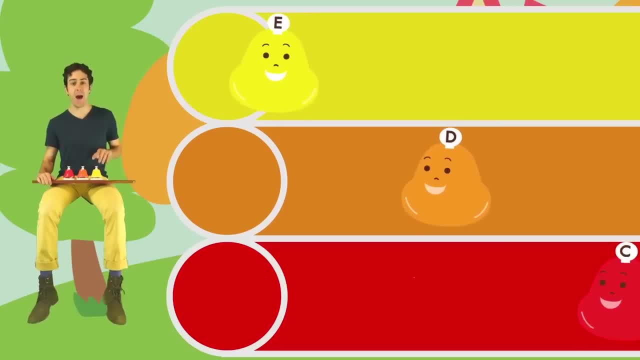 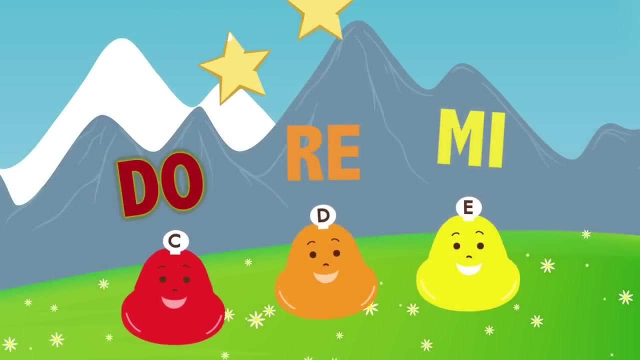 Nice job. Now we're going to sing the words and play. Mary had a little lamb, Little lamb, Little lamb. Mary had a little lamb, Little lamb, Whose fleece was white as snow. Nice job, everybody. Give yourselves a big round of applause. Nice job playing. Mary Had a Little Lamb with Doh Ray and Me. 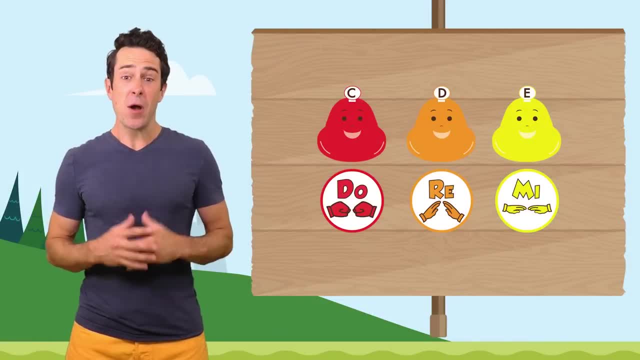 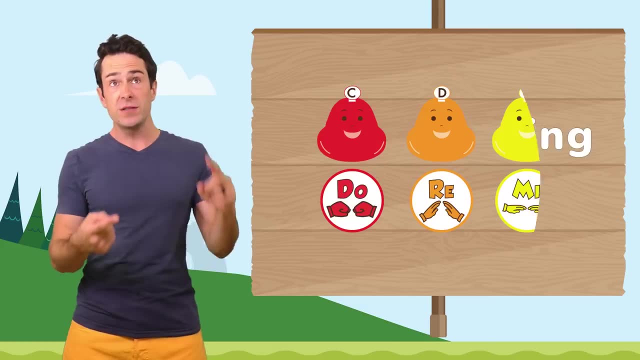 Nice job with Doh Ray. Me and Mary Had a Little Lamb. We've practiced a lot with these three notes, so now we're going to play a little listening game and see if you can figure out with the notes Doh Ray and Me, C, D and E, Red, Orange and Yellow. 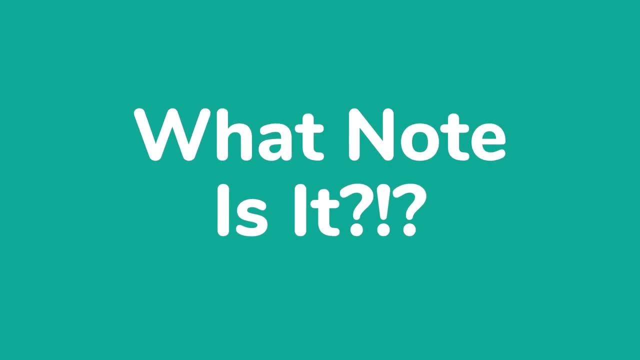 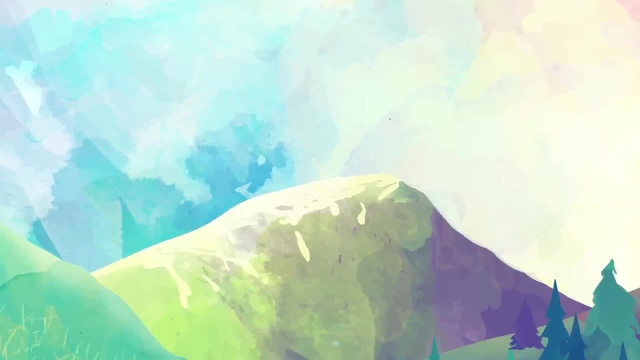 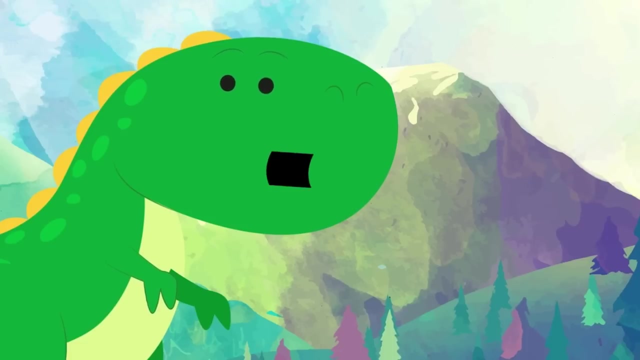 What note is it? And now it's time for another episode of everyone's favorite game show. What Note Is It With your host, this Tyrannosaurus Rex? Alright, kids, they're going to play a note And we're going to try and guess which one it is. 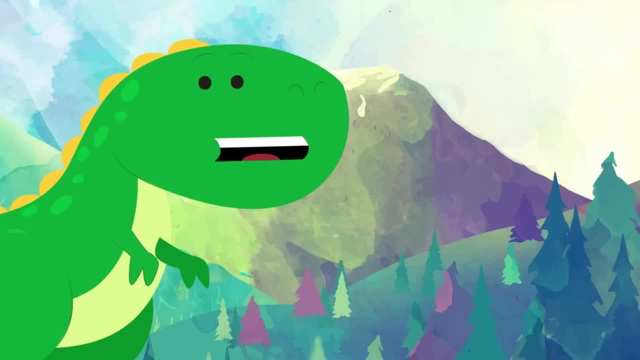 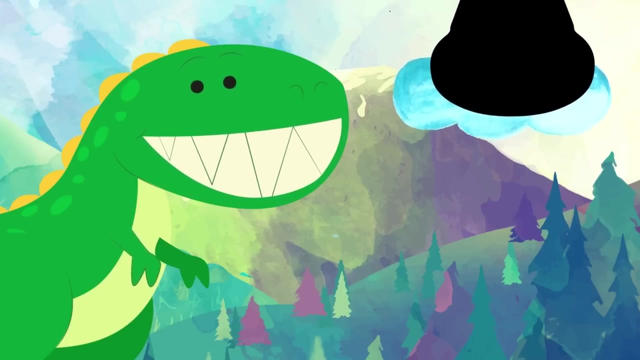 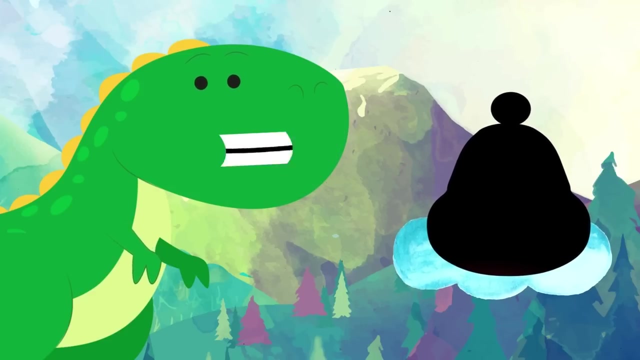 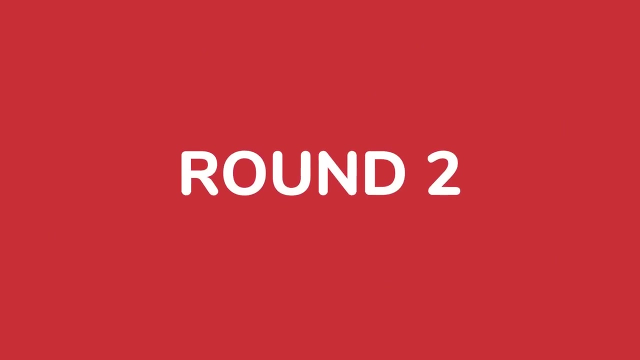 Are you ready? Today we're playing with C, D and E. Alright, listen up. What note is it? I think I've got it And the note is That's right. it's C. Alright, time for round two. 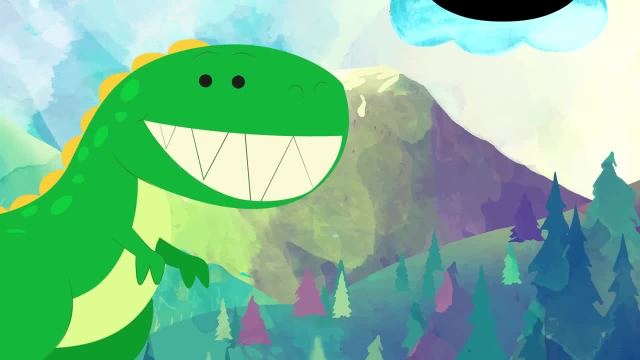 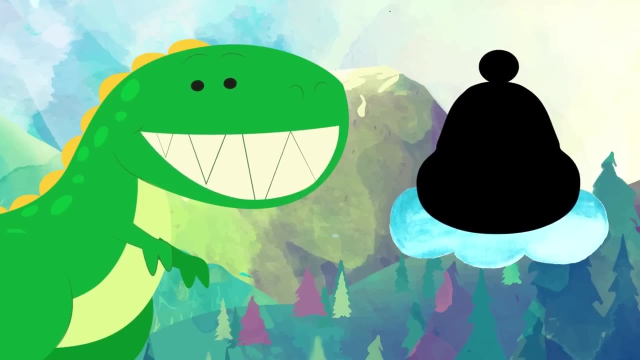 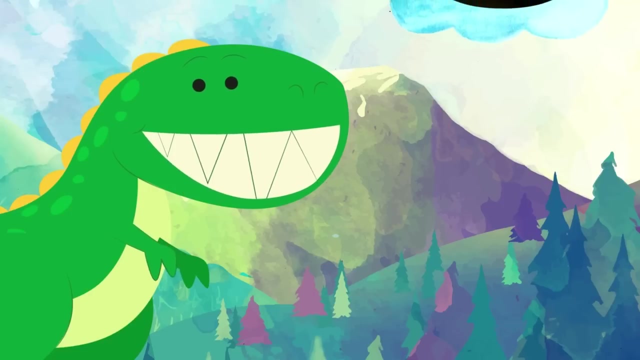 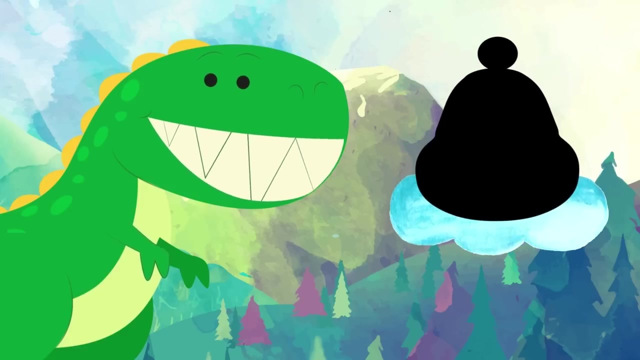 Let's see what it is. What could it be, Can you guess? And the note is: That's right. it's D Time for another round. Hmm, I wonder. This one's an easy one, And the note is: 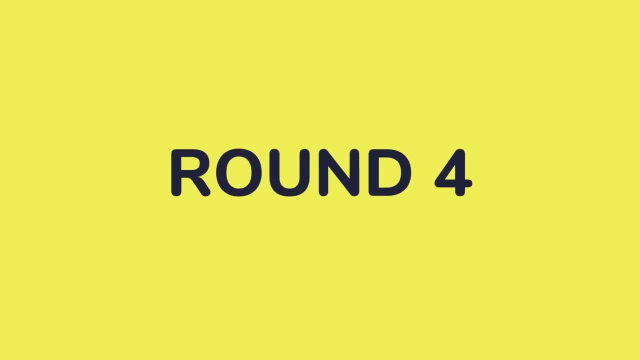 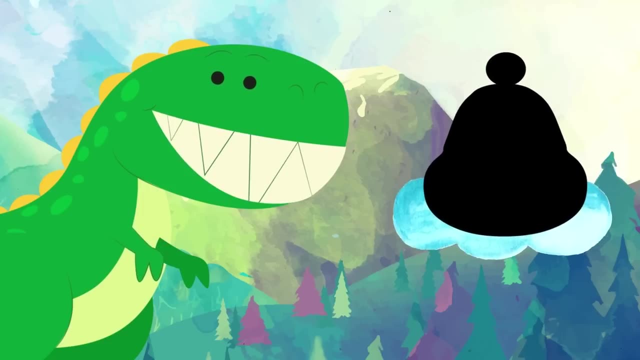 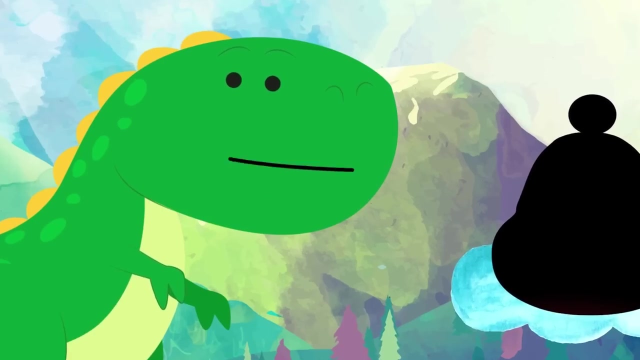 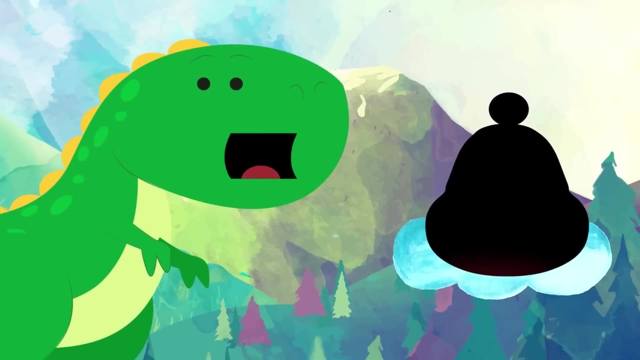 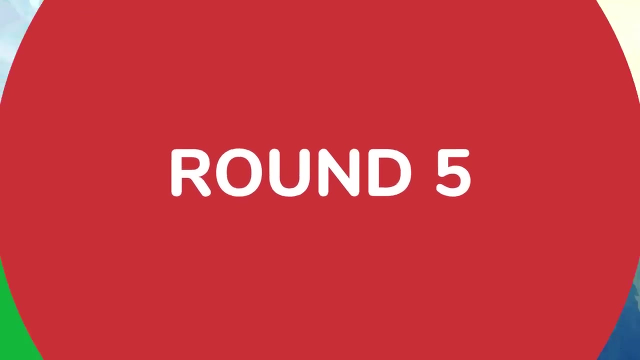 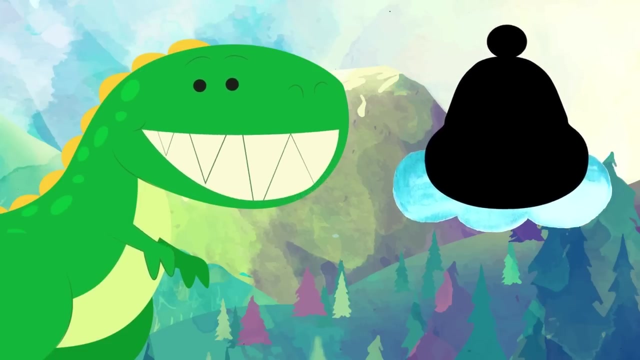 It was E or Me. Here comes another one. Which one is it? I knew I should have practiced And the note is It was C or D. Alright, what note is it? This one's a tough one. What do you think it is? 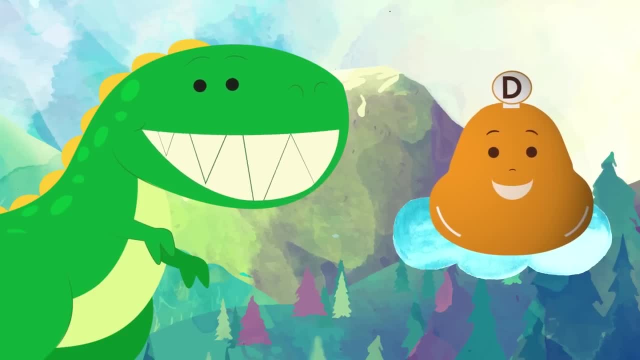 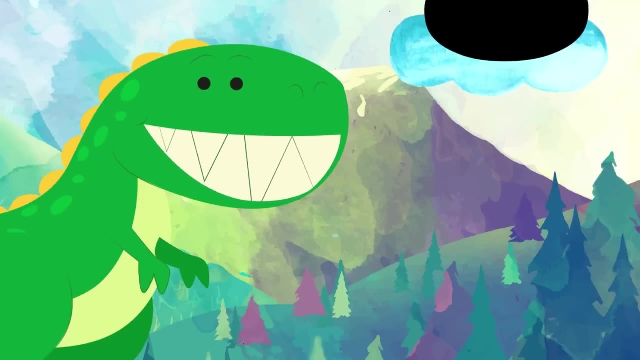 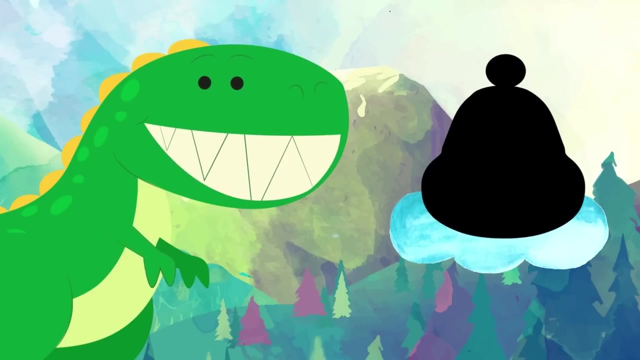 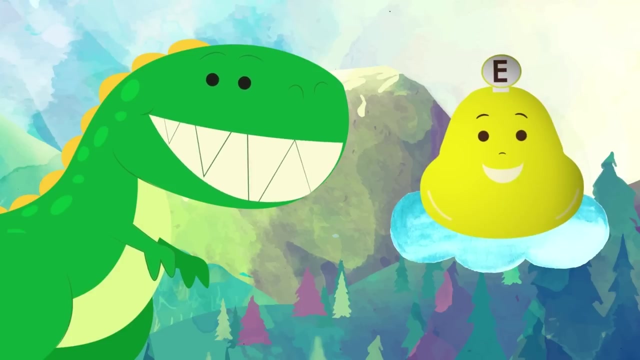 And the note is: It was D or Re. Now for the next round. What note is it? Can you guess? And the note is: And the note is: That's right, it's E. Have you been practicing? Let's see what the next one is. 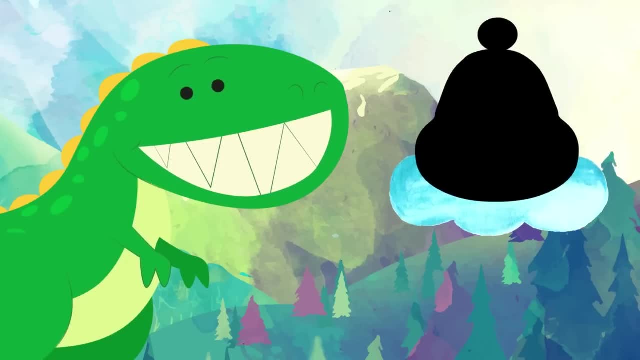 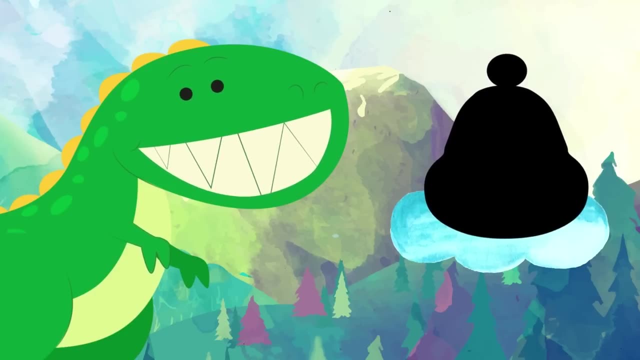 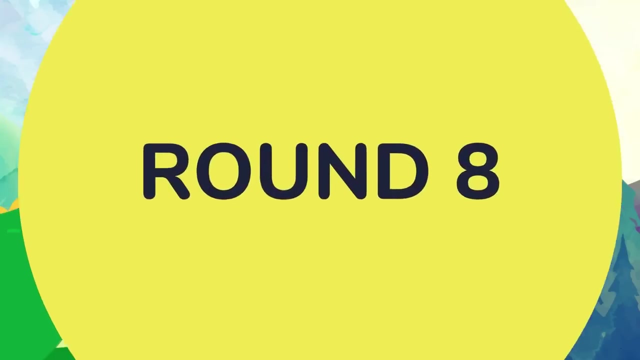 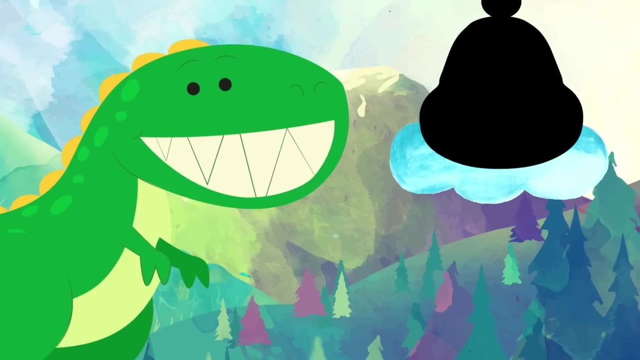 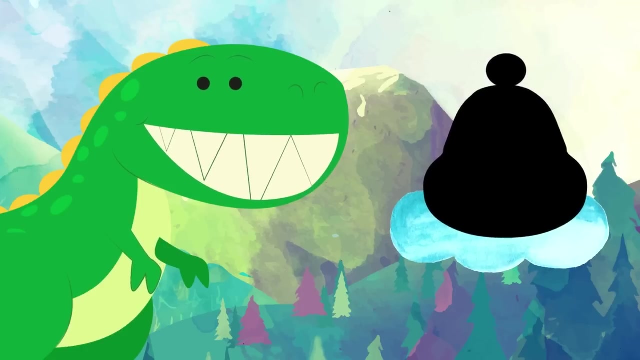 What note is it? Do you know it? And the note is. And the note is: That's right, it's E Great job. Let's try this next one. Any guess Which one is it? And the note is: 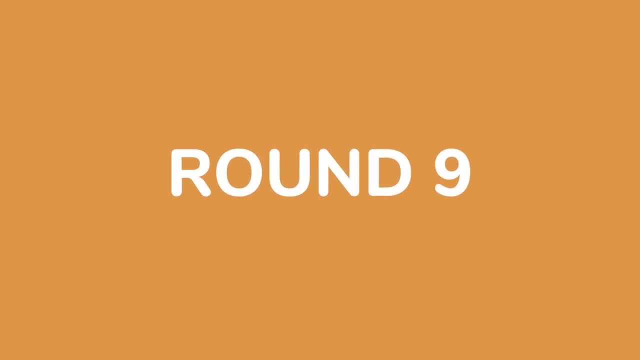 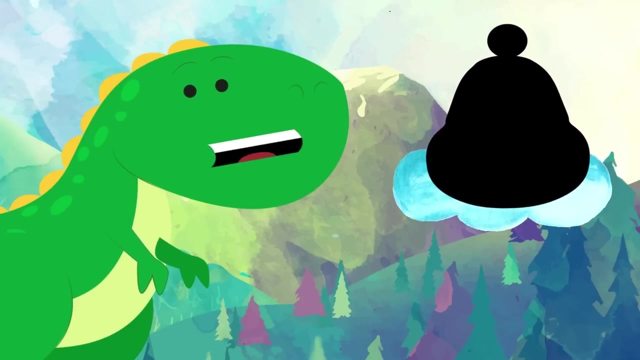 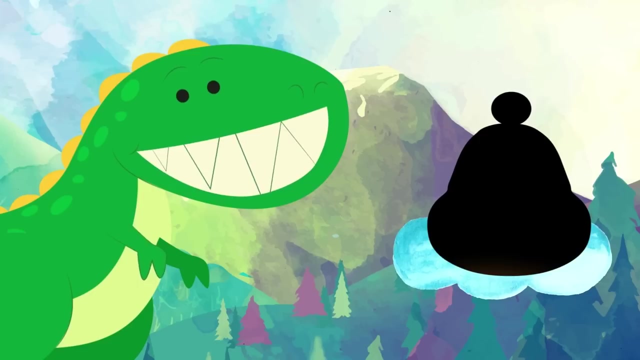 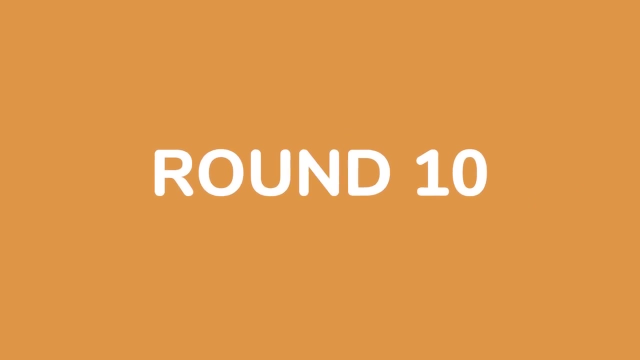 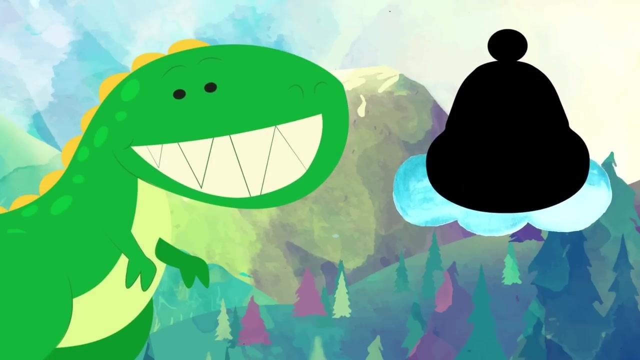 That's right, it's D. Let's see what comes next. What do you think it is? This one's a tough one, And the note is It was D or Re. Let's play again. What note is it? 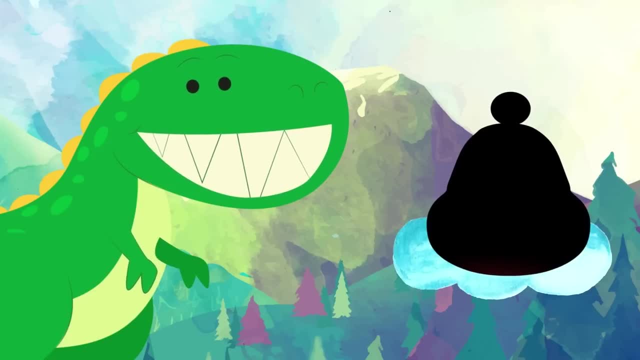 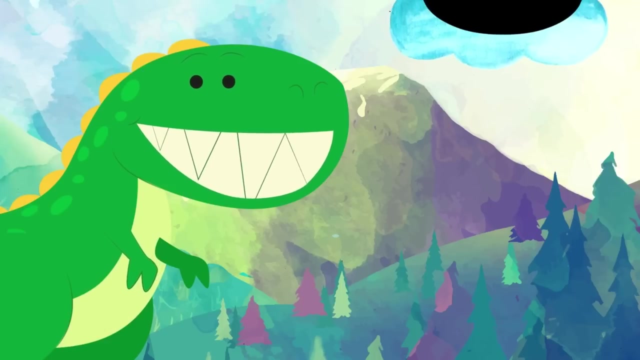 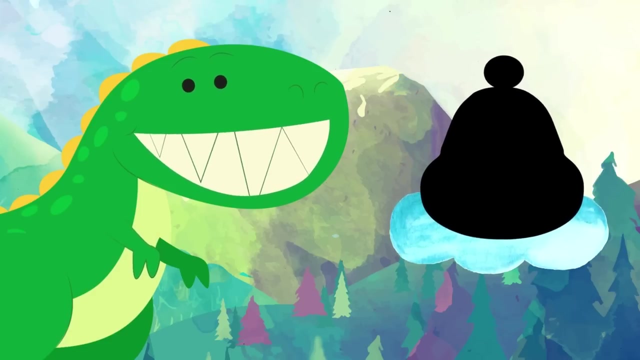 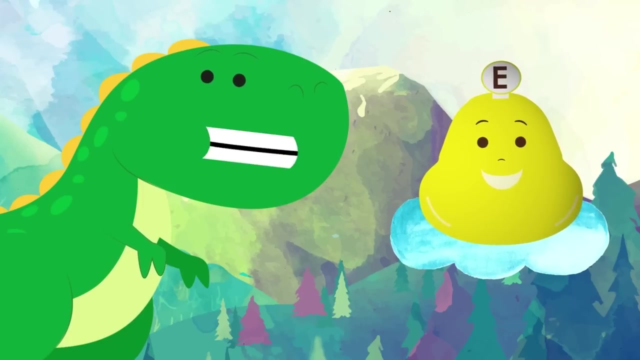 Which one is it? And the note is: That's right, it's C. Here comes another one. This one's a tough one. This one's a tough one. Do you have an answer? And the note is: That's right, it's E. 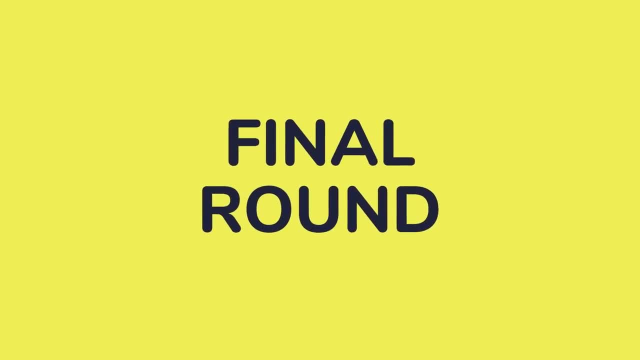 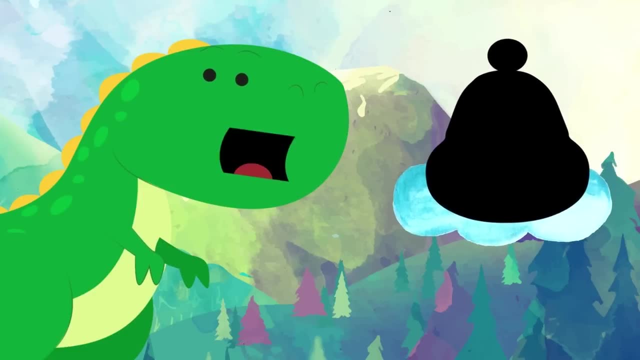 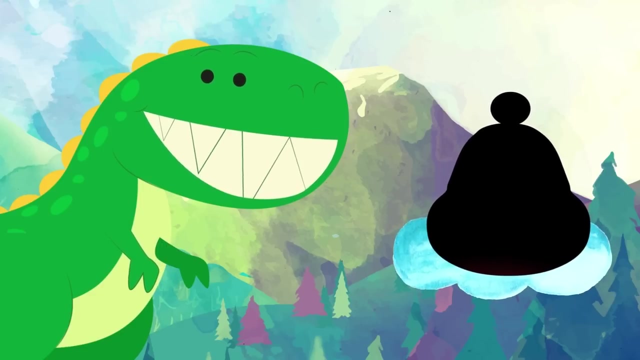 Now it's time for the final round. Let's see what it is. Let's see what it is, And the note is. This one's a tough one. Which one is it? And the note is Good, guess It's C. 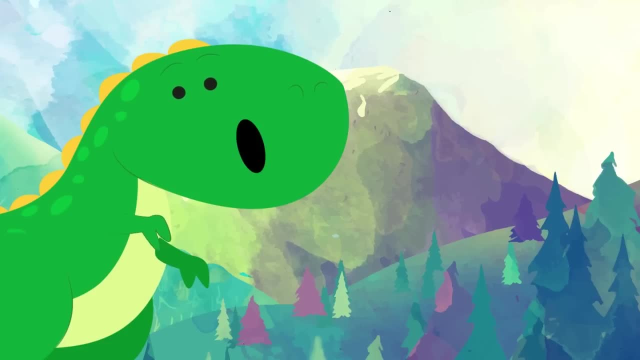 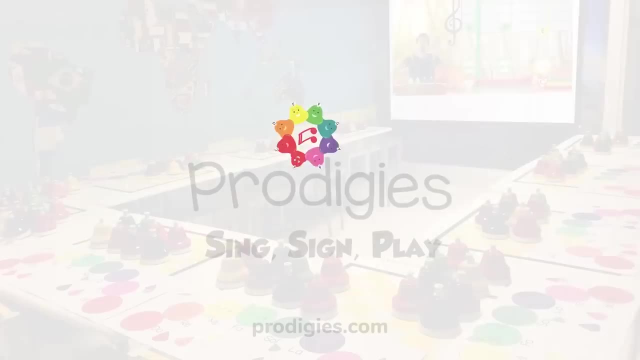 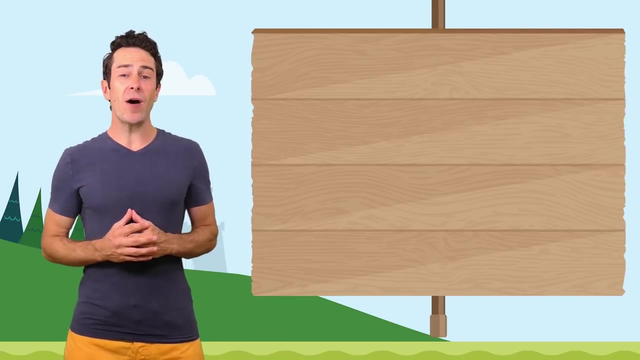 Well, thanks for playing everybody. We had a lot of fun and we'll see you here next time. on What Note Is It Nice job with that listening game. everyone To finish up strong. we're going to sing sweet beats one more time. 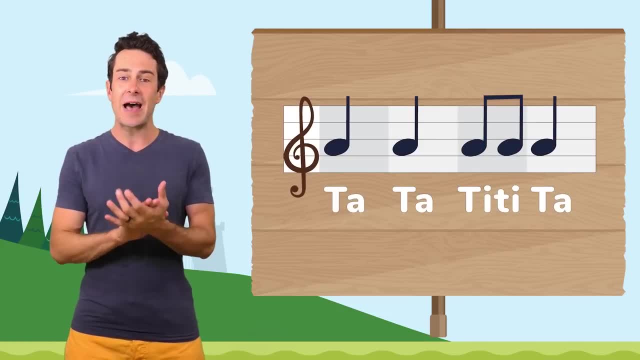 but this time we're going to add some harder syllables like ta-ta-ti-ti-ta. Can you sing that Ready set go Ta-ta-ti-ti-ta, Again ta-ta-ti-ti-ta. 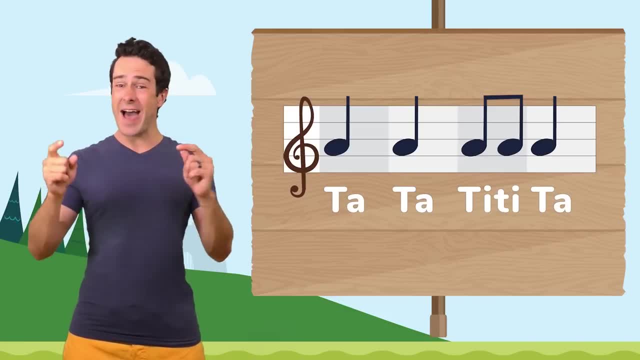 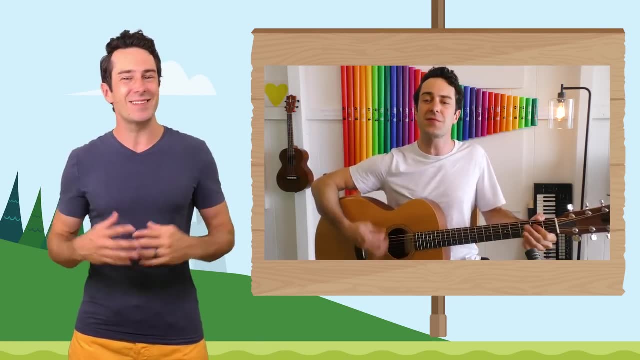 Ta-ta-ti-ti-ta, Ta-ta, Ti-ti-ta. And we're going to head back to the studio one more time to have some fun singing sweet beats together. If you want some sweet beats, we've got some. 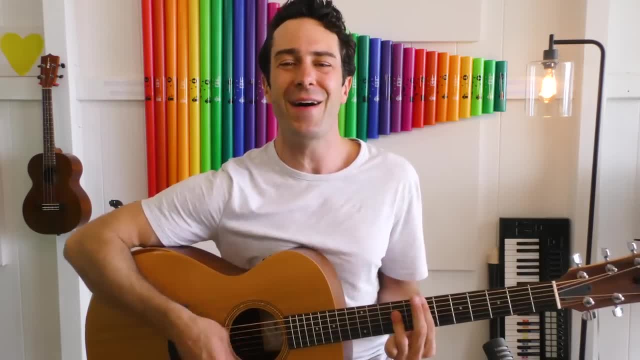 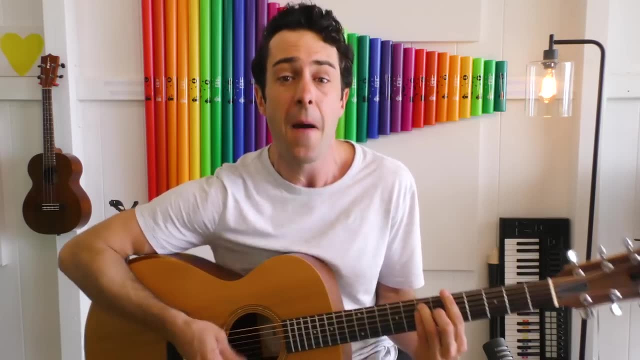 If you want some sweet beats, we've got them. If you want some sweet beats, we've got some. If you want some sweet beats, we've got them. All right, here we go, Ta-ta-ti-ti-ta. 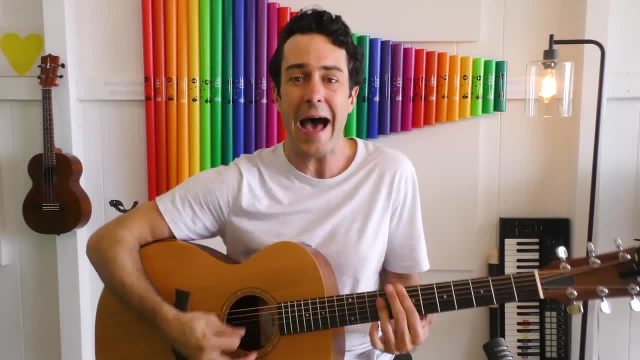 Ta-ta-ti-ti-ta, Ti-ti-ti-ti-ta-ta, Ti-ti-ti-ti-ta-ta, Ti-ti-ti-ti-ta-ta, Ti-ti-ti-ta-ta-ta. 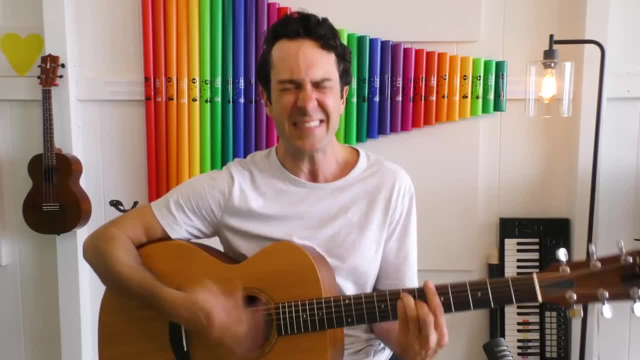 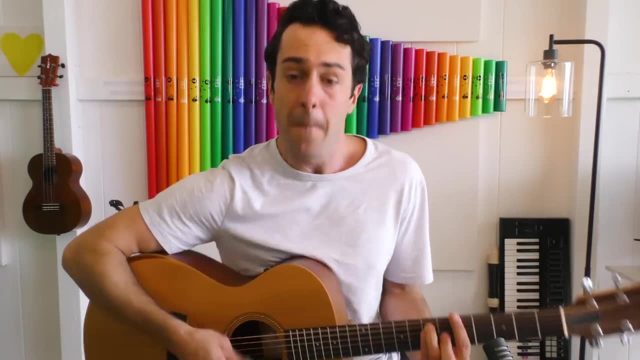 Ti-ti-ti-ti-ta-ta, Tika-tika-tika-tika-ta-ta, Tika-tika-tika-tika-ta-ta Sweet beats- oh, we've got some. And if you want some sweet beats, oh, we've got them. 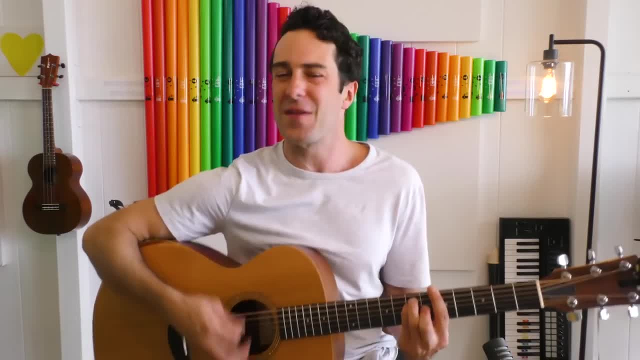 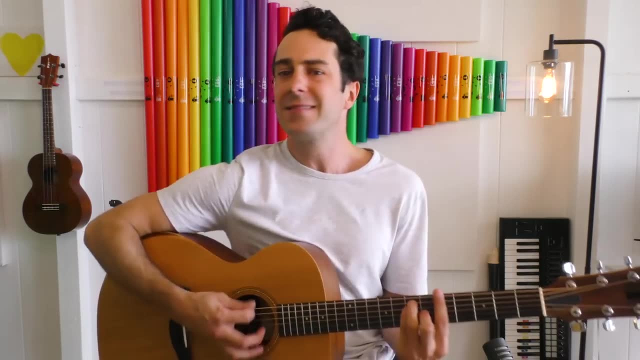 And if you want some sweet beats, oh, we've got some. And if you want some sweet beats, oh, we've got them. Let's try it again, Ready, Ta-ta-ti-ti-ta, Ta-ta-ti-ti-ta. 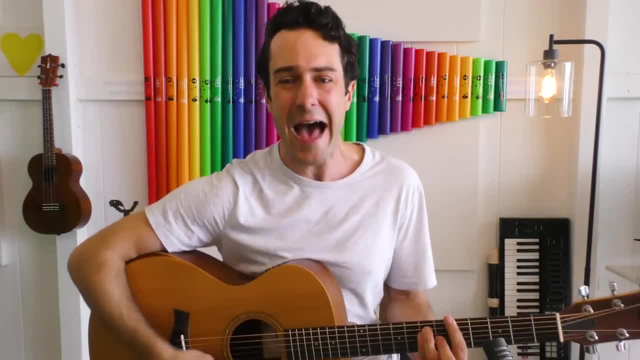 Ti-ti-ti-ti-ta-ta, Ti-ti-ti-ti-ta-ta, Ti-ti-ti-ti-ta-ta, Ti-ti-ti-ta-ti-ti-ta, Ti-ti-ti-ti-ta-ta. 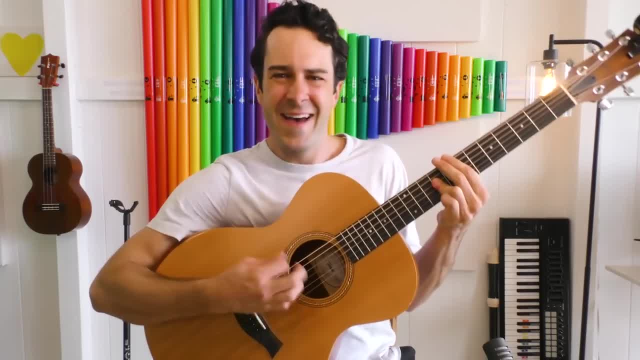 Tika-tika-tika-ta-ta Sweet beats, oh, we've got some. And if you want some sweet beats, oh, we've got them. And if you want some sweet beats, oh, we've got them. And if you want some sweet beats, oh, we've got them. 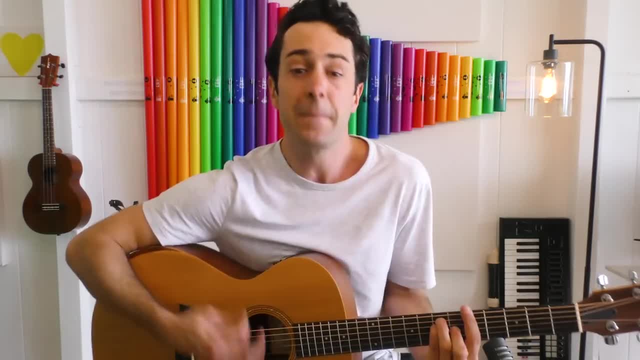 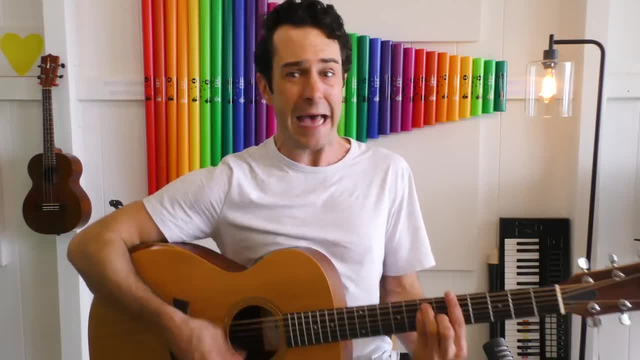 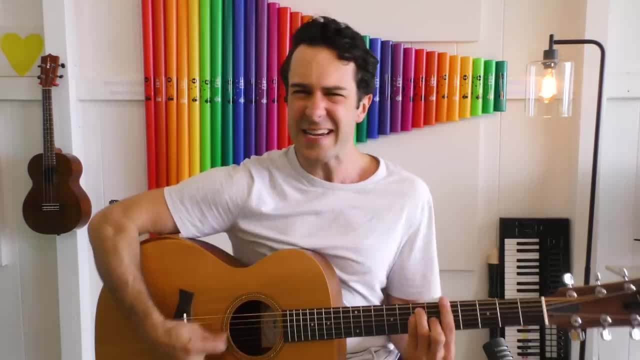 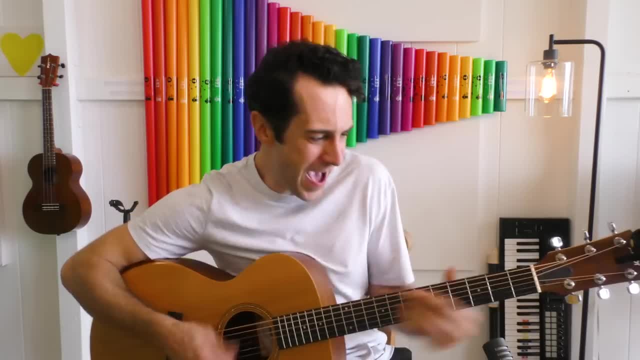 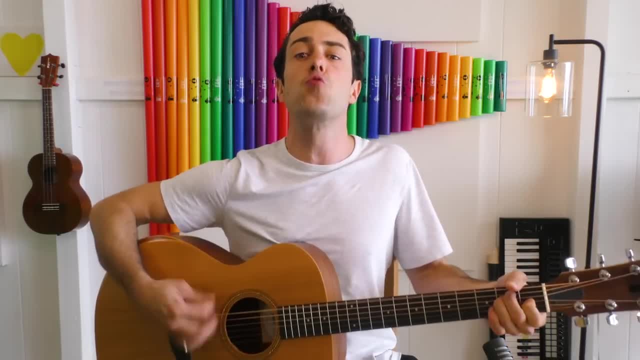 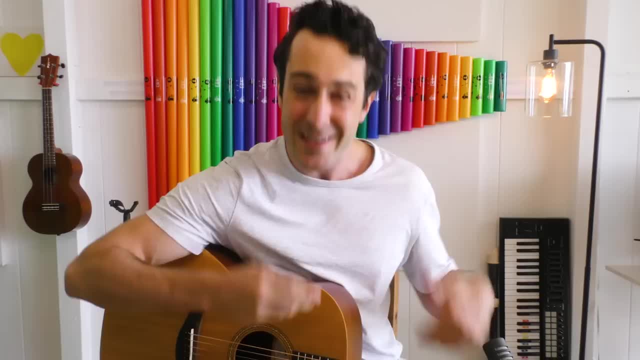 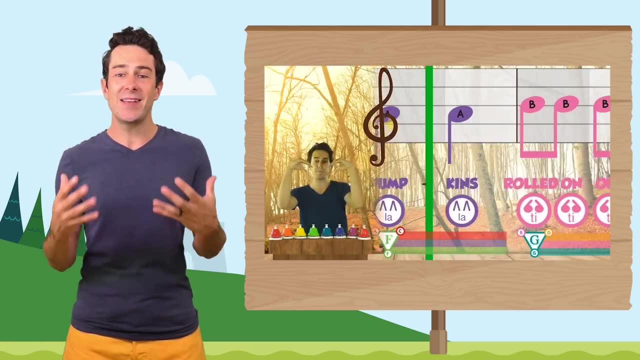 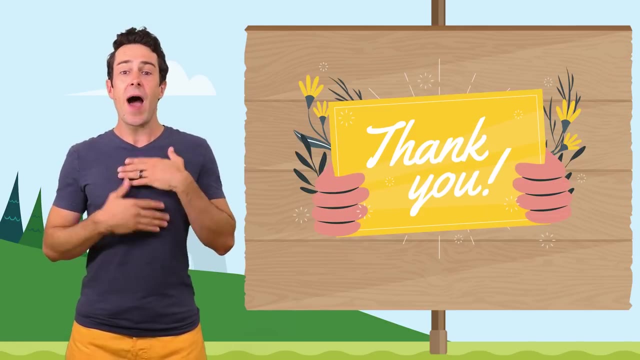 Give yourself a huge round of applause. If you had fun singing and playing with me today. we have lots more videos and lessons and activities inside of our full program at prodigiescom. Thank you so much, so much for being here. i hope you had a good time. i hope you have a wonderful rest of your day. 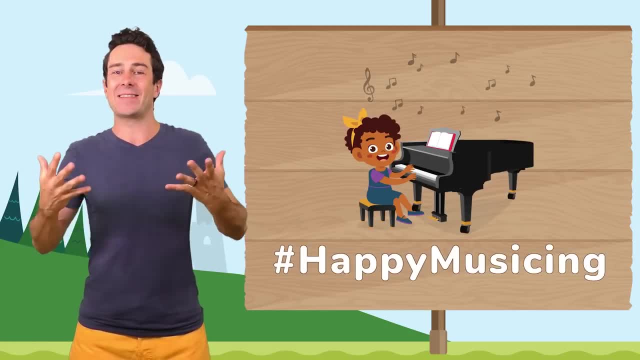 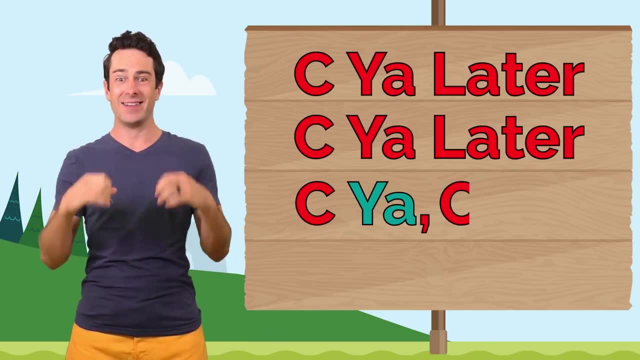 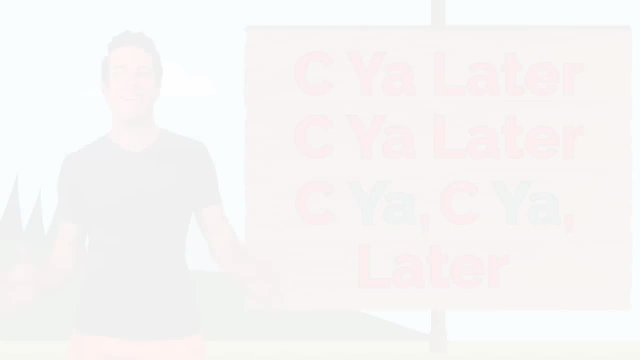 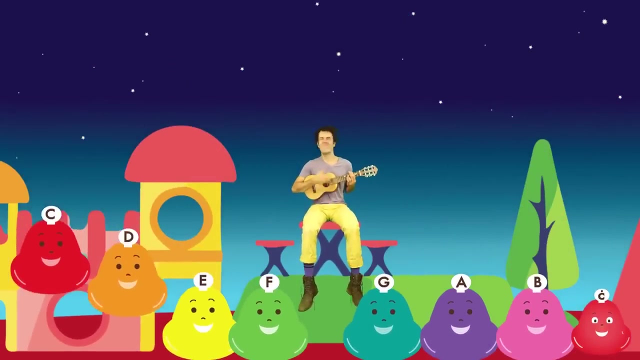 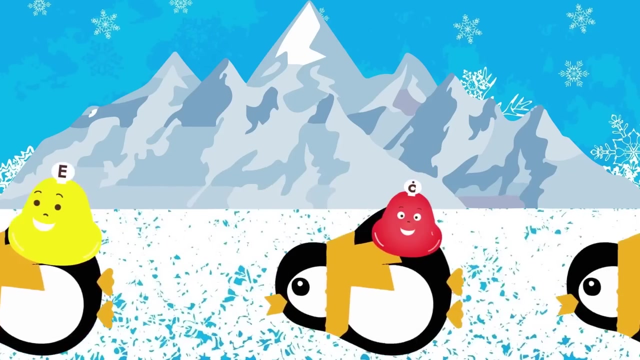 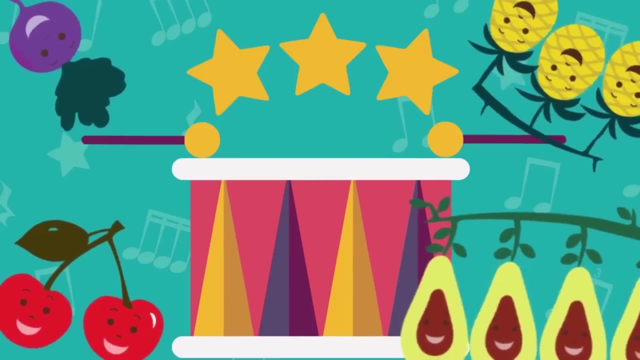 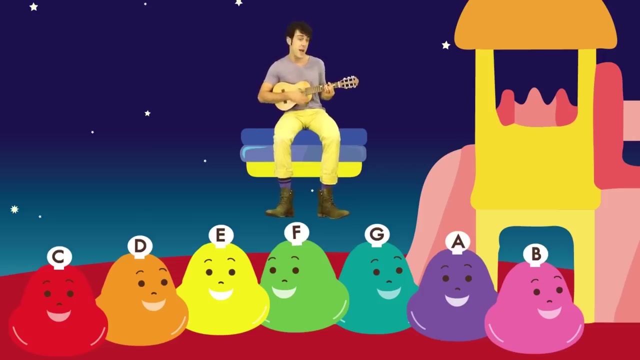 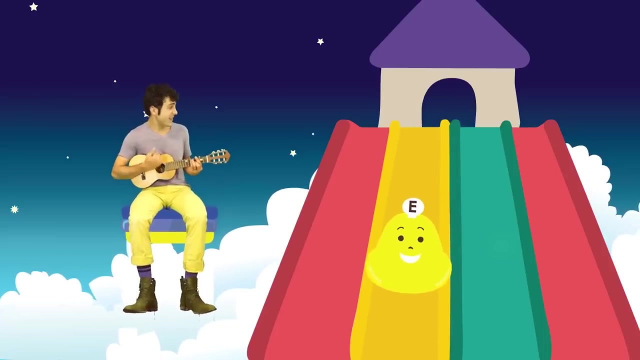 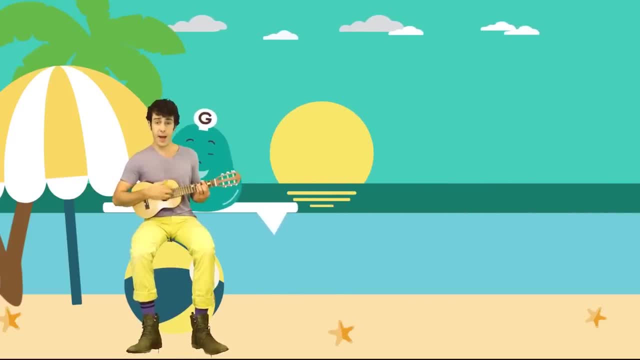 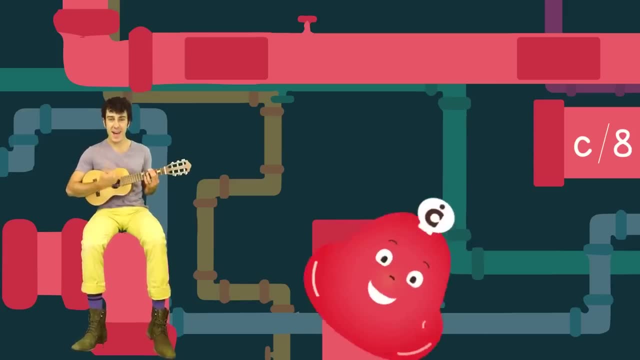 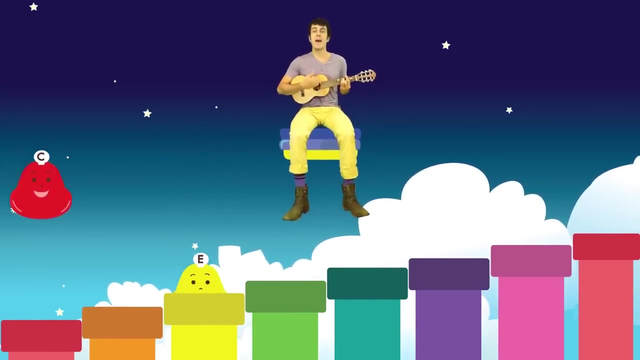 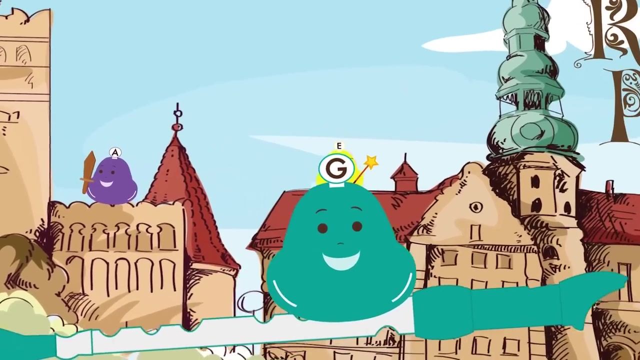 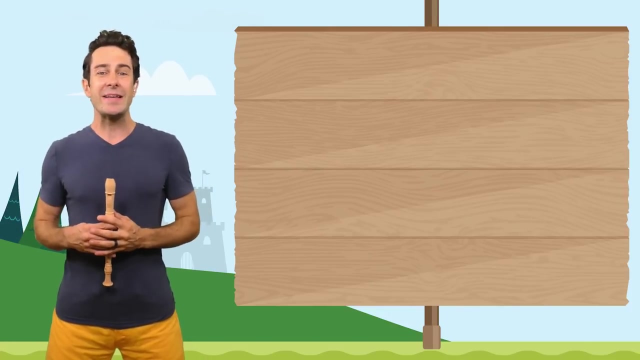 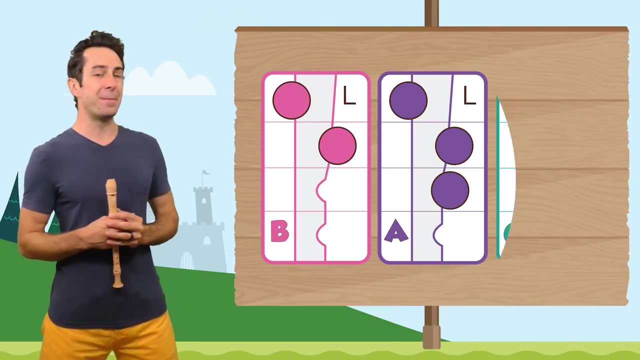 hello g, hello a, hello b, hello c. let us play, sing and play ready. do re mi fa sol, la ti do sol, do do. hey, everyone, and welcome to another song here inside of recorder prodigies. today we're going to play a beautiful tune called gently sleep, using the nodes b, a and g. 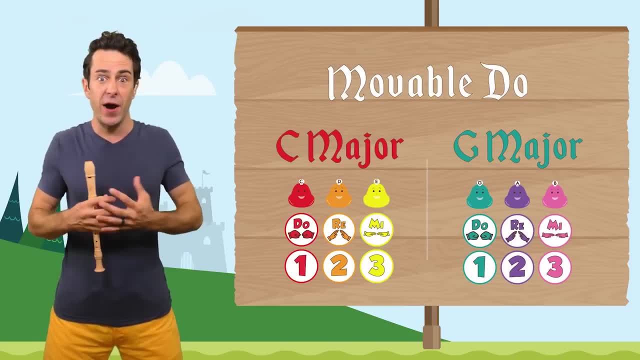 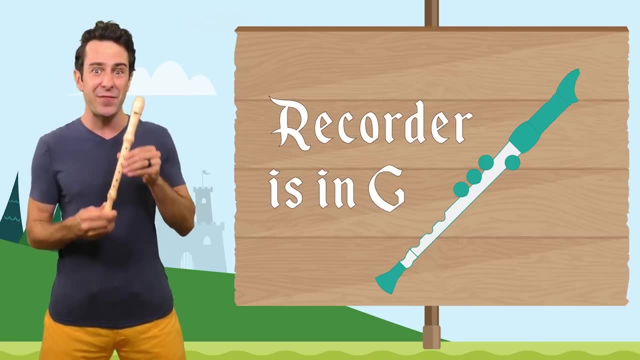 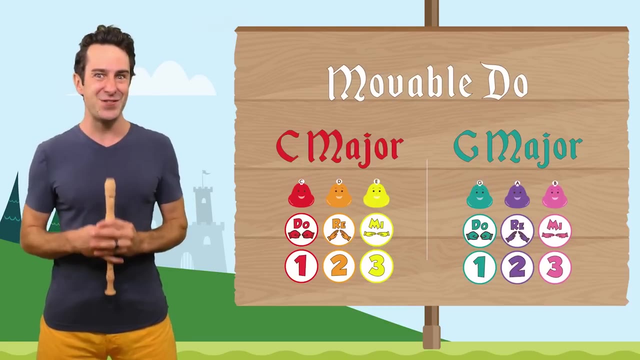 we're going to think in movable dough today, so do is going to be our home base. node g: the recorder is really easy to play in the key of g. so, unlike the bell, instead of playing lots of songs in c major, we're going to play lots of songs in g major. 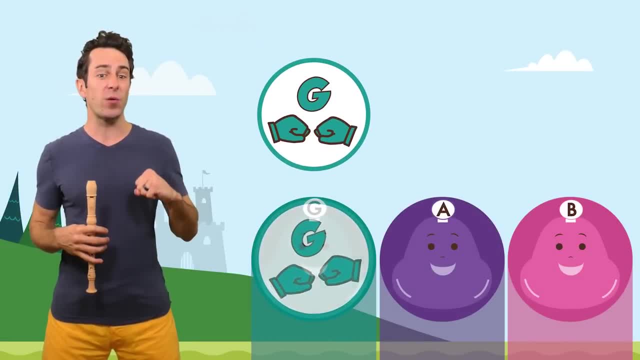 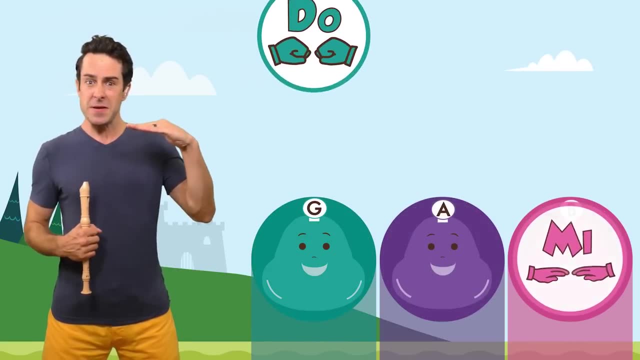 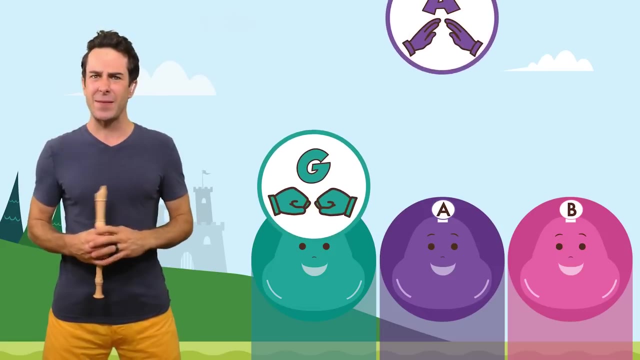 this means that our home base note today is going to be g, so we're going to call g do. all right, we'll sing, do re mi. you sing, do re mi. yeah, those are the three notes that we're going to be singing, and we're singing them on a, g, an, a and a- b. make sure you can play a, g, a and b on your recorder and. 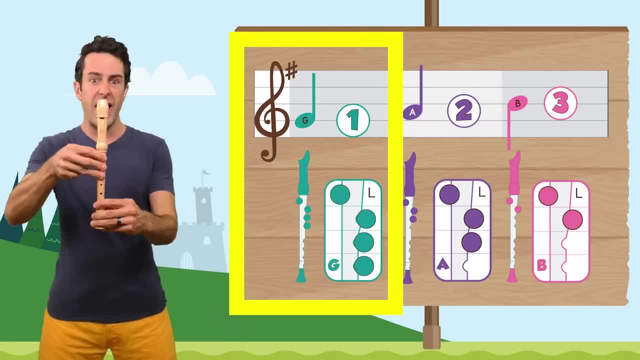 so, for example, if we're on a back note, we can sing it e, f and m? e, but if we're on a cر measure, we're going to get in the middle of that. but the g note comes from a c. who's mid note? uh? 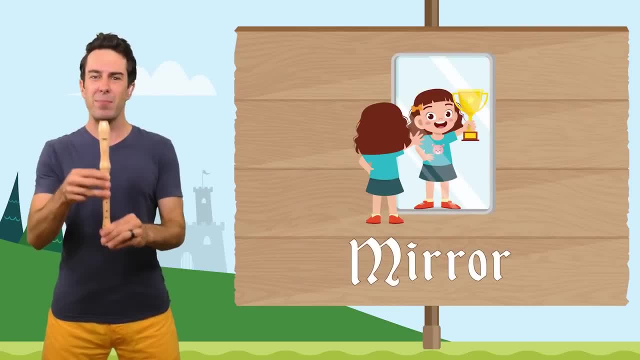 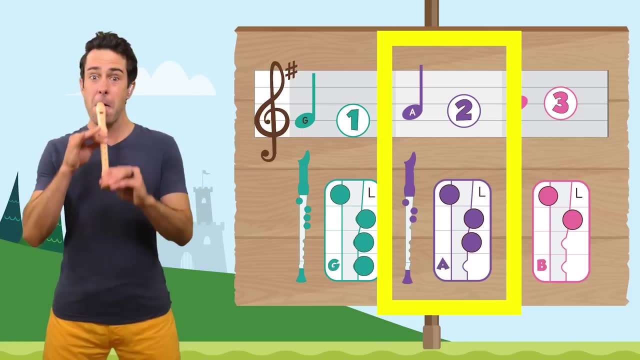 c and d, d flat. so we play a little bit of that and song a such a finger, finger, finger, finger, finger, and there you go. so that's the every note that we we we're going to be playing, along with a little bit of the three notes that we're going to be using. 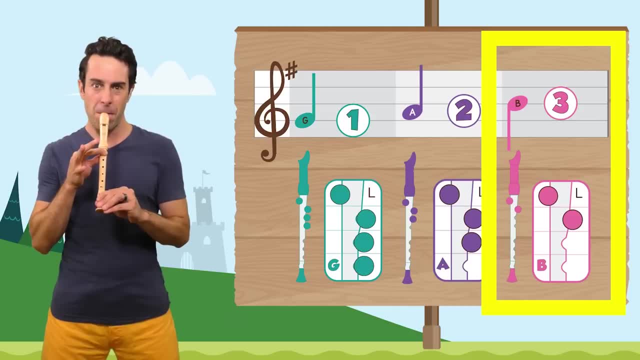 together is a swallow. I know a lot of you guys don't have a small g數, but some fans of ours, especially from online music, feel free to tap down below if you're interested in that type of a note notes you're gonna need for today's song. 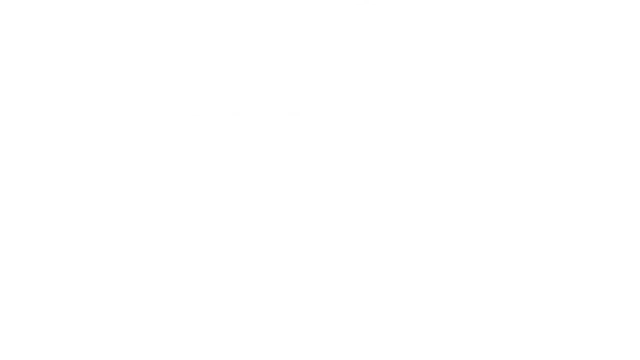 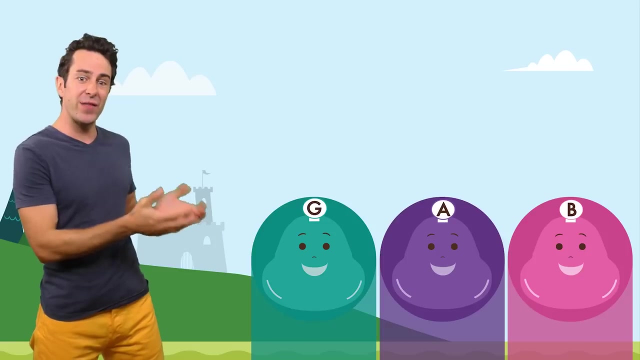 Thanks so much for being here and let's hop into Gently Sleep. All right, we're ready to play Gently Sleep. We're gonna start out with the solfege hand signs as they fall into the circles and then we'll play our recorder one time to finish up. 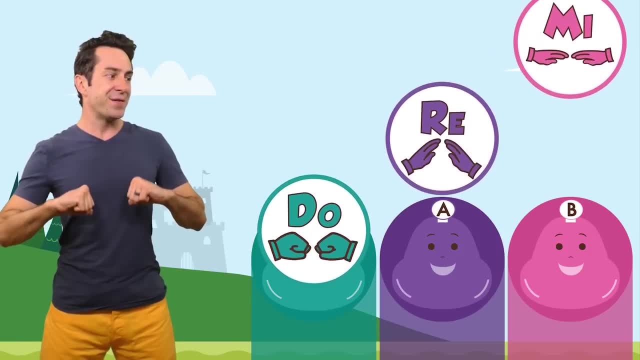 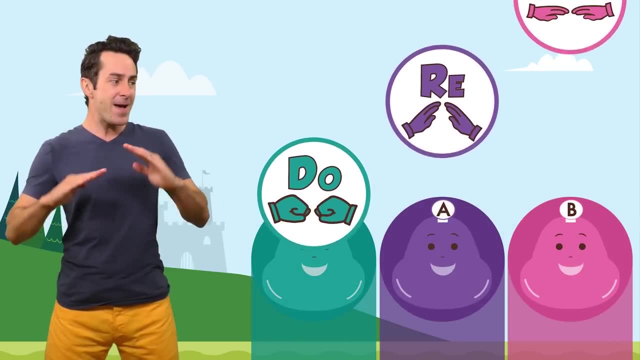 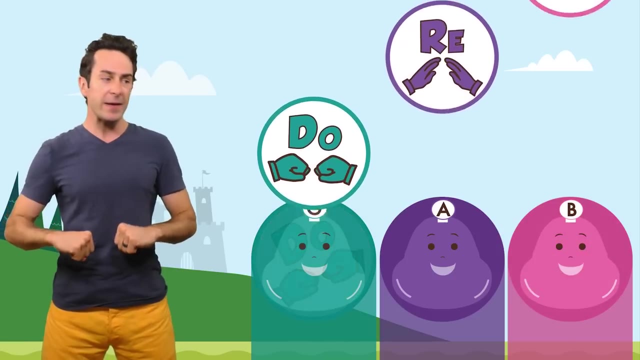 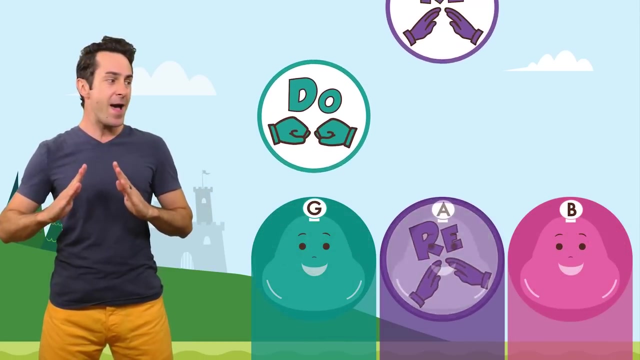 Starting on: do Ready set. Do re mi re, do re, do re mi re mi. do again. Do re mi re, do re, do re mi. 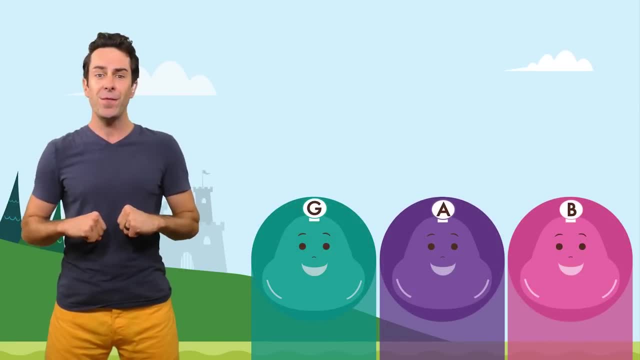 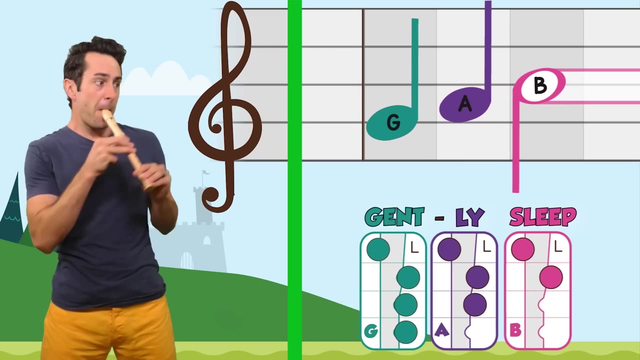 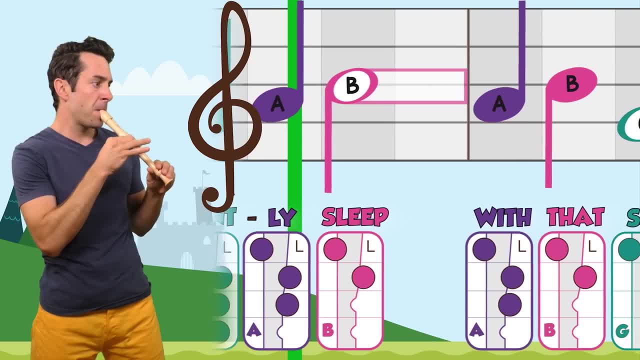 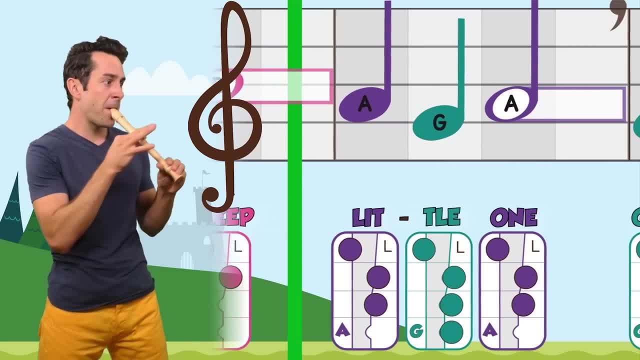 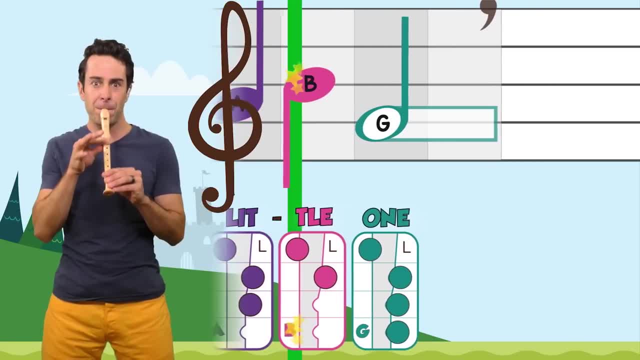 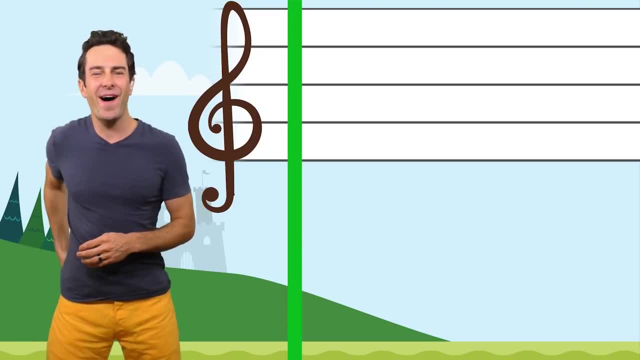 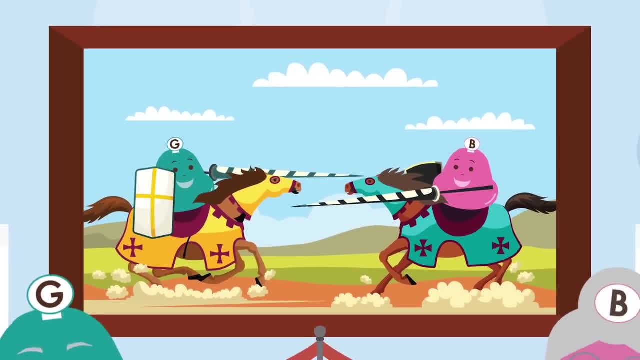 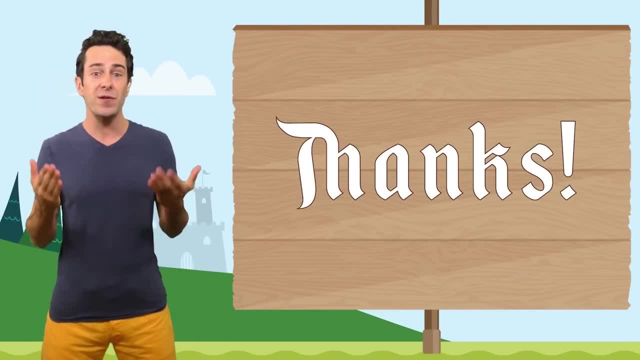 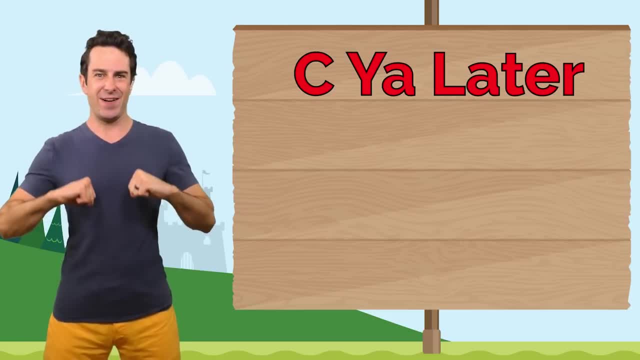 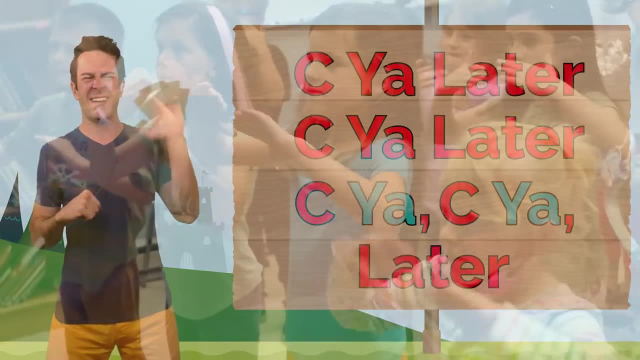 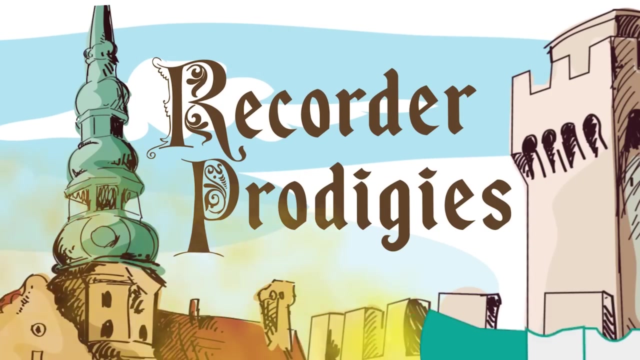 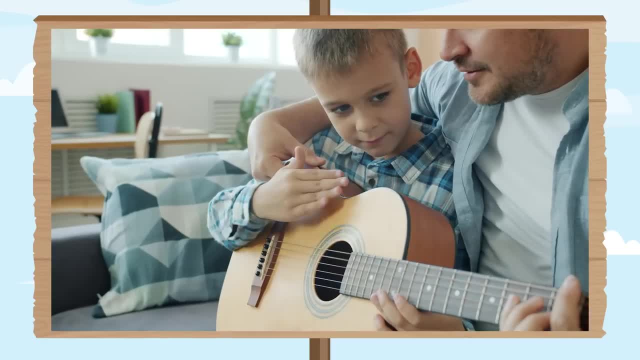 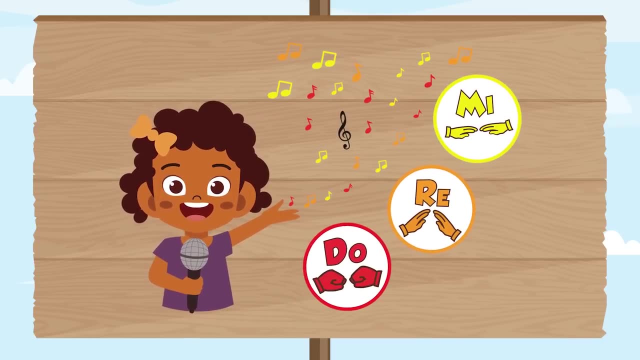 It's great for your brain and for your heart And it's a lifelong skill that's beloved by people all across the world. When you're learning to sing, using those hand signs can be really powerful for helping you to sing in tune and memorize the sound of the notes. 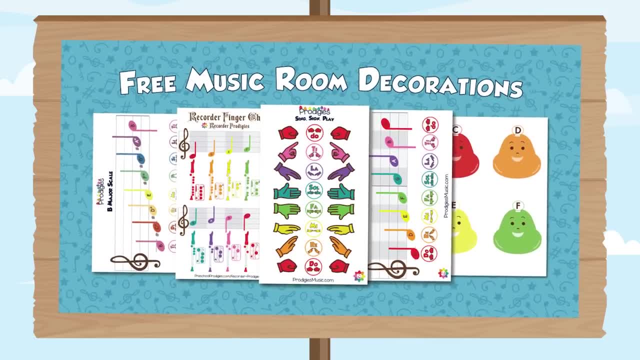 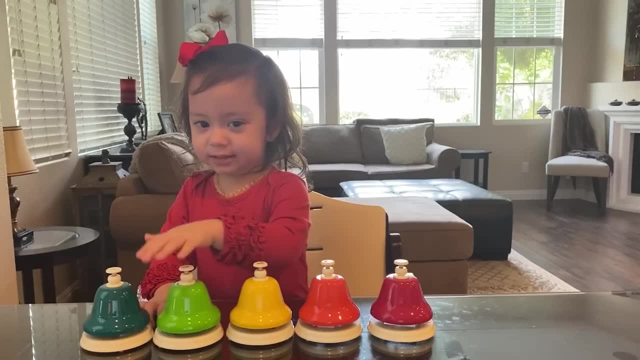 If you'd like, you can download a free poster pack of hand signs and other solfege materials at prodigiescom slash free. If you're ready to play an instrument. the easiest place to start is on the C major desk bells. 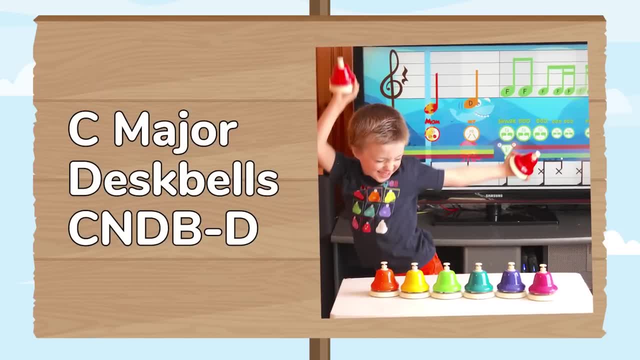 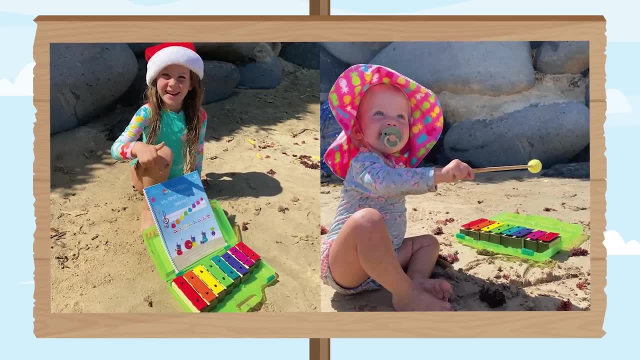 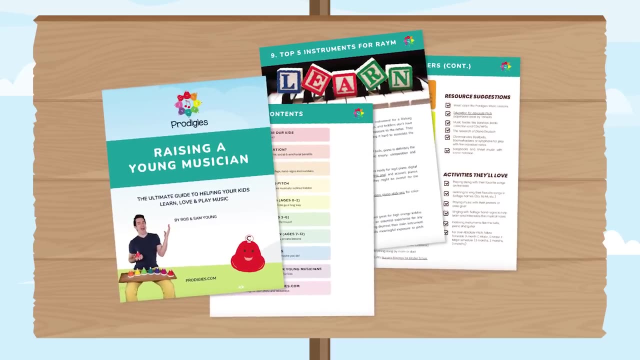 You can find them by searching for CNDB-D online, Or you can download our free instrument app, Prodigy. Otherwise, pianos and xylophones are also excellent places to start. Finally, I've got one more awesome free download to help you on your musical journey.